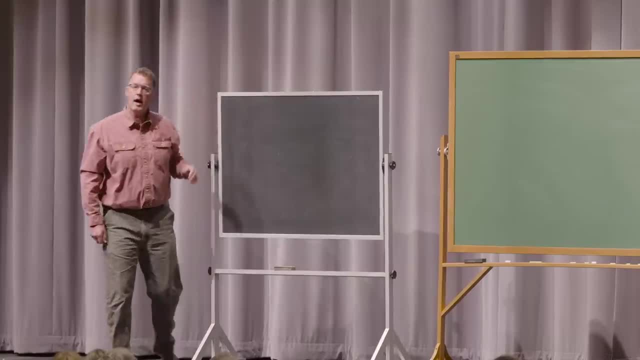 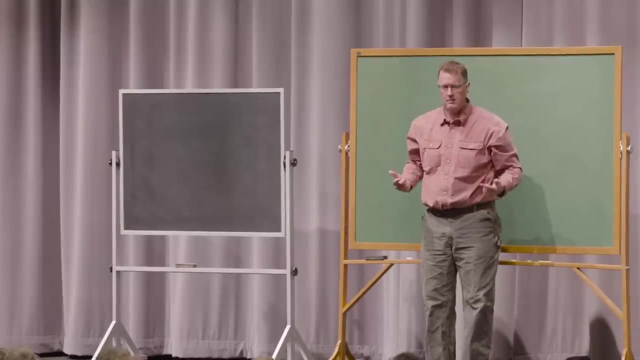 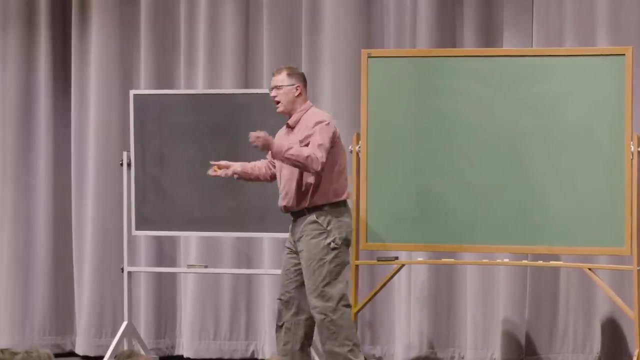 Let's pretend that it's a world map, a world map from your youth, in front of your grade school classroom. Can you picture a world map in your mind? How many continents are on that world map? Seven continents, that's right, And there's a handful of oceans between North America and. 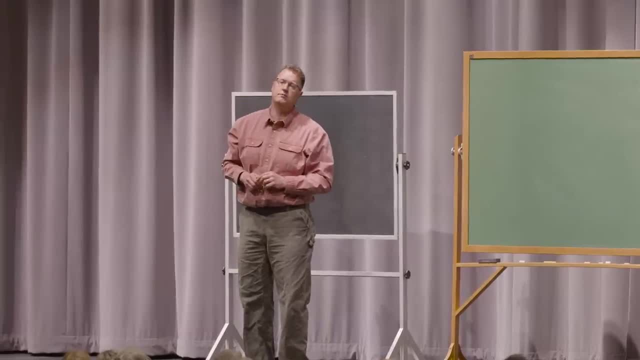 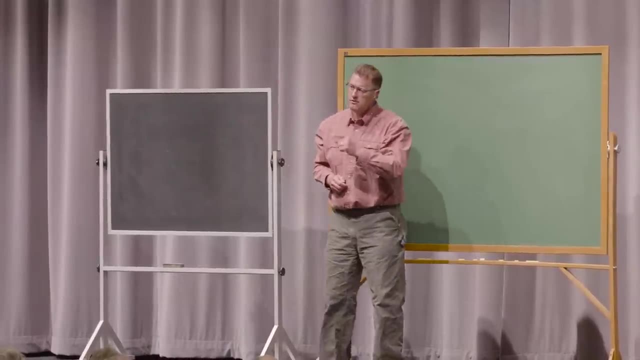 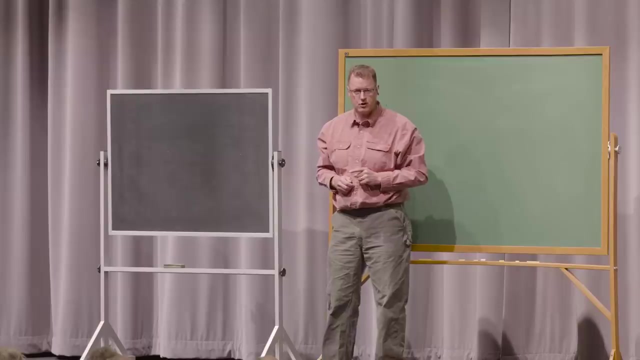 Africa, the Atlantic Ocean, the Pacific Ocean. Okay, fine, Good Aware that if we pull down a different world map for 200 million years ago, it will look very different. In fact, there'll be one continent on that world map for 200 million years ago and one 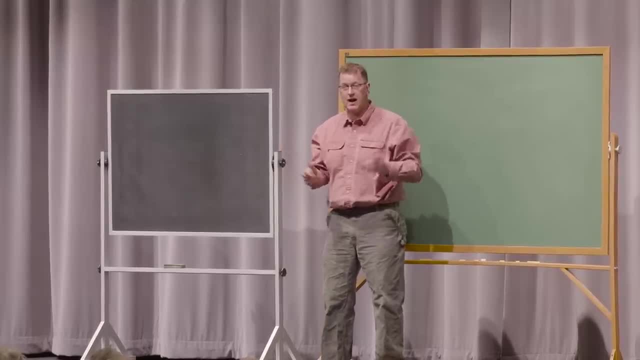 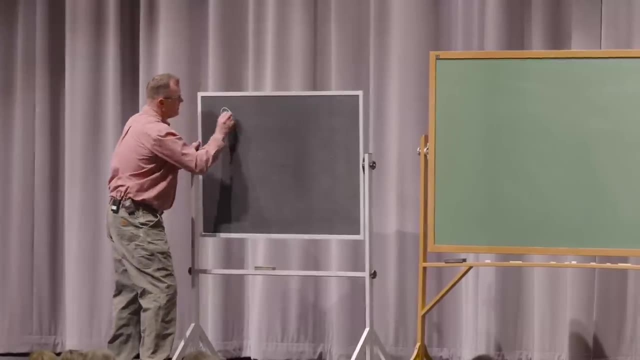 ocean And that one continent was a big, big continent. In fact, it was a super continent called Pangea. Let's write it out: Pangea P-A-N-G-E-A. That's one way to spell it, and 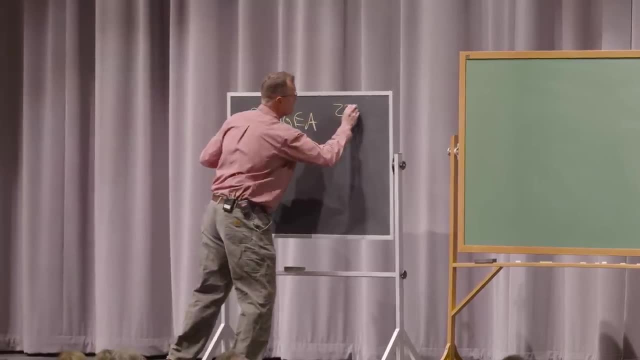 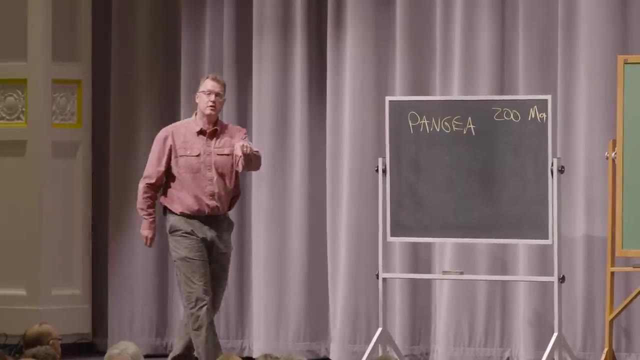 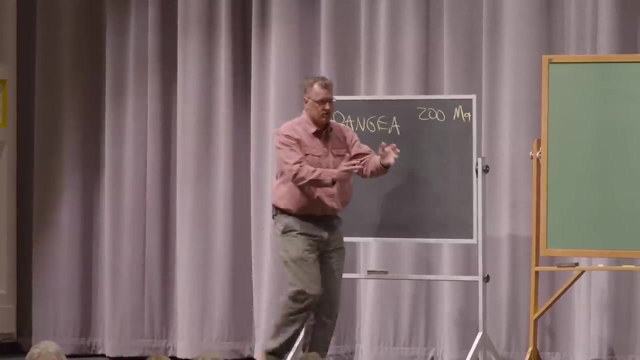 that's how we're going to spell it tonight. Hundred million years. Again, we're going to be working in. hundreds of millions of years, even thousands of millions of years tonight, more than a billion years. So one way to view Pangea is okay. it was a super continent and in the last 200 million years, 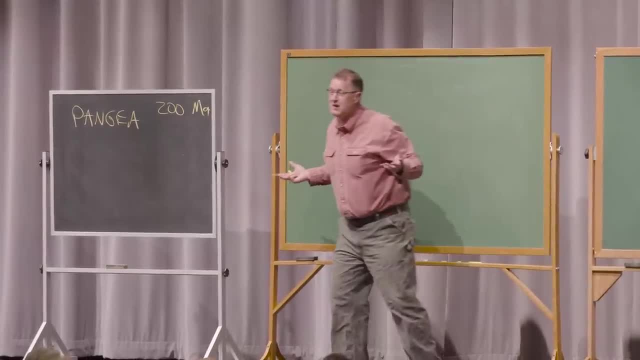 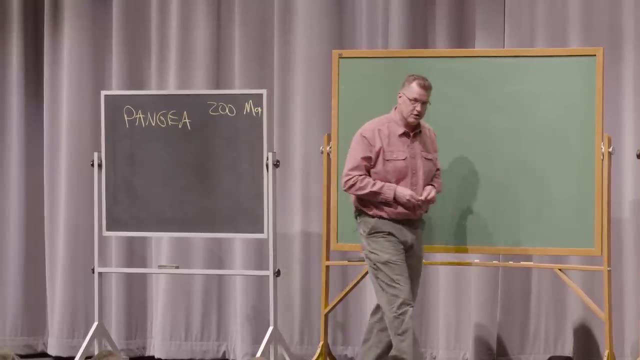 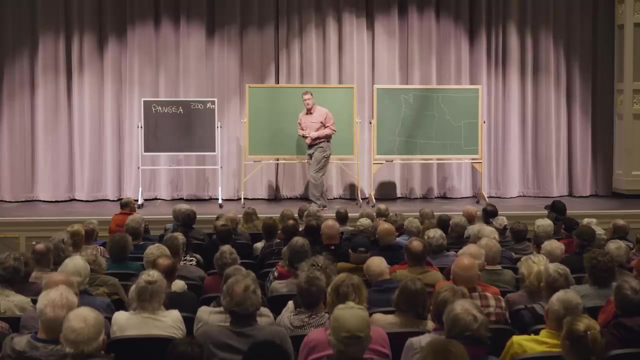 Pangea has been breaking up. It broke into seven pieces, our seven continents, and those continents continue to drift away from each other. There was no Atlantic Ocean. during Pangea, You could walk directly from New York to Morocco in Africa And, in the last 200 million years, the Atlantic. Ocean has continued to grow in width and the Pacific Ocean has been shrinking in width Four inches a year. The Atlantic Ocean grows four inches wider every year. That's pretty fast. We have GPS measurements to document that Christopher Columbus did not have as far to travel. 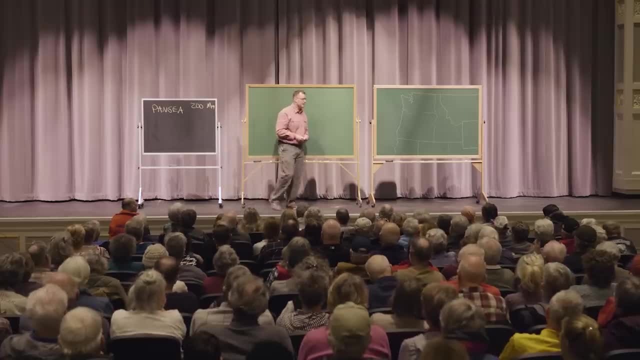 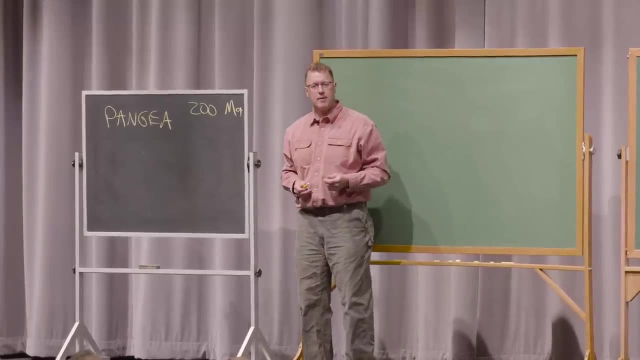 as we do now, Insert laugh track: Okay, great. So if we open Pangea, if we open the Atlantic Ocean as we break up Pangea, we're actually closing the Pacific, And so one way to view Pangea breaking up is we're. 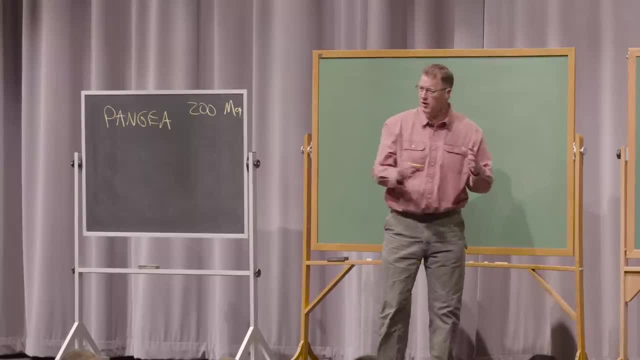 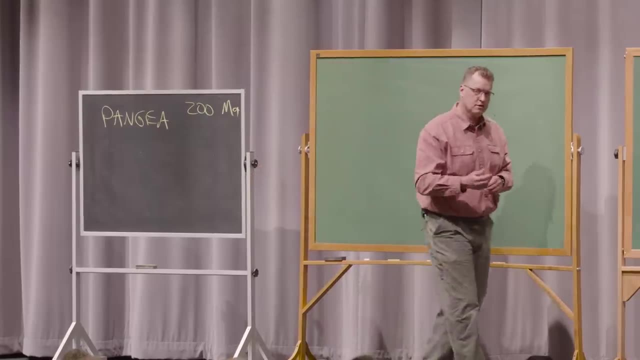 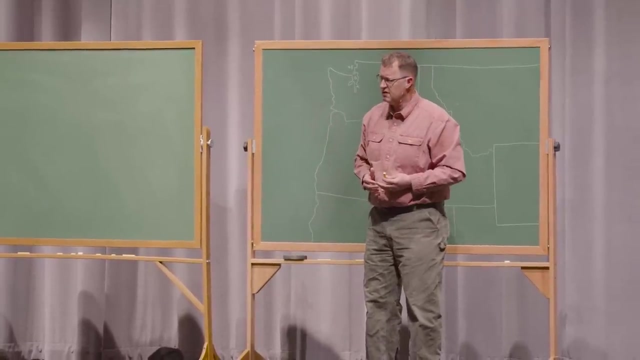 heading for the next super continent. We're closing the Pacific and opening the Atlantic. Now, if you're aware of Pangea- and I think most of you are- maybe you assume that Pangea was the way Earth was given to us. Like Pangea was the original configuration And there's 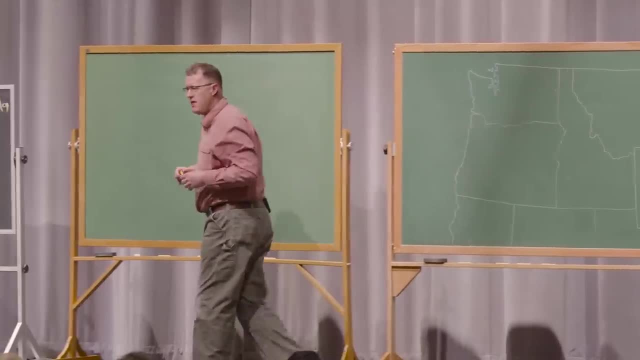 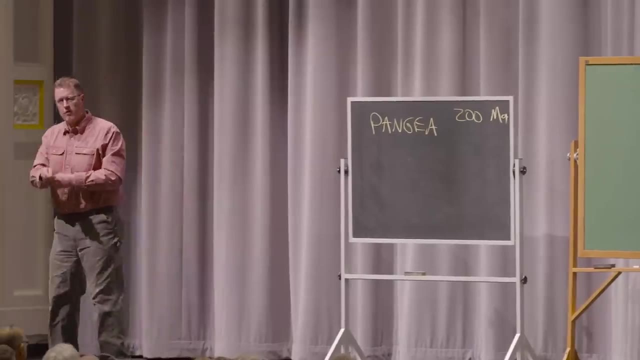 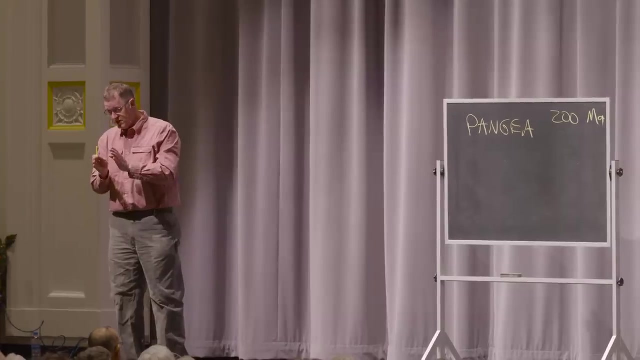 just simply been this breakup. I think a lot of people think that without thinking about it a whole lot. But how old is the Earth? This is a science lecture, right? How old is the Earth? It's 4,600 million years old. The Earth is 4.6 billion And I want to stay in millions tonight. 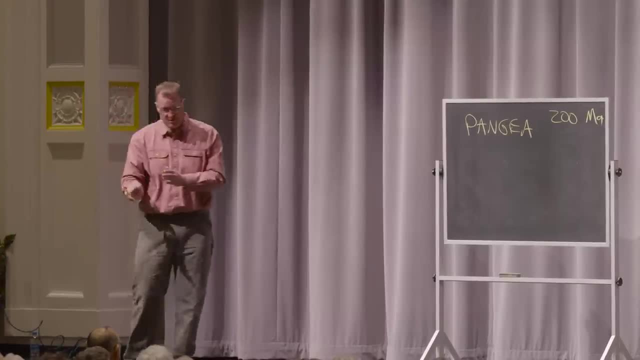 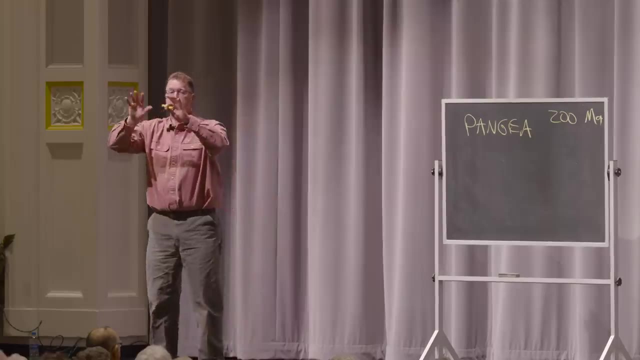 I don't want to go back and forth between millions and billions. okay, So 4,600 million. So there's a lot. There's a lot of time before Pangea. That's the next concept. There was a completely different. 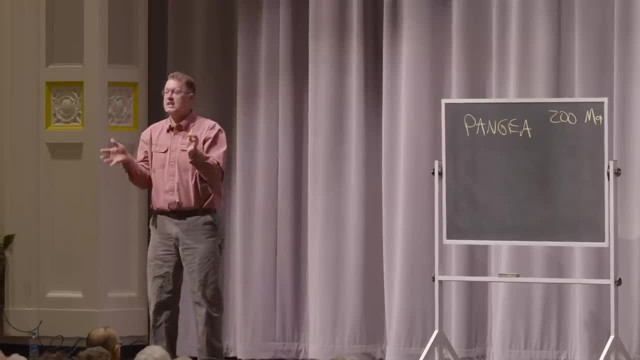 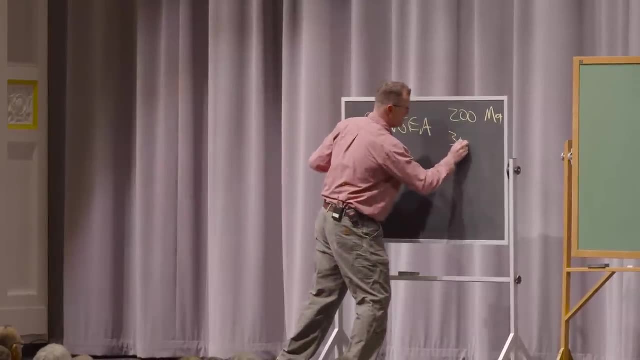 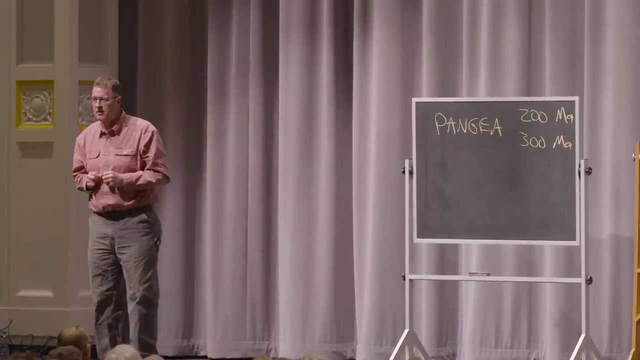 global geography that's almost unrecognizable to us before Pangea. Therefore, there was a time that we assembled Pangea- Yes, like a jigsaw puzzle. That's the common analogy. Put the pieces of the puzzle together, So Pangea super continent was together for 100 million years. That's a lot of time, But that's worth thinking about for a second. That's a long time. Dinosaurs were alive during when Pangea was together, And dinosaurs were alive when Pangea started to break apart. A hundred million years for one continent and one ocean on planet Earth. 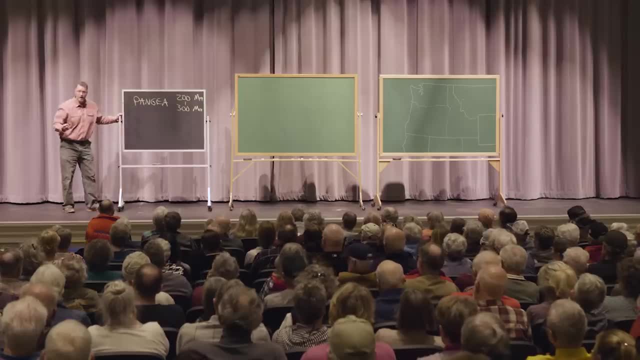 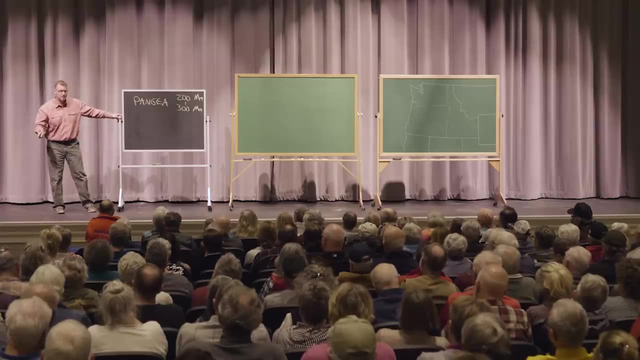 But I got room And I got a piece of chalk And I'm going to write down two other names of two other names, And I'm going to write down two other names of two other names, And I'm going to write down two other super continents that we now know about, that predate. 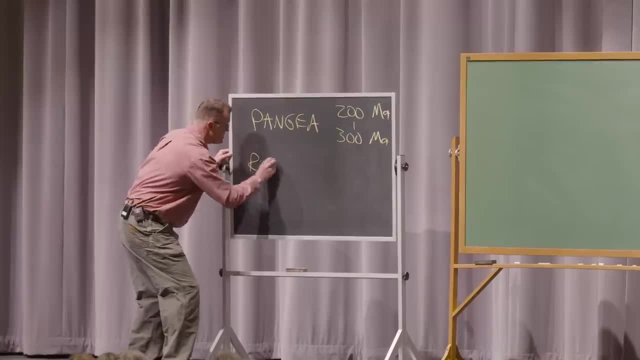 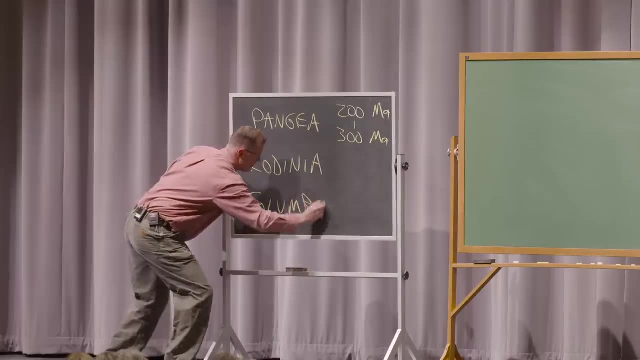 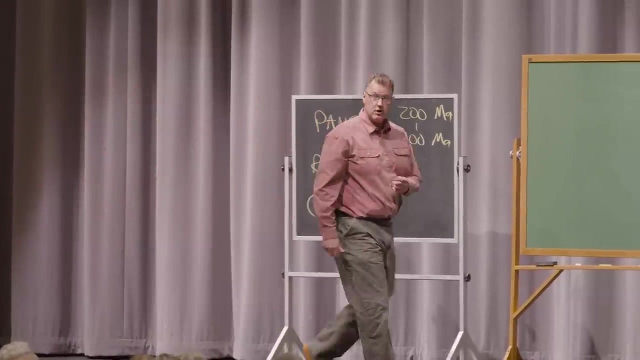 Pangea, Let's get to it. Rodinia, Columbia, And you're like: wait a minute, I like geology. I read about geology all the time. I've never heard about either of those. Well, they're pretty new. The proposal for the super continent. 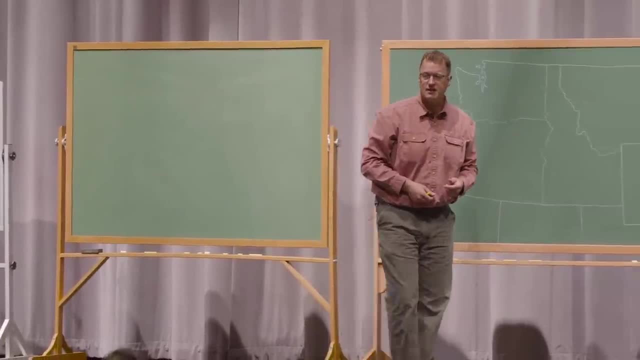 Rodinia got into scientific research And I'm going to write down two other names. And I'm going to write down two other names And I'm going to write down two other names And I'm going to papers. in the early 1990s, That's not that long ago, Pangea was proposed by Alfred Wegener. more. than a hundred years ago, And the super continent of Columbia, sometimes called Nunia, came out in the last 15 years. So this is pretty new information, So don't feel too bad if you haven't heard about it. I knew very little about these two super continents. about a week ago I've been 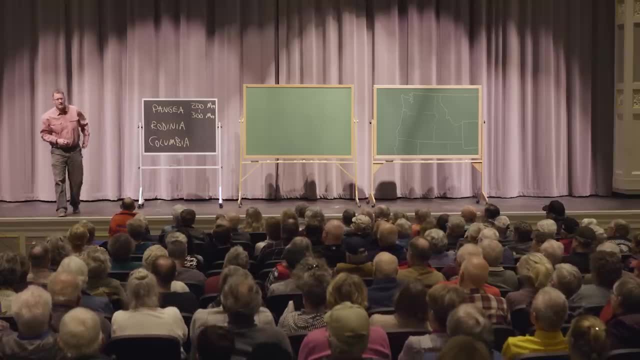 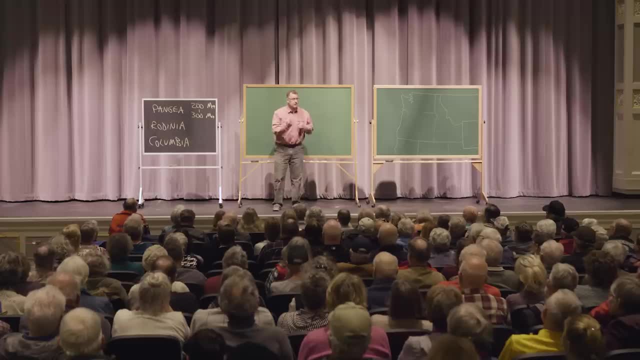 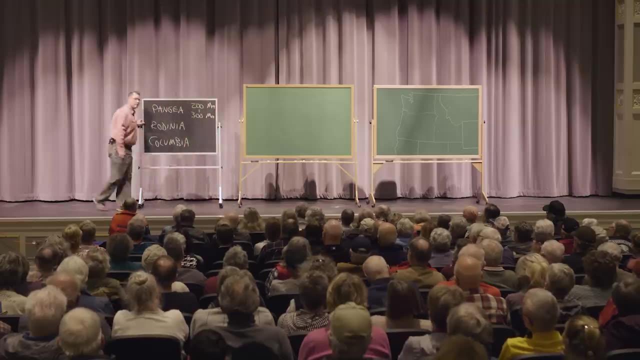 I'm like, oh my God, I got a lot of work to do on this lecture And I started emailing these authors, these researchers, in addition to reading their papers, And I've got some good stuff for you. I've got some good stuff for you about Rodinia and Columbia. I can't hold it. I got to say the first. 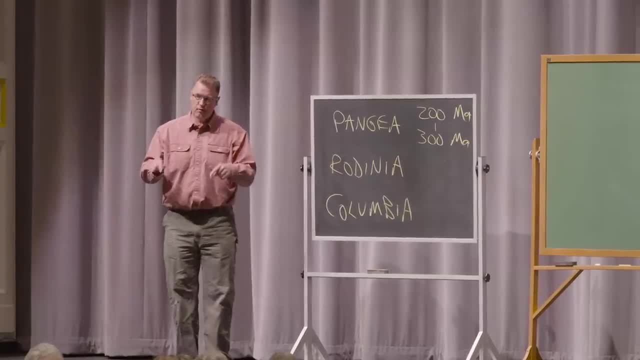 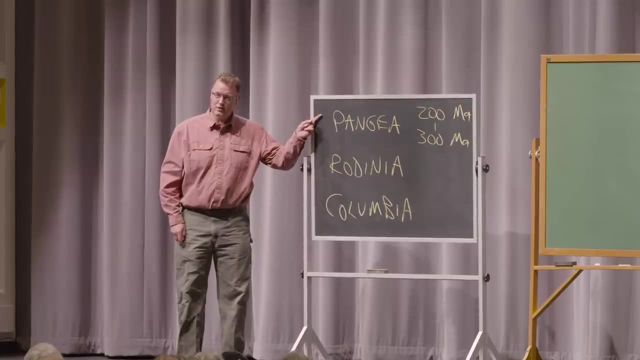 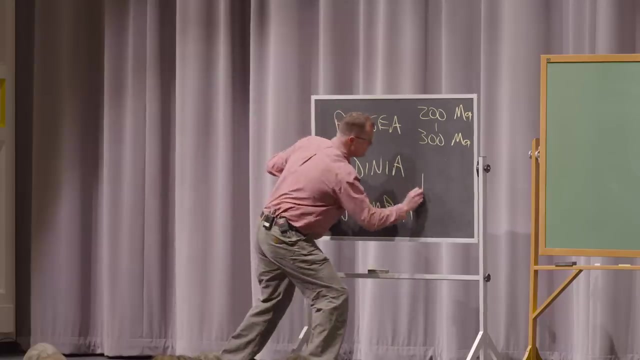 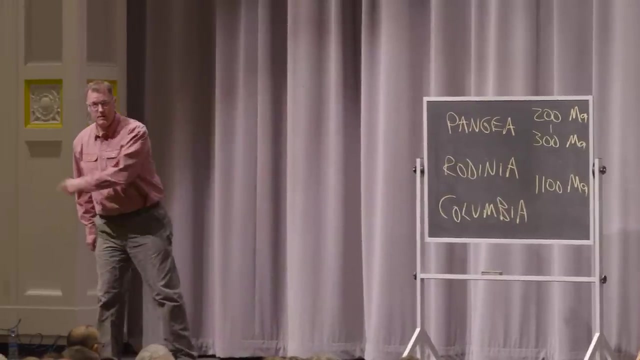 major message: The Pacific Northwest have rocks that are all about these two super continents, about Pangaea. Pangaea is too new for us, too young for us. So Rodinia was assembled more than a billion years ago. 1,100 million years ago is more than a billion right And 750 million years. 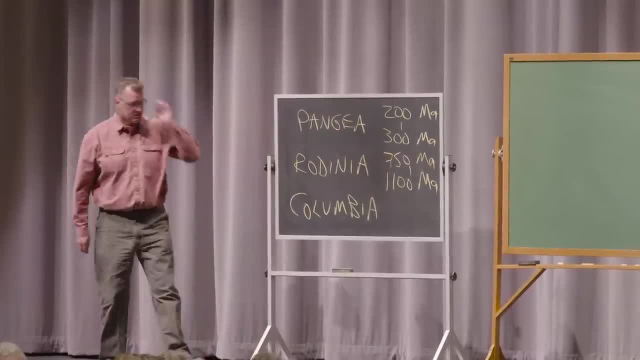 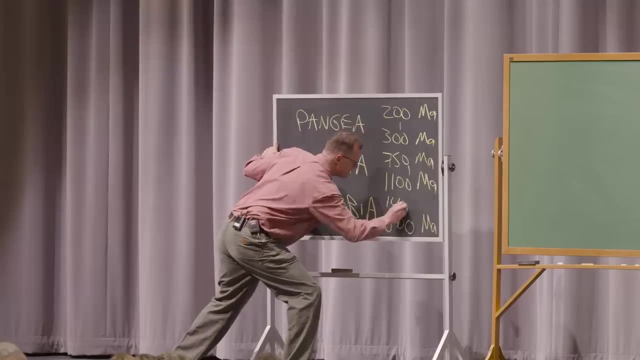 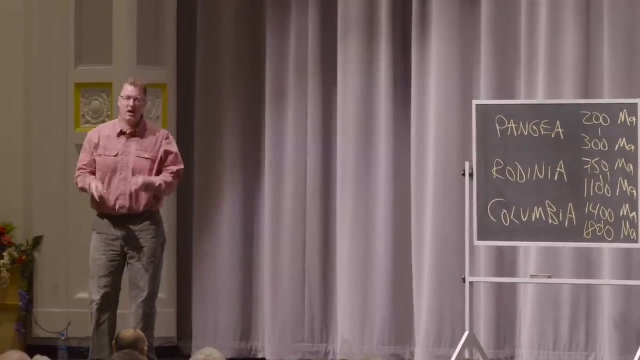 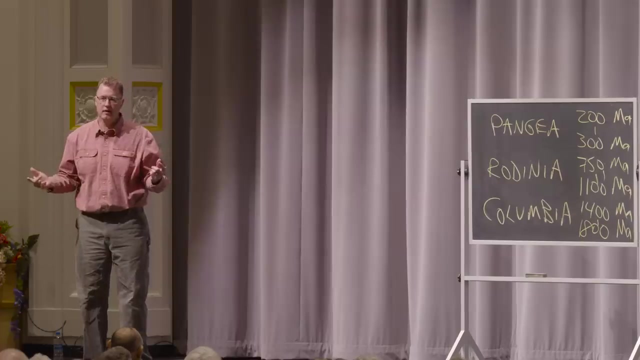 ago is when Rodinia started to break apart. Let me finish the blackboard here: Columbia to 1,400.. There's a super continent. cycle Assemble, keep together for hundreds of millions of years. break apart. We live in a ball. If we break apart a super continent, they're going to. 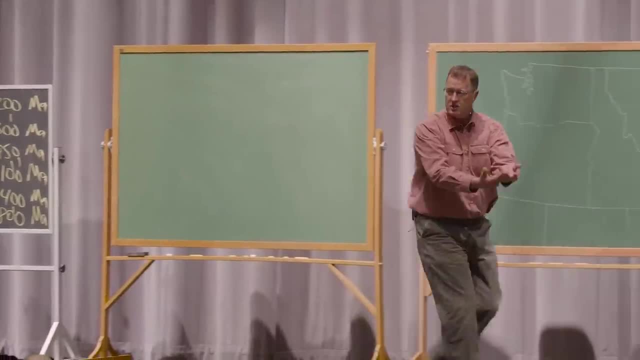 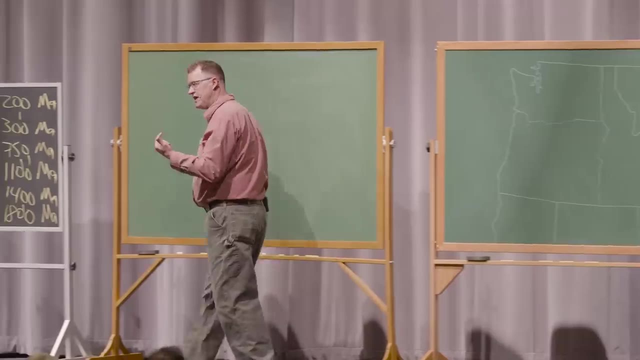 get together somewhere at some time. Next super continent, break that apart, Next super continent, you get it. And just like all kinds of history, the further back in time we go, the less we know. We know. We know by far the most about Pangaea and very little about Columbia, but enough. 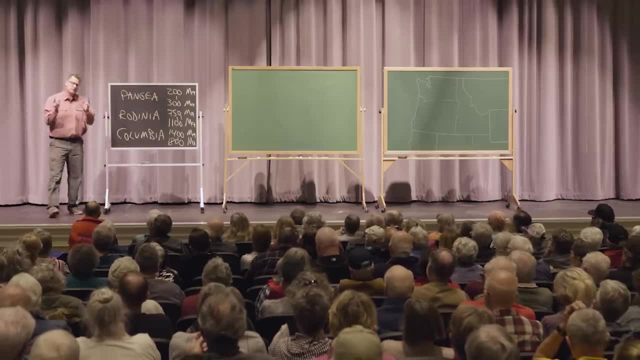 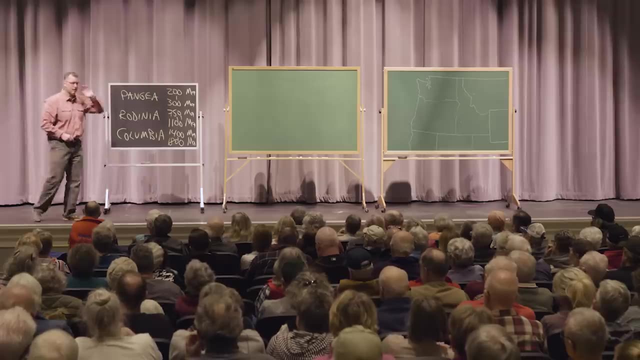 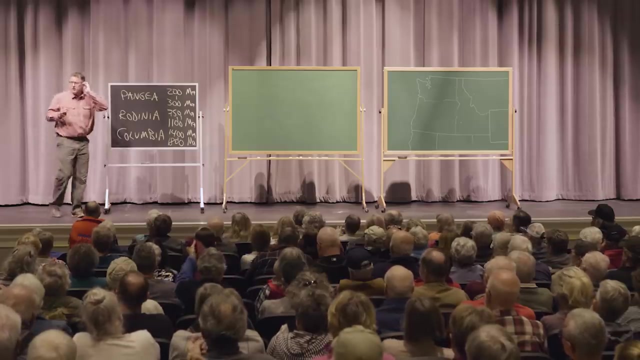 to include it in this lecture And I do feel, for the sense of completeness, that there are earlier than this super continent ideas, but those are really scraps. It's not worth it in my opinion. Comfortable Head spinning Too much time, Can't handle it. Looking for the nearest exit. 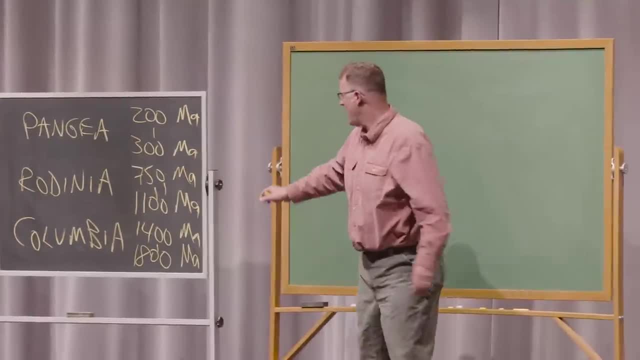 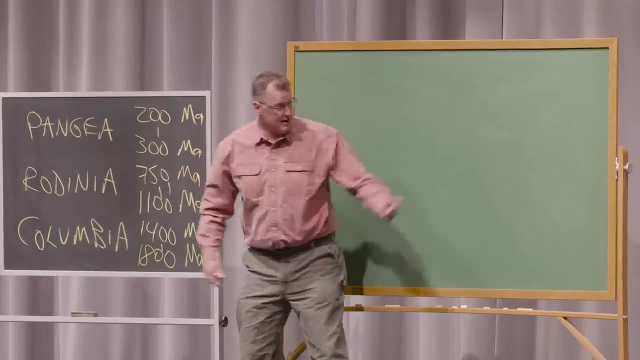 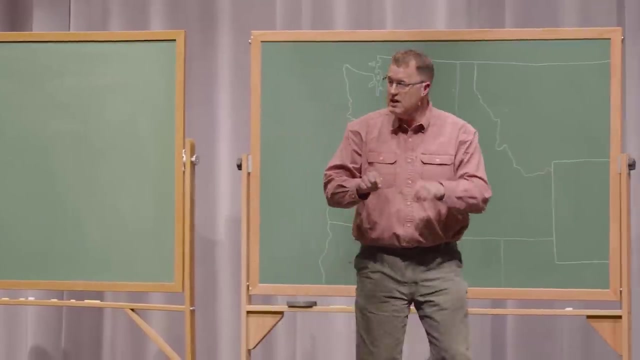 All right, Maybe I figured that was the case, So I'm going to keep this on the stage up here As a reminder. it's not going to change the rest of tonight And now I'm going to work with these two guys for the next 20 minutes or so and try to use Northwest geology to somehow eventually 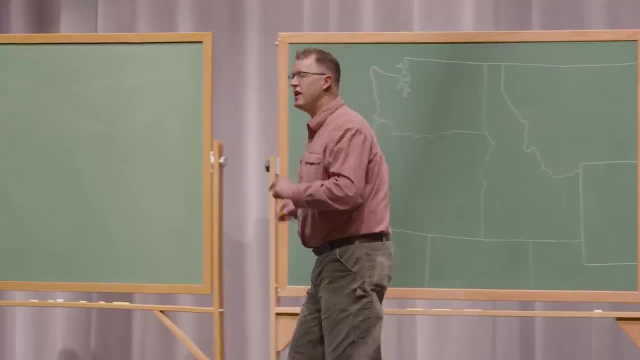 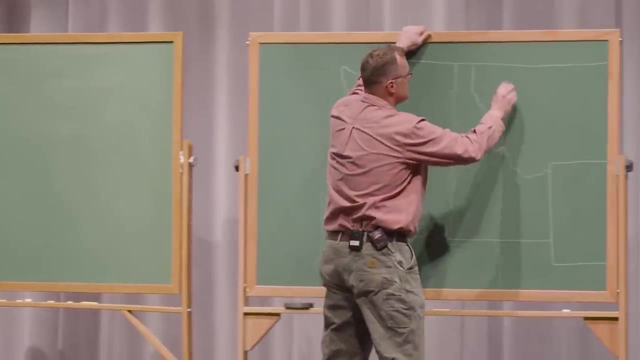 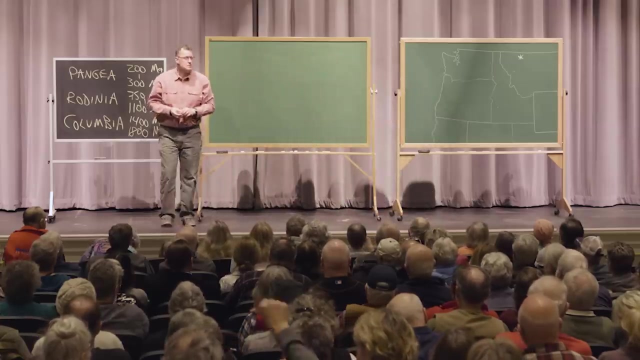 plug back in. Okay, so let's switch things up. I think we need a break from this. Let me tell you a story, And the story takes place in a national park that's right there, Glacier National Park. So the story takes place in a national park that's right there, Glacier National Park. 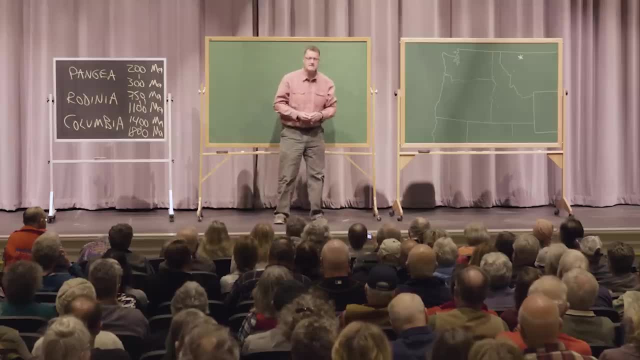 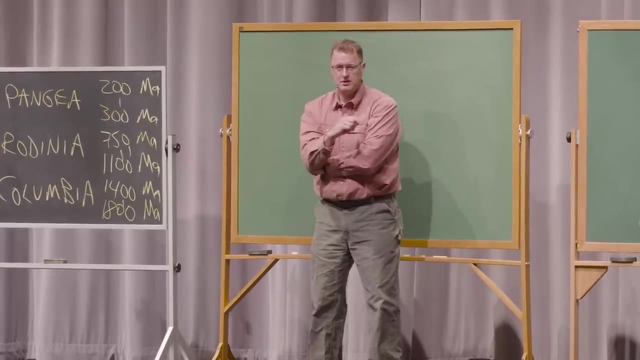 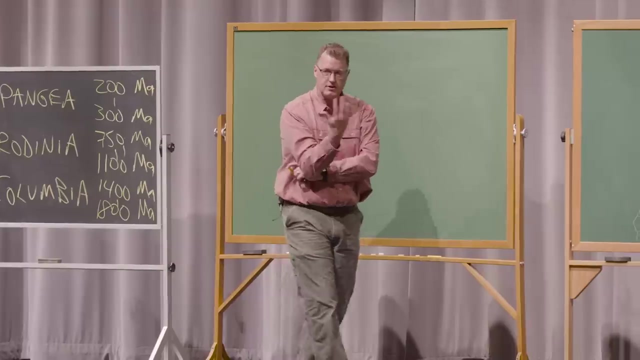 So the story involves my favorite subject, me. It was the summer of 1983.. It was the summer that I was turning 21 years old. I was going to school in Wisconsin- That's where I'm from- Madison. Three years in college, no direction, no major. 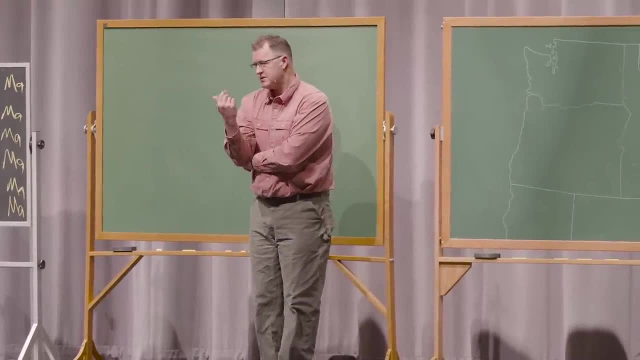 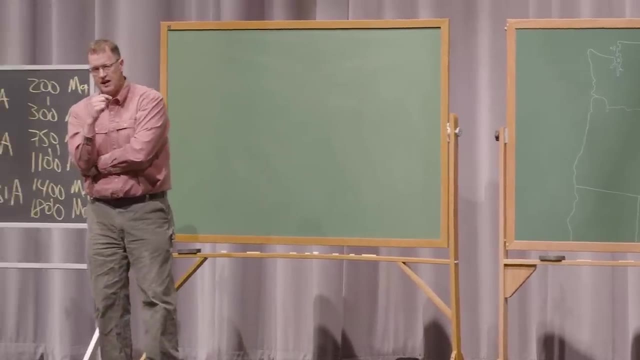 couldn't find anything that interested me, Ran out of money, basically Took a train from Madison, Wisconsin, to Glacier National Park in June of 1983.. I mean, how old am I? I'm taking the train. for goodness sake, It's not that far. I didn't have a car at the time. 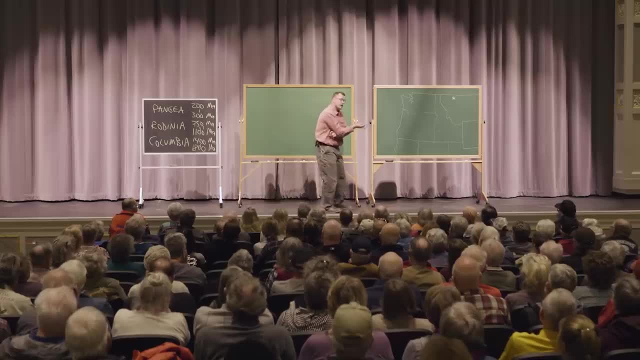 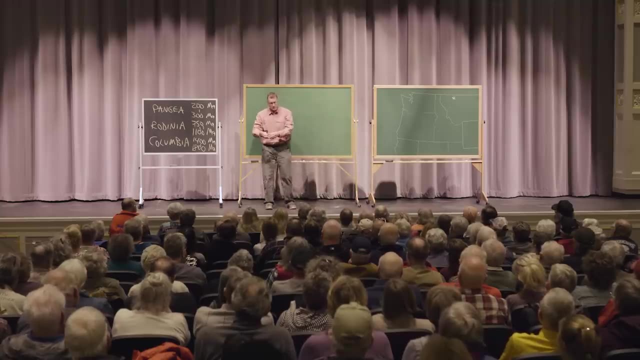 Great. My job, my summer job, was to work at Lake McDonald Lodge on the west side of Glacier Park. Many of you have been there. There's the lodge, there's the general store. there used to be a little gas station and my job was to pump gas and to sell souvenirs at the general store. 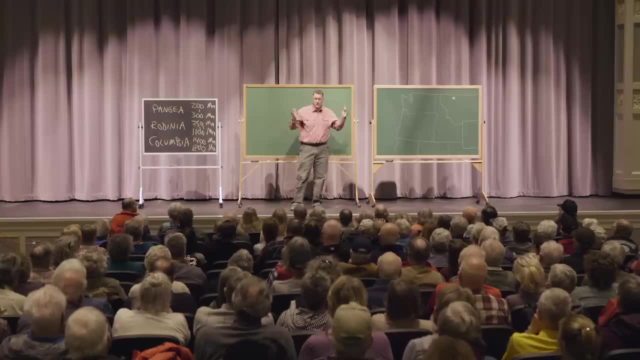 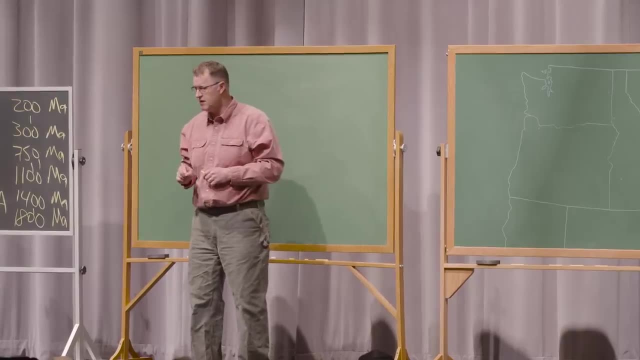 with a bunch of other college kids who were there for the summer, from all across the country. I'm telling you this story because it was my first time living in the west, It was my first time hiking in the mountains, and it's the summer that I discovered geology I had no interest in. 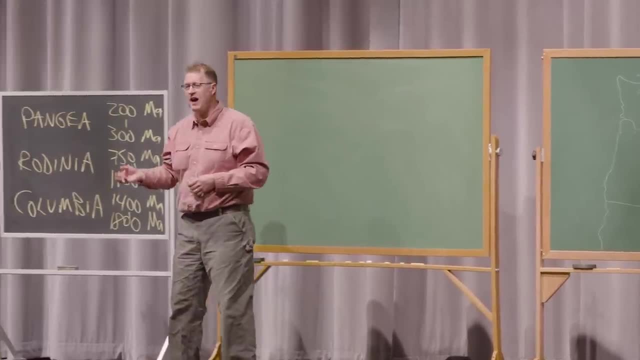 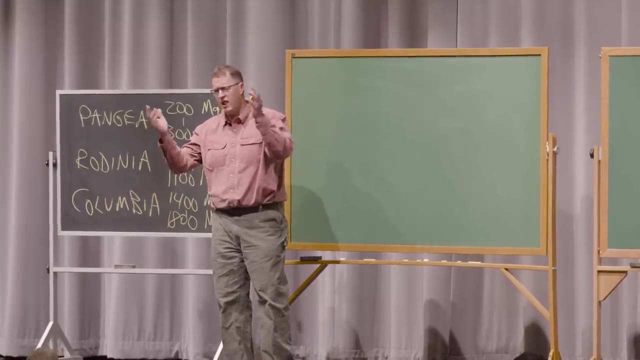 geology before that summer. But I did these day hikes, I did these visits to these places that really surprised me. First of all, the scenery was beautiful. We all have that experience. But there was one particular day hike I want to tell you about as quickly as I can. 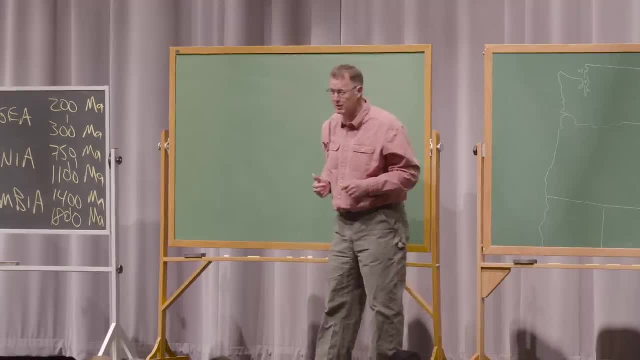 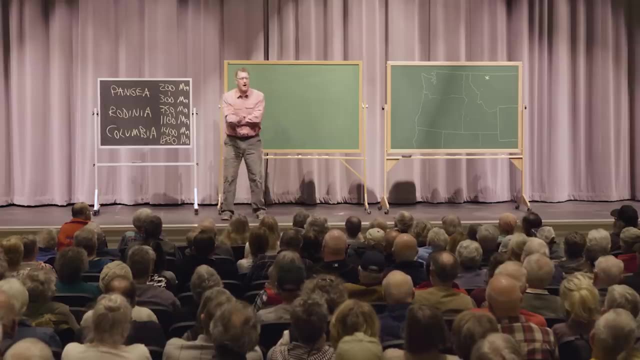 I've got photos I'll show you from that actual hike in 1983.. We're going into the archives tonight. So Craig and And Webb and Bruce and I jumped in Craig's car. We drove from Lake McDonald up the Going to the. 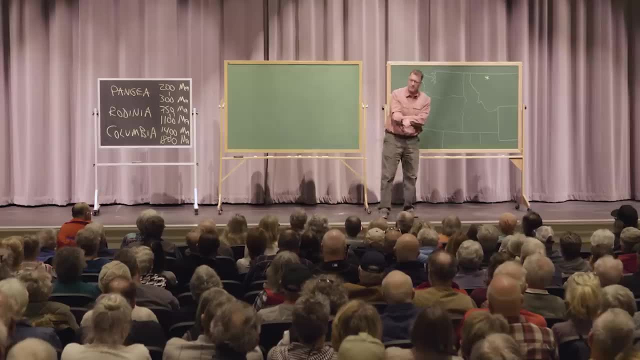 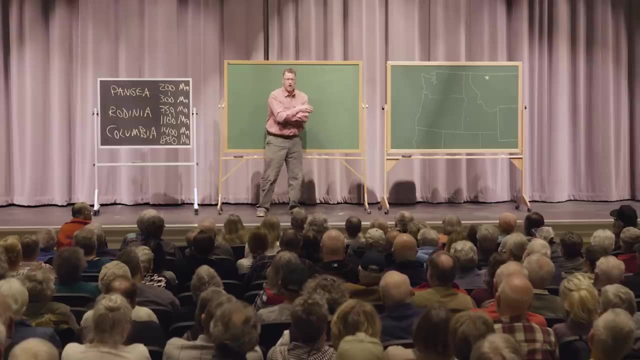 Sun Highway to Logan's Pass. Many of you have been there. We parked right at that big parking lot early in the morning. We hiked north on the Highline Trail- Pretty easy walking- And then at some point Craig said we're going to the top of Mount Gould, Are you ready? 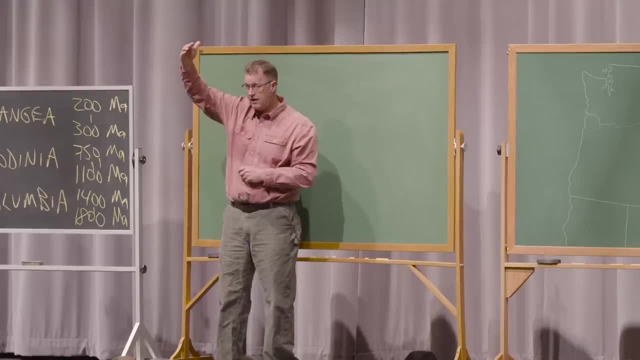 Mount Gould is the very top of the Continental Divide. in Glacier Park It's the top of the Garden Wall And we're all in our early 20s. Do you remember the days where you could just walk up a mountain with your hands in your pockets? essentially, I miss those days. 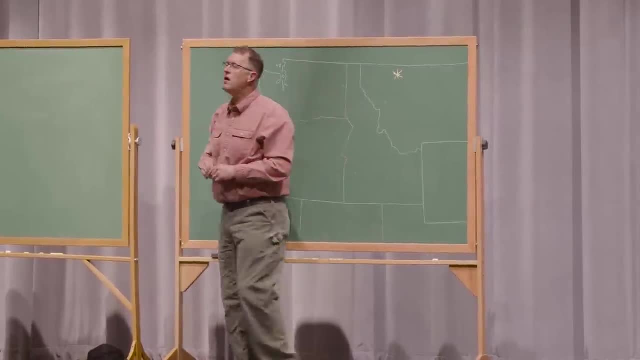 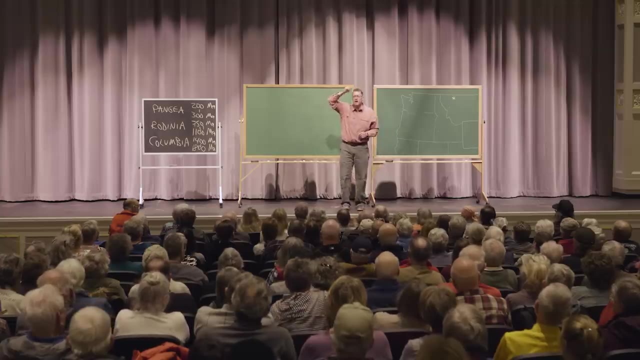 So it was two o'clock in the afternoon. We're on top of Mount Gould. We're up high enough that it's a bluebird day and we can see out to the plains of Montana. Some of you have experienced that. You're up that high, You can look down on Grinnell Glacier, down on Many Glacier Hotel. 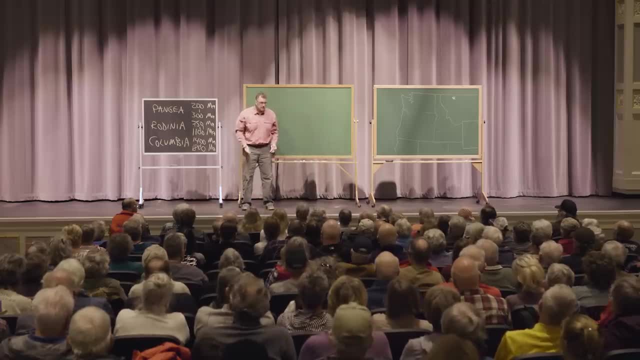 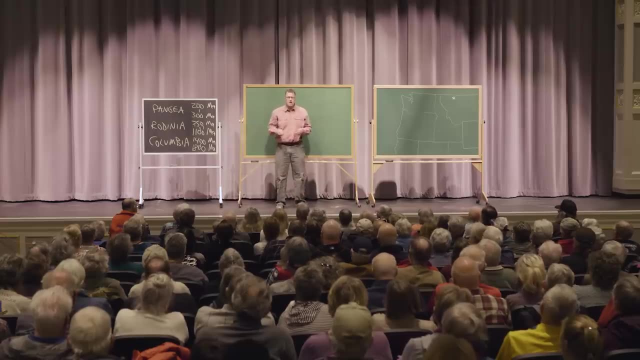 And I was a greenhorn. I was literally wearing my farm boots- Literally My farm boots from Wisconsin. All these other guys had all the hiking gear, But I was new to the whole scene And we had lunch. I had my little PB&J and a little packet. 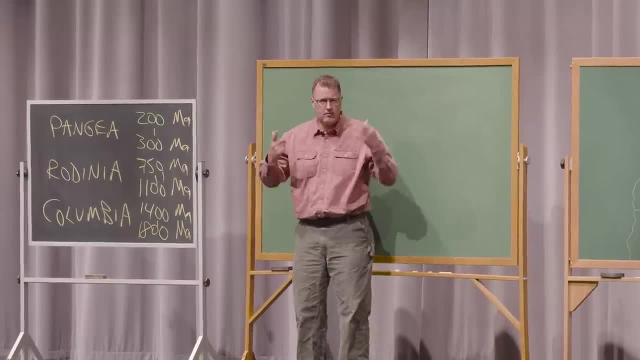 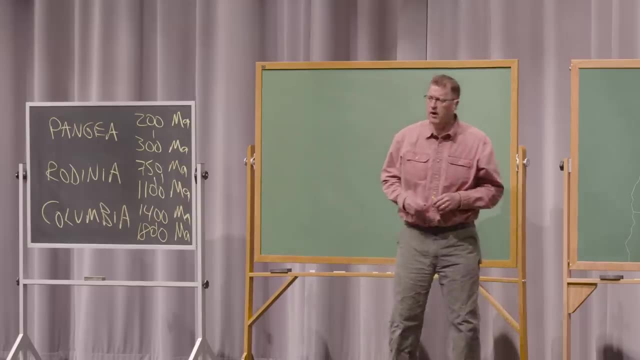 of Skittles, I remember, And I was sitting on this maroon rock up there on the top of Mount Gould And the other three guys were about 15 yards away from me, sitting on a different rock, And at some point Craig broke the silence and said: hey, you are so out. 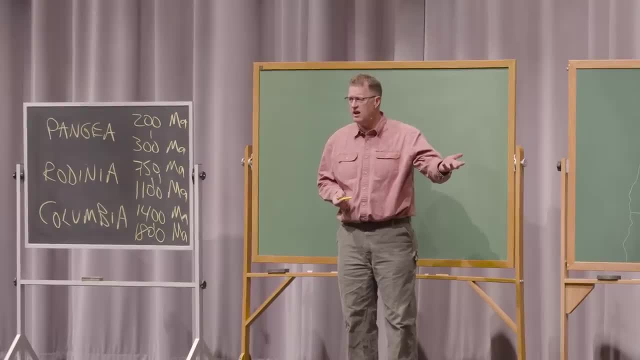 of it. Why did you pick that rock to sit on? Isn't it uncomfortable? And I'm like I don't know. He said you're sitting on a bunch of those ripples. Have you noticed? Aren't you uncomfortable? And it's true, I was sitting on this slab of maroon. 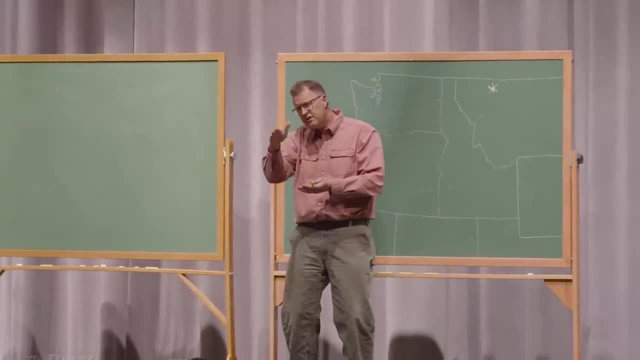 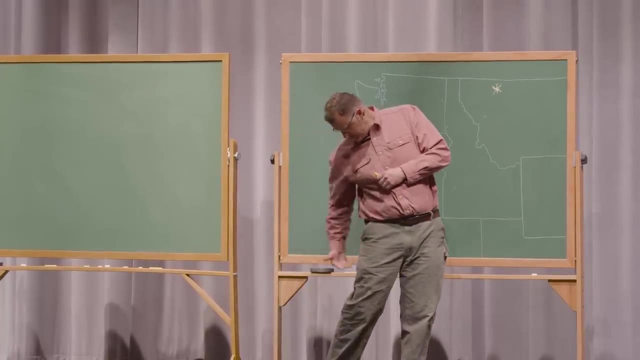 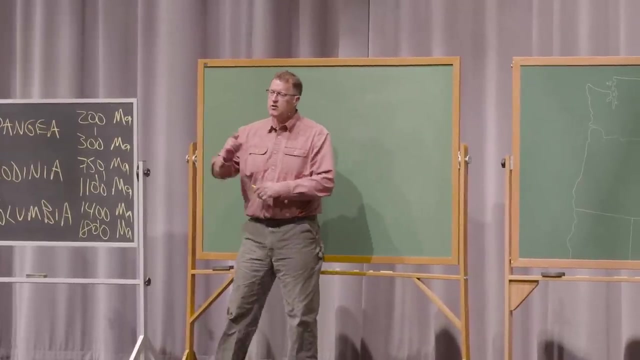 rock that had these beautiful symmetrical petrified ripples on the surface of the rock. And I was like, oh yeah, I had these red stripes on the back of my bottom and my thighs. And then Craig said: do you know how those ripples formed? In a kind of a show-offy way. 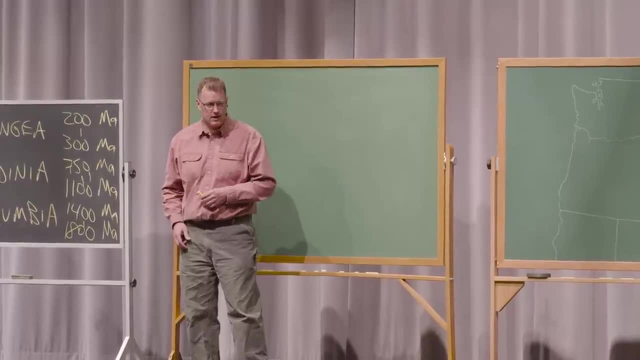 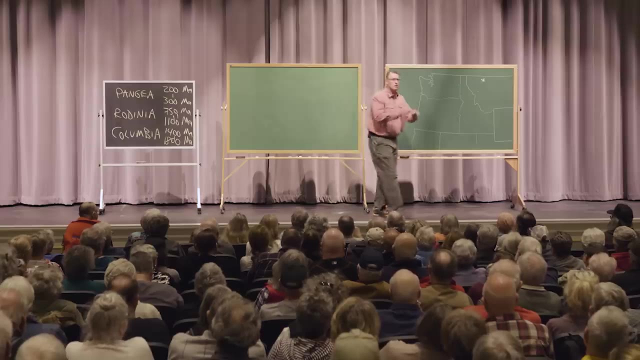 This is 1983. You can't just pull out your phone and like double check what the guy's saying. you know He was like this used to be a beach. I took Geology 101 at Oregon State University and I learned that these ripples formed at the beach And I'm like, yeah, bullshit. 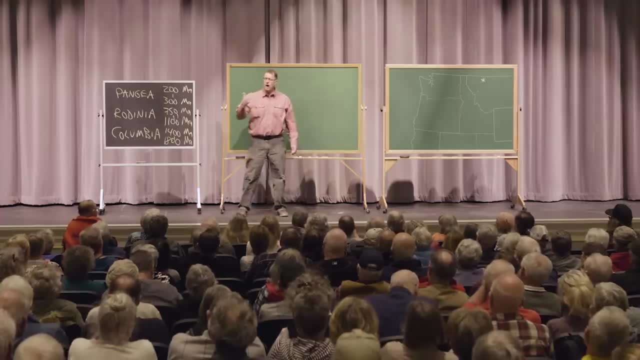 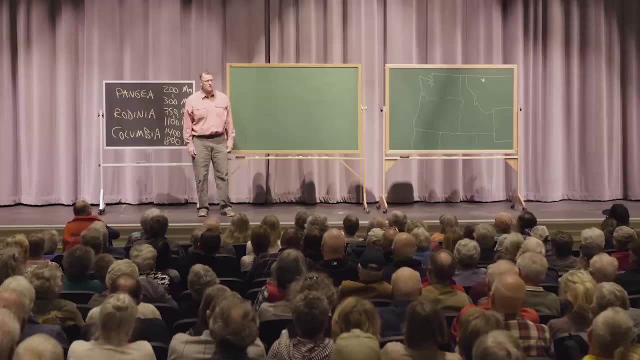 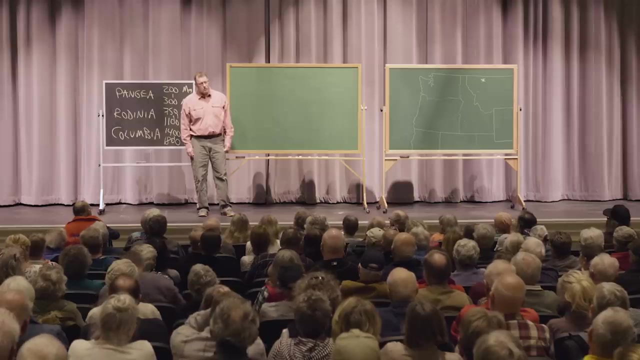 That's not good. And he kept talking about this beach thing and the coastline. This was the old coastline And all the other guys were like nodding their heads And I'm like I don't believe you. Okay, I'll finish the story. Craig was right, Those rocks are pre-Cambrian rocks. that clearly. 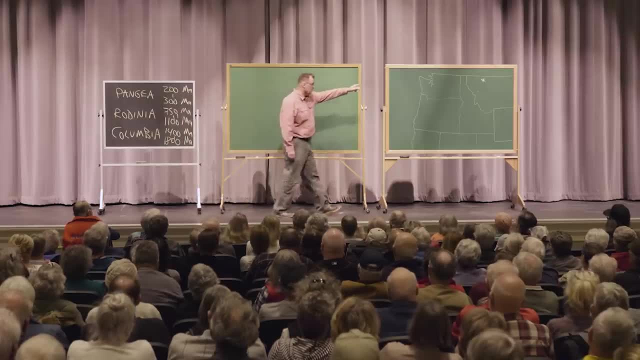 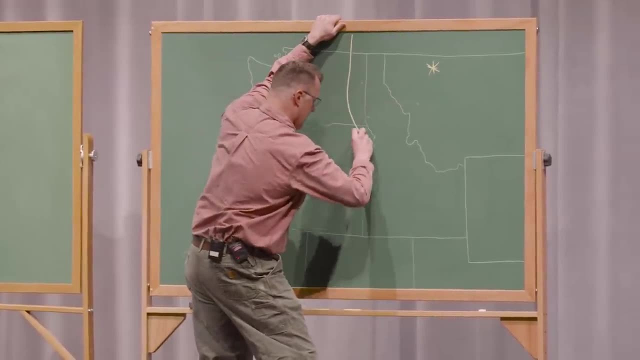 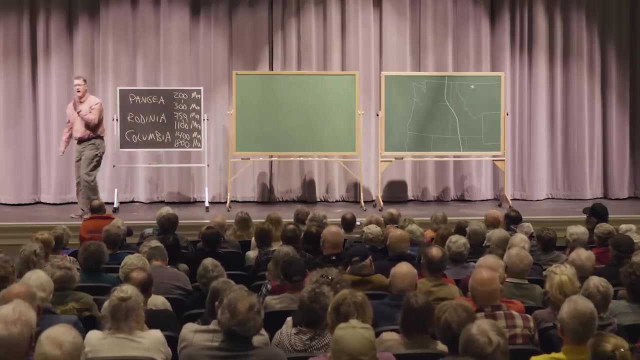 formed at the old coastline of North America here And those rocks are all through this area. Let me draw a line for you. This is a very clear line on that map of the Pacific Northwest And that line is the true coast of the Pacific Northwest or the west coast. 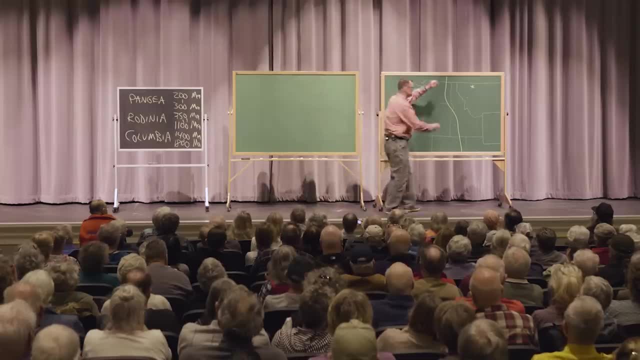 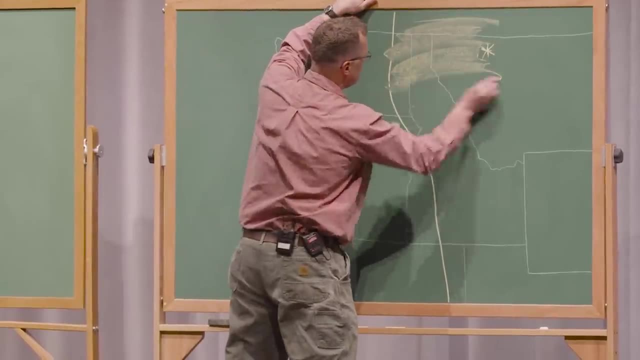 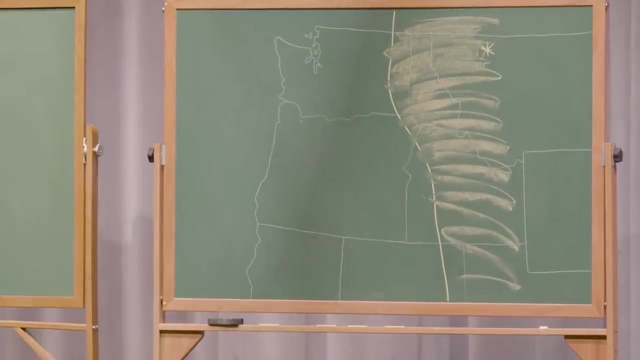 of North America for hundreds of millions of years. And Spokane is right here if you can see that gold dot So pretty much everything between Spokane and Glacier Park. And those rocks continue to the south, down to Vegas and even into Mexico and north up through. 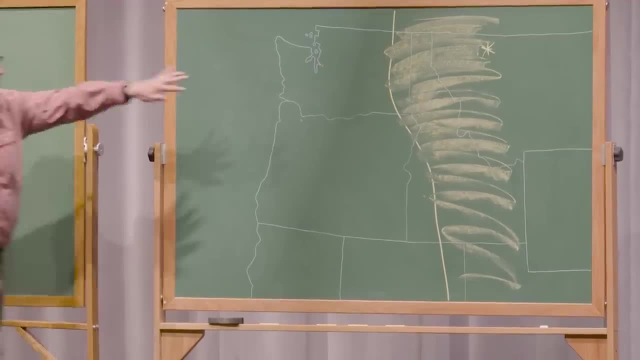 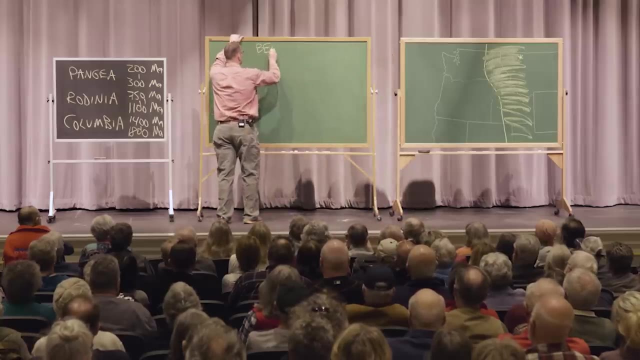 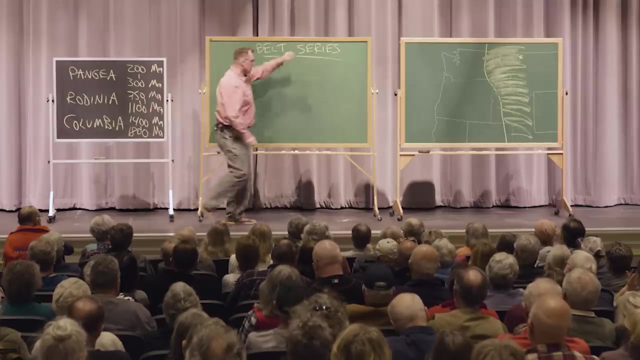 Canada. These are all beach rocks. These are all rocks that are going to be found in. the are muds and sands, and they are called, at least in the United States, the Belt Series or the Belt Supergroup. It's where the Rockies are today, but this predates the Rocky Mountains. 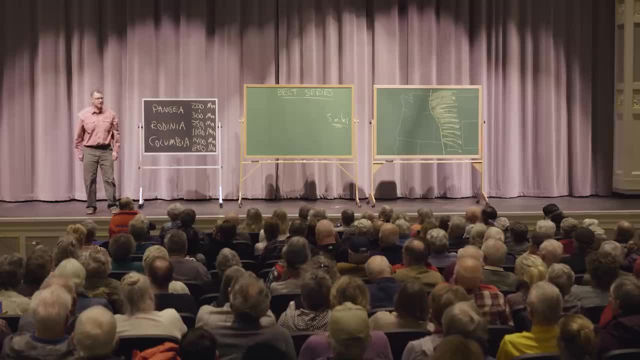 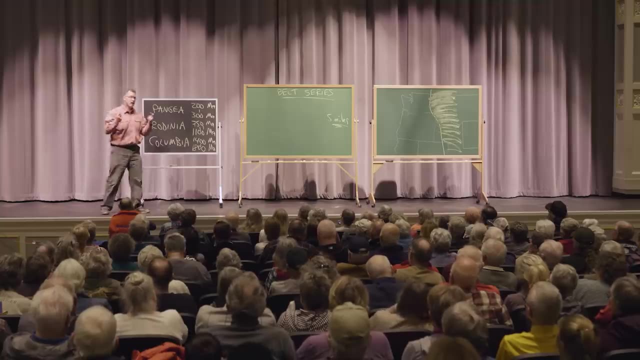 That was my confusion. eating my Skittles, I'm like I don't get it. These are the mountains. What are you talking about the beach? for? You can go from a beach scene to a mountain scene if you have enough time, and that's what we're talking about here. Collectively, these layers of rock. that were originally sedimentary rock and are now metamorphic rock, the Belt Series located on that map. there- Glacier Park, Spokane, Steptoe Butte, Caulville, Chewila, Medical Lake, Libby, Bonner Ferry- take your pick- All those plots have belt rocks located there. They're beach rocks, They're. 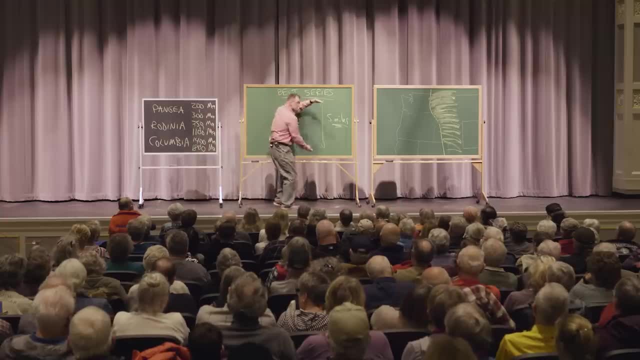 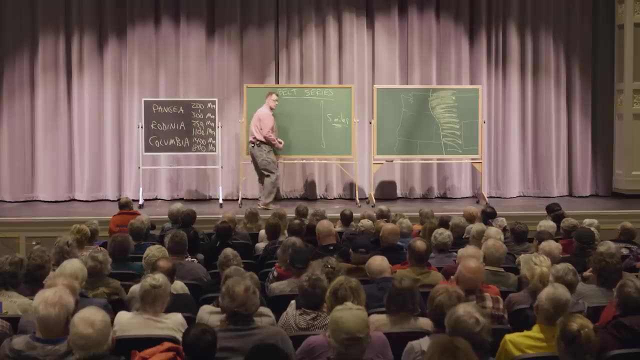 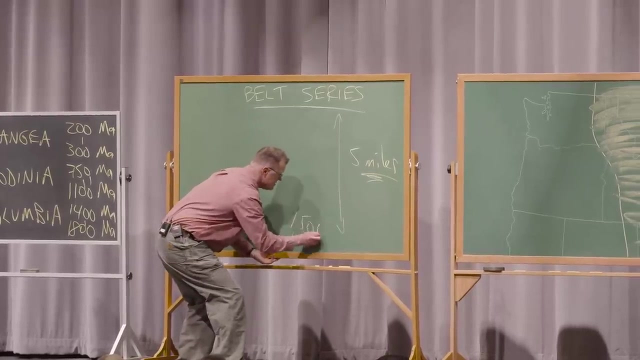 pre-Cambrian aged rocks. In total, that cake is five miles thick- 25,000 feet worth of sedimentary rock deposited at the coastline of North America. We have dates now. Dates for the belt: 1,500 million to 1,400 million. 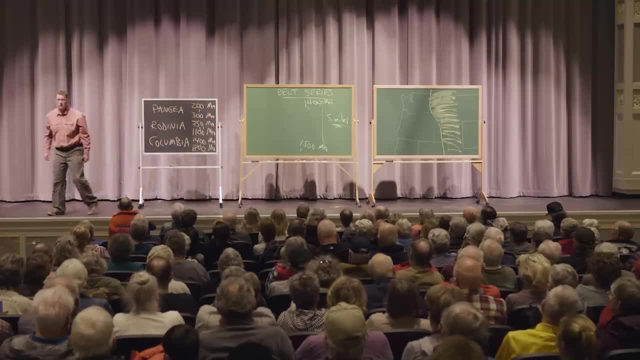 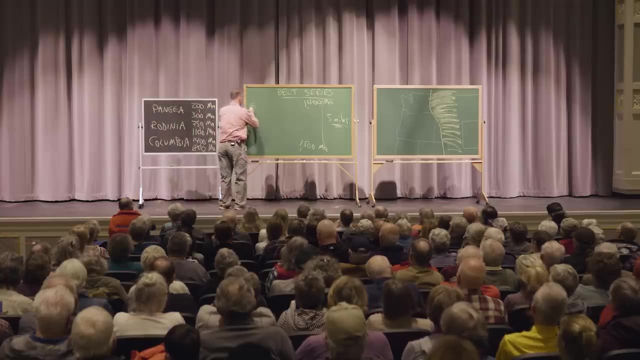 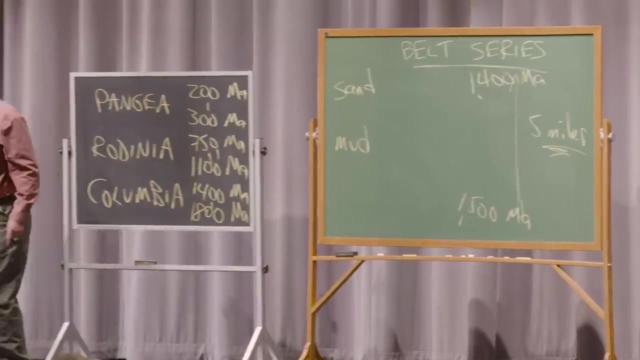 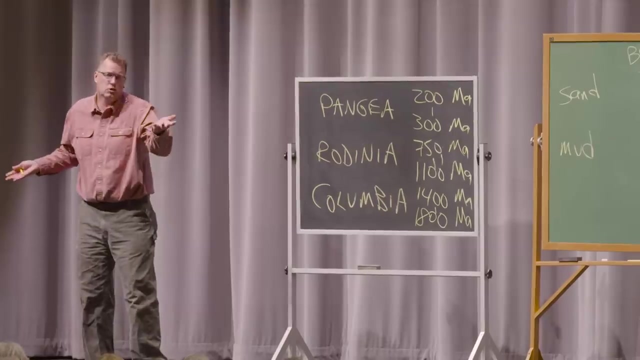 Seriously old. During that time we deposited all of those beach rocks Now. originally it was sand at the beach and mud at the beach. Those ripples I was sitting on beneath the patch of Skittles, was a tidal zone, was a muddy zone. You've been to the beach, The coast of Washington. 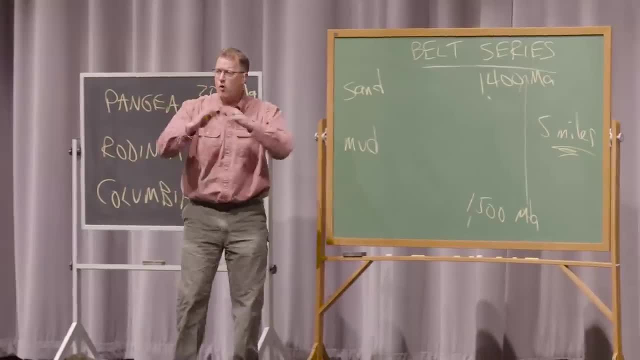 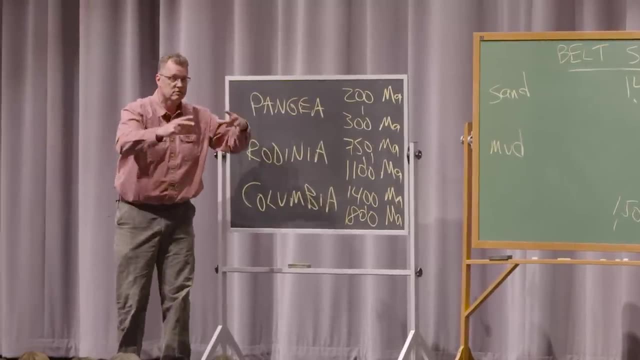 has a lot of mud right And you have drying mud that forms cracks. You have the ripples. In certain places off the coast of Australia you can get stromatolites, these big mounds of blue-green algae, stromatolites that are fossilized in this mud. 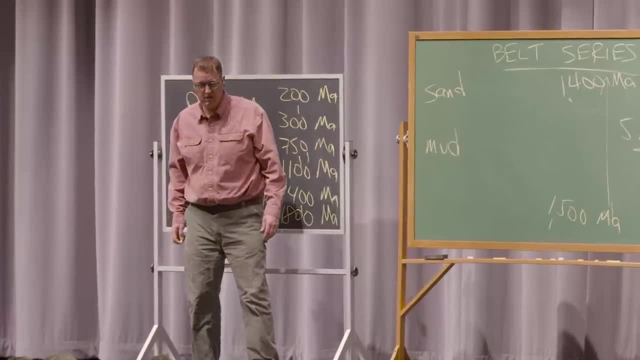 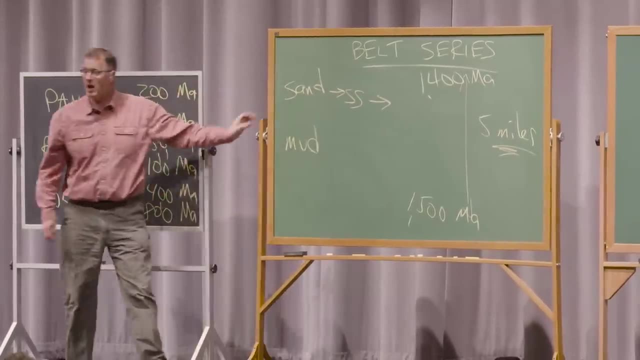 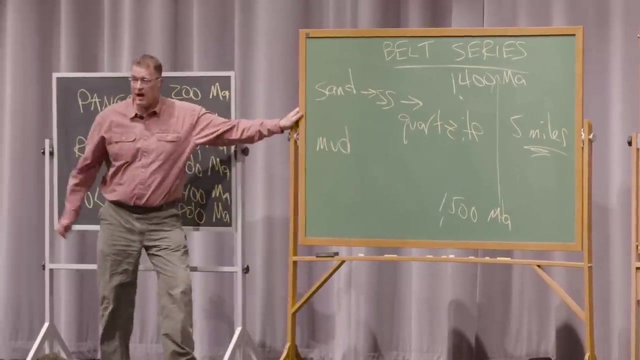 And sand. we all know sand is at the coastline, at the beach, But originally the sand got buried into sandstone and the sandstone got heated up and pressurized to become quartzite And the mud got buried to become a sediment. 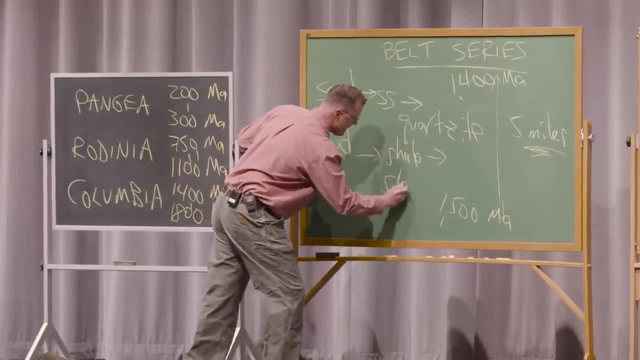 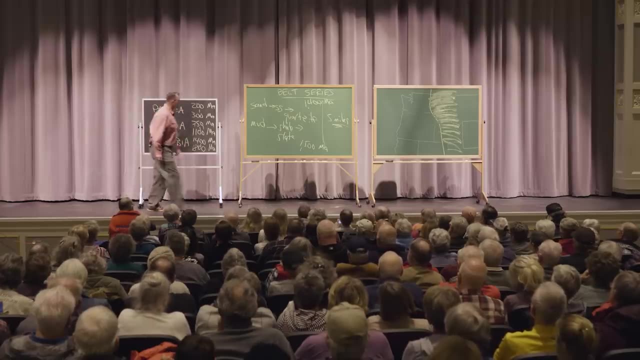 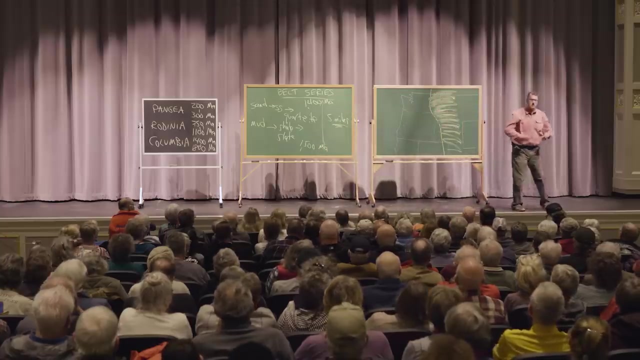 rock called shale, and the shale got buried to become a metamorphic rock called slate, and the slate sometimes turned into argillite. So what are the belt rocks today? Rocks of this age representing an old coastline, interbedded layers of quartzites and argillites- quartzites and 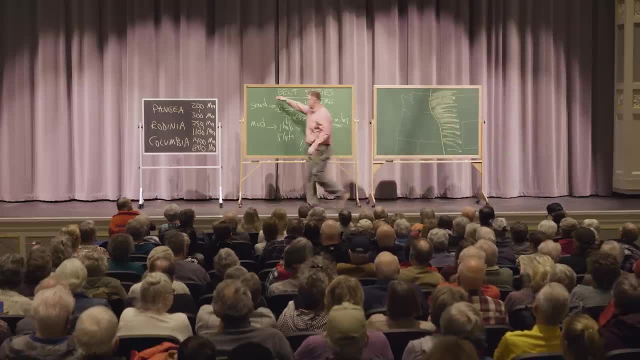 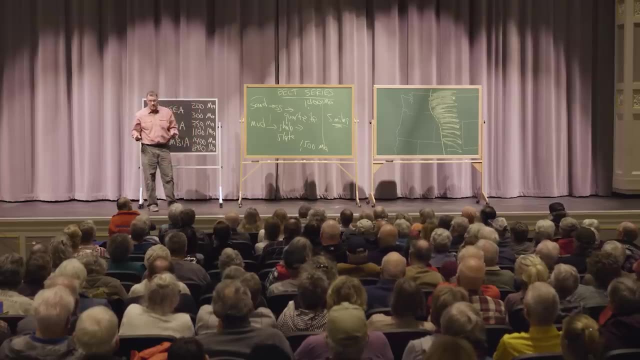 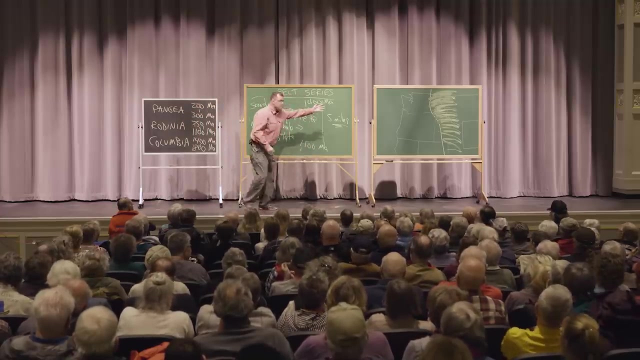 argillites, but we don't care that they're metamorphic today. We care that they were originally deposits at the beach. The energy in the room is great, and we're now to the juicy part. We haven't even gotten to the good stuff yet. Now, this is what I've been teaching for a long time. 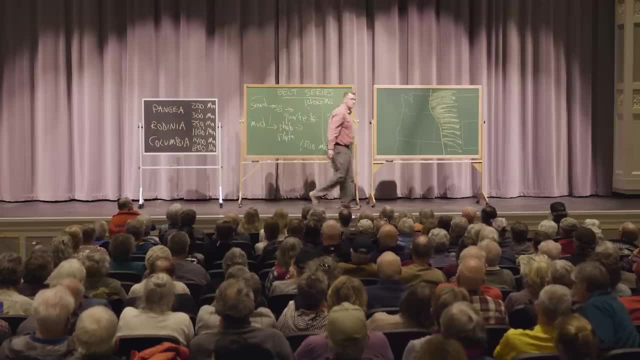 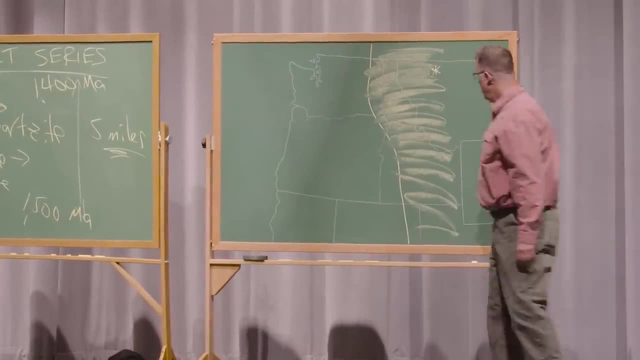 and I would not only draw what I just drew here for you, but then I would say to my students over the last 25 years: where do you think all that sand came from? Well, it's the coast, isn't it? Aren't we going to? 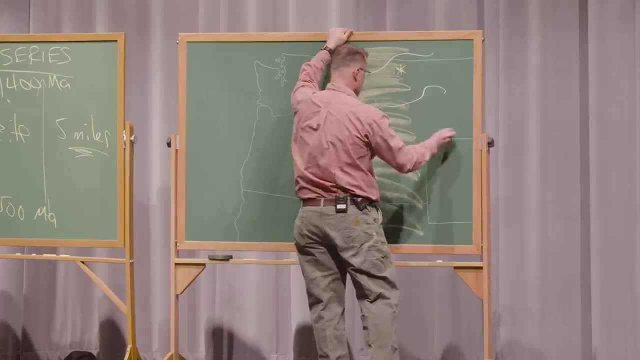 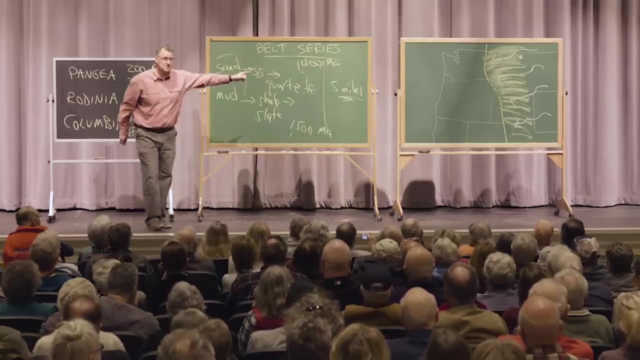 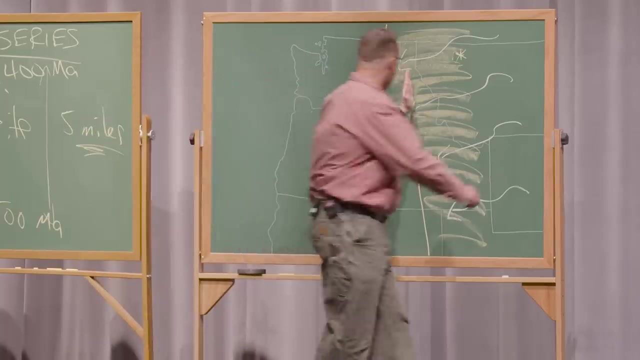 a assume there were rivers draining North America at the time. I hope it's clear to you: Washington doesn't exist yet, Ellensburg doesn't exist yet, Oregon doesn't. This is deep ocean. This is open ocean, but we're talking about all this sediment accumulating at that shoreline, the belt. 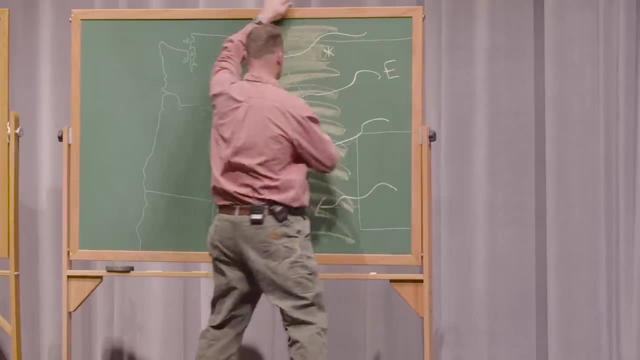 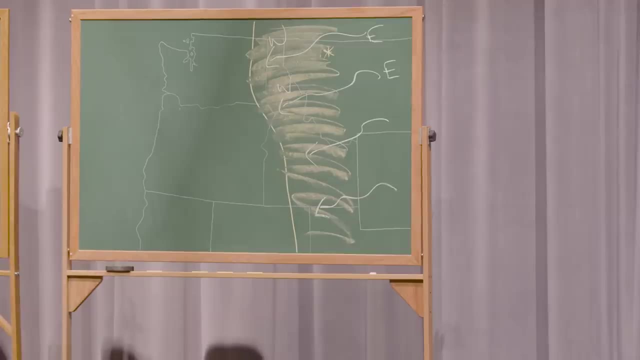 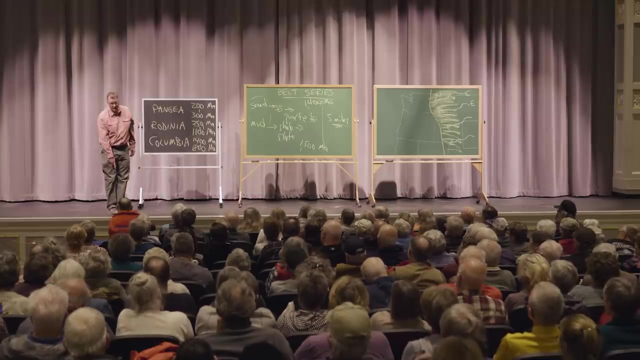 and we're assuming that the rivers are flowing from east to west, and that's true. A lot of the sediment in the belt came from the east, from the interior of old North America, and drained to the coast. You ready, I'm leaving stuff. I've taught forever to stuff. I've never taught stuff that. 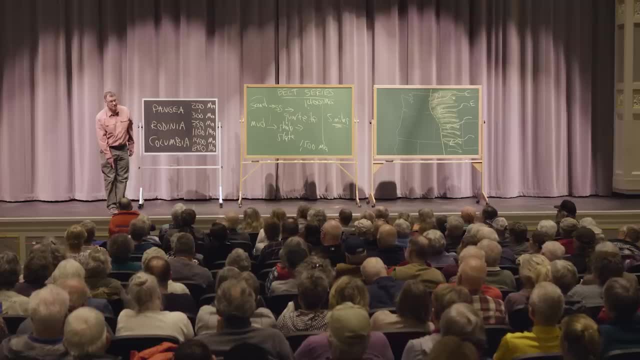 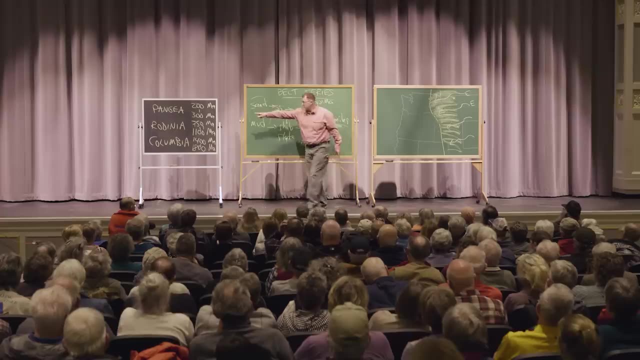 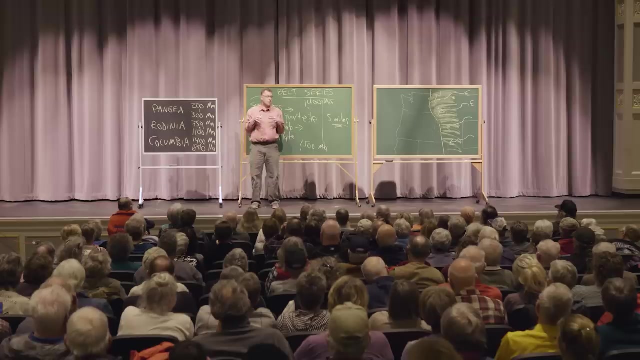 I've learned in the last 10 days. It's good, Here we go, Because remember the gimmick of the lecture I'm going to somehow say the belt has something to do with this. This is just a coastline and yet I'm saying there are times when all the continents of the 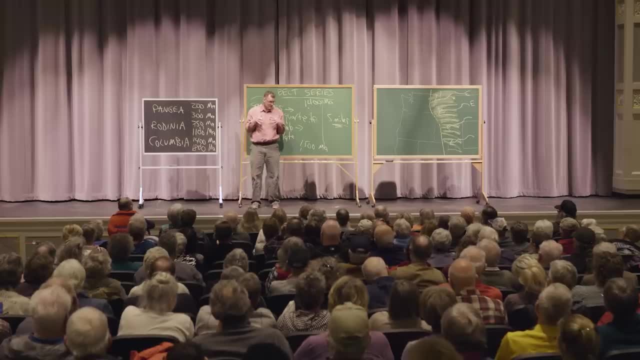 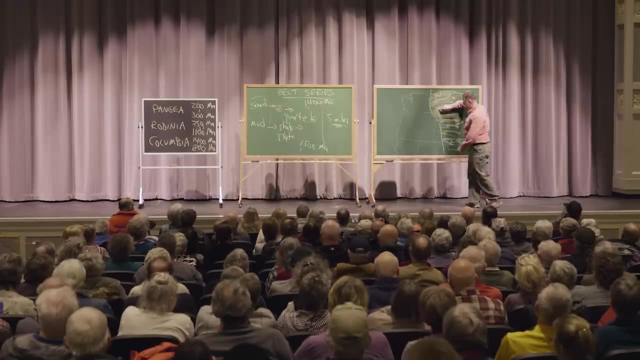 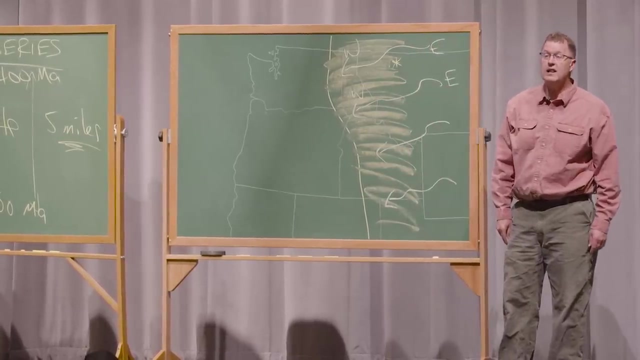 world are hooked together. Some of you are a few steps ahead of me possibly, especially when I say this. For years, it was clear that when you carefully study the sand in the belt, not all of it came from the east. There were paleocurrent indicators, details written in the quartzites and 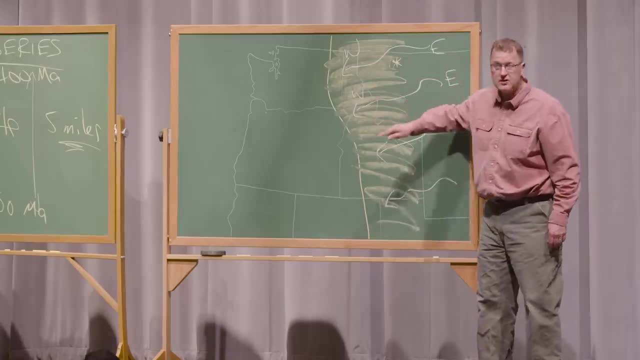 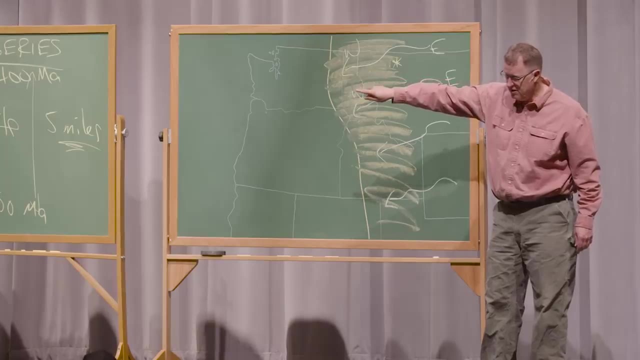 the sandstones to say, a bunch of the sand in this belt came from the west. Now let's pause and think about that for a second. Is that possible? You can't have a river come out of the deep ocean and come onto land and 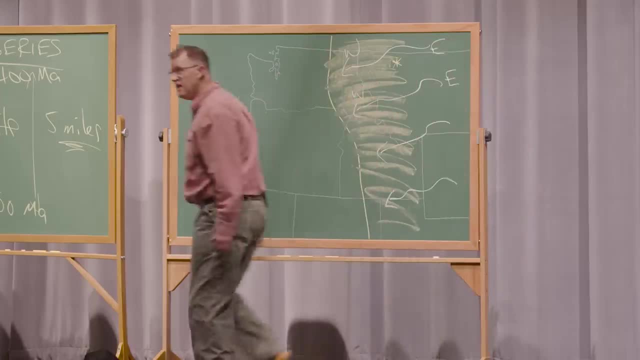 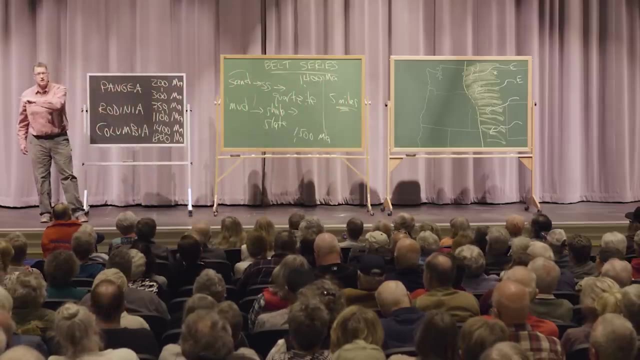 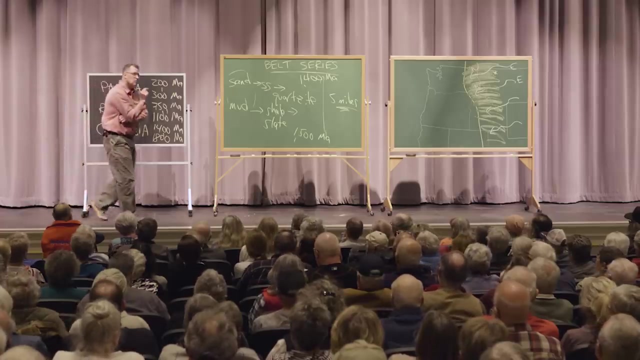 bring sand. There's a lot of sand that looked like it came from the west. Next point: there's a new technique we talked about last year and we're talking about again right now: a mineral called zircon. Zircon is a very durable mineral. Many of the sand grains are zircons. As a geologist now, 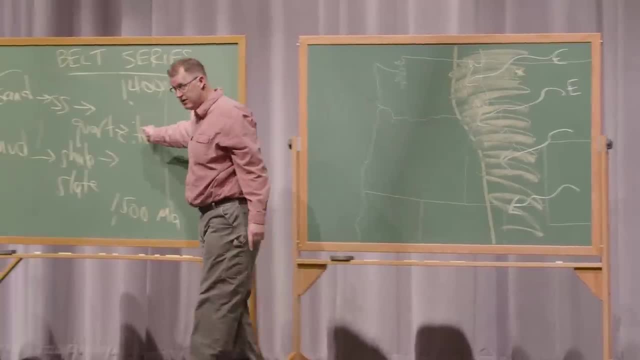 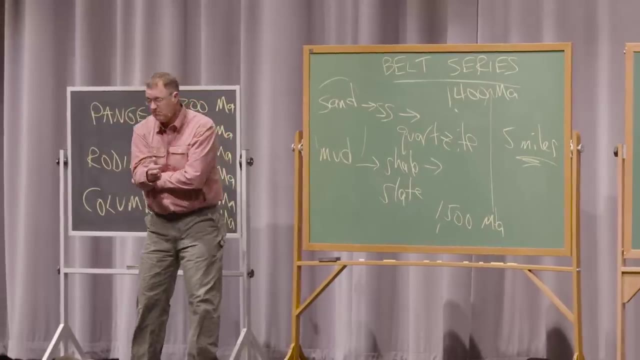 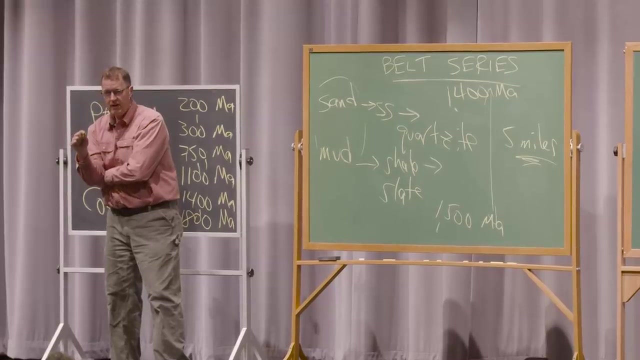 you can go out and collect sand grains from the belt, analyze the age and the chemistry and the rock type of those sand grains and find a source, find a place where those zircon grains came from. We couldn't do that before. Are you ready? 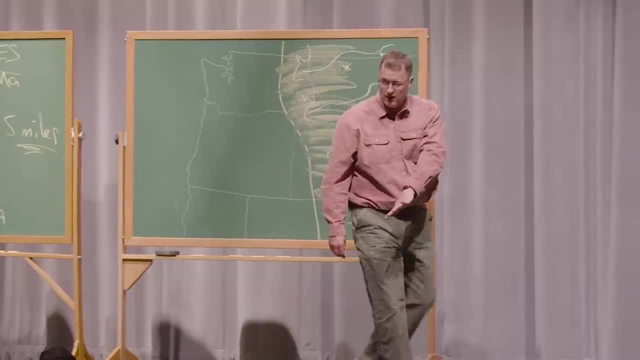 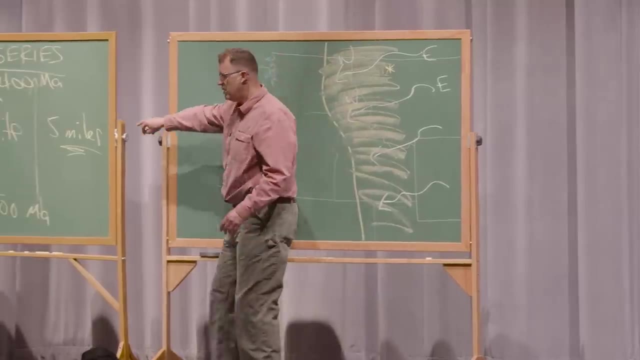 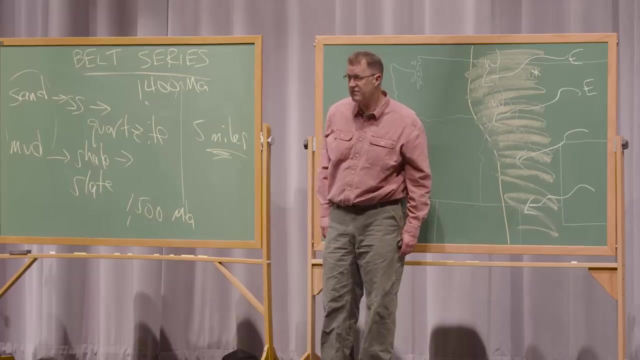 Paleocurrent indicators in a bunch of the belt, especially the lower belt and the zircon, say that a substantial amount of this five miles worth of sand is somebody else's. sand is exotic sand is not sand from North America. There's not a match to interior North America. 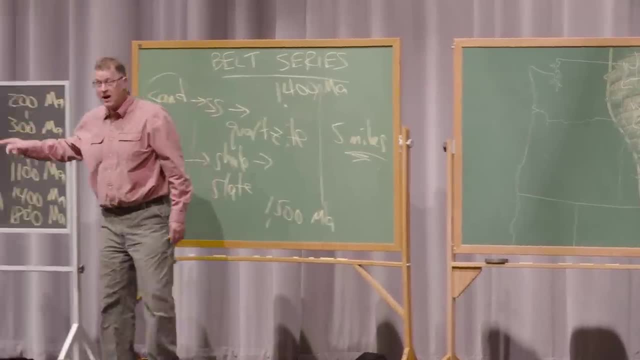 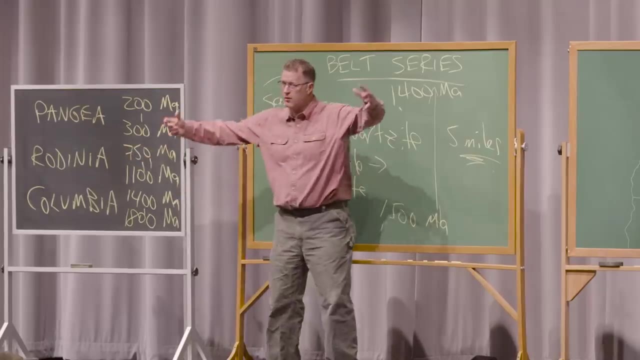 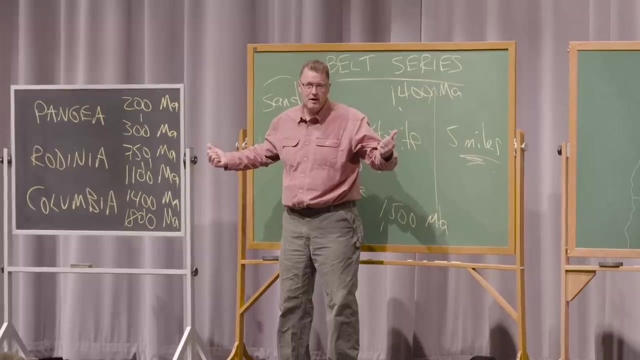 There's a match where Somebody else's continent Now hold on. When we have a supercontinent, we have continents coming together and soldering together for a while before they then decide to split up. Don Winston, who spent most of his career on the belt, he's a. 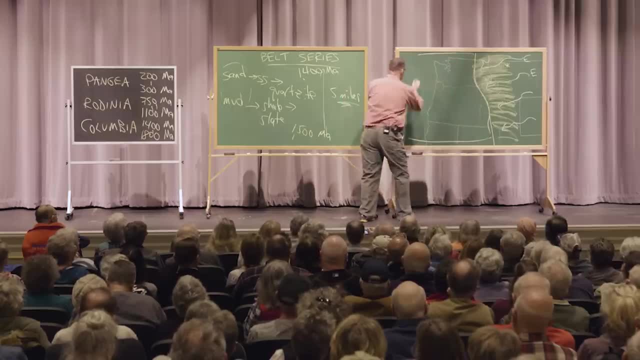 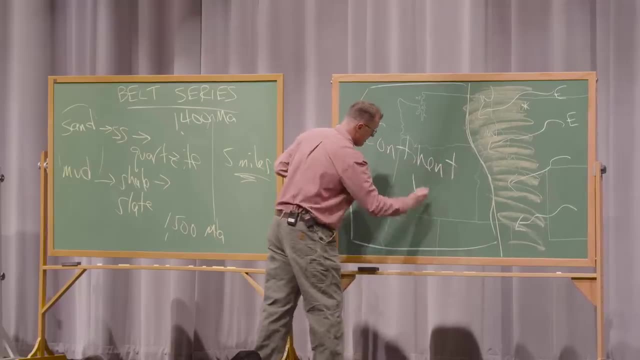 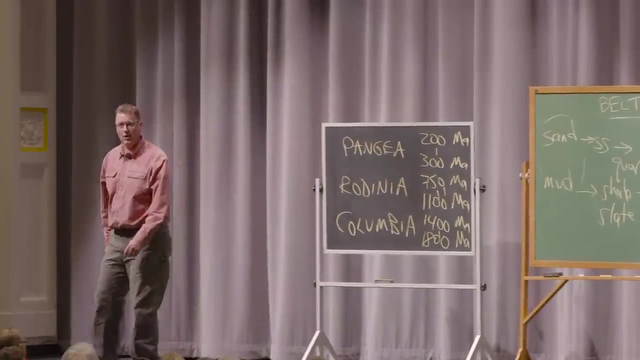 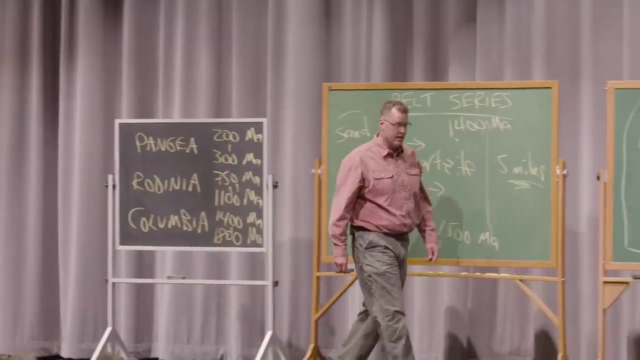 geologist in Montana would have maps and during belt time would say: even in some scientific papers, Don Winston would say continent X, continent X. I don't know what continent it was, but it was some. somebody was here, Somebody was docked right at Spokane and then took off at some point. 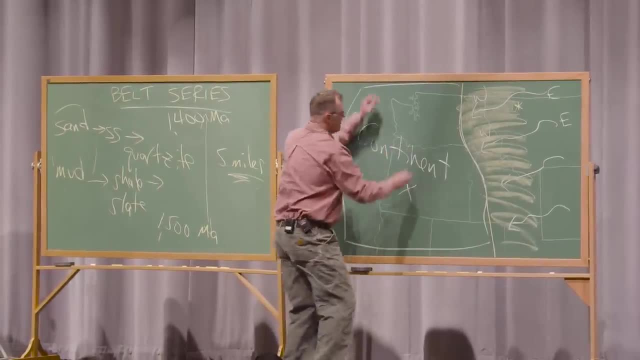 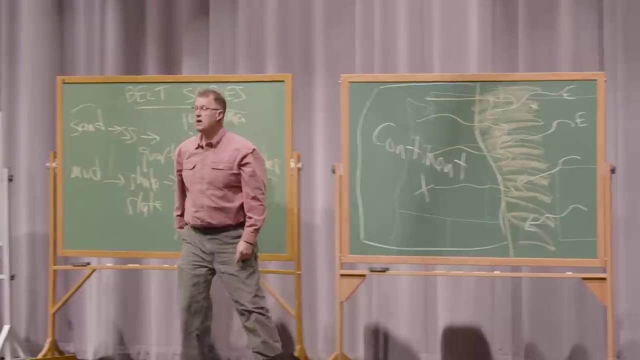 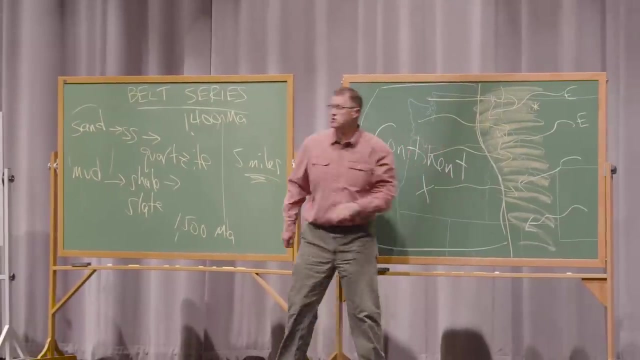 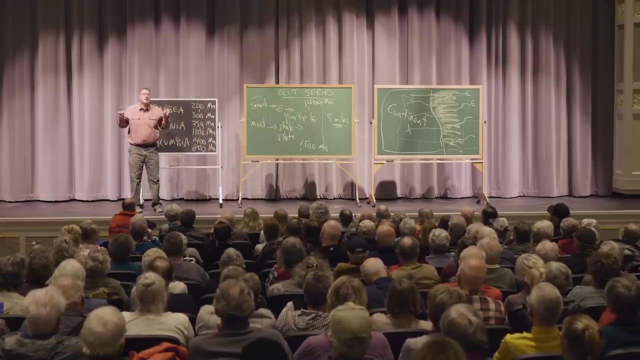 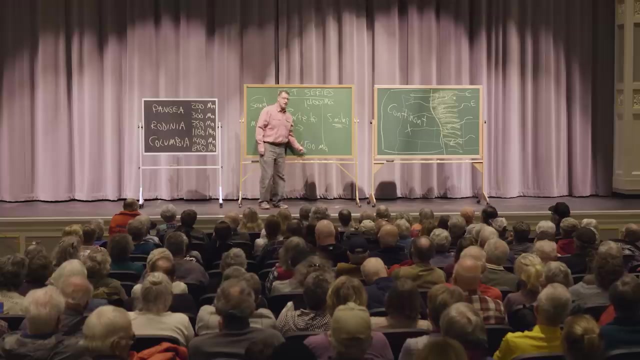 But the concept is we need continent X because we clearly have a continent with rivers flowing from West to East and depositing the sand into the belt from a different source. Let's pause again and then we'll reveal continent X. Look at the age of the belt. Does this work age-wise with Pangea? Of course it doesn't. 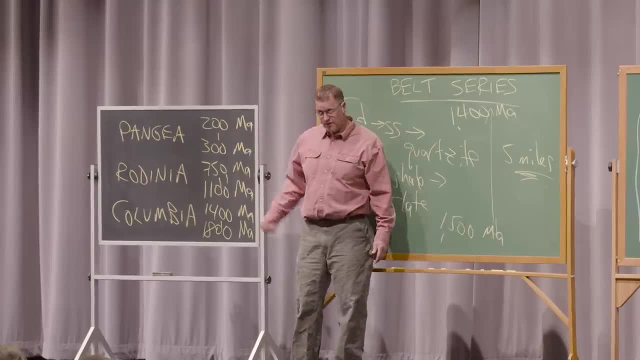 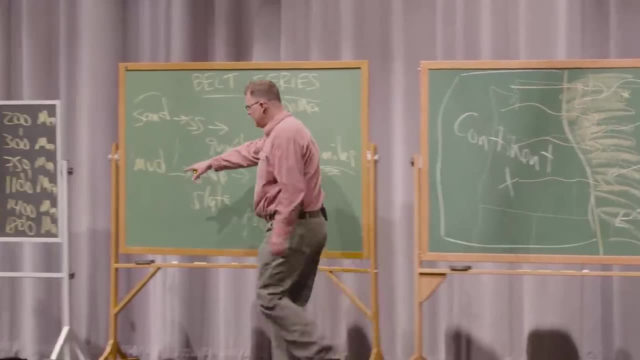 You've already done this. Does it work well with Rodinia? It doesn't work well with Rodinia as well. Look at these dates: 1,500 million to 1,400 million. that's the last 100 million years of the Belt. 1,500 million to 1,400 million: that's the last 100 million years of the Belt. 1,500 million to 1,400 million: that's the last 100 million years of the Belt. 1,500 million to 1,400 million: that's the last 100 million years of supercontinent Columbia. 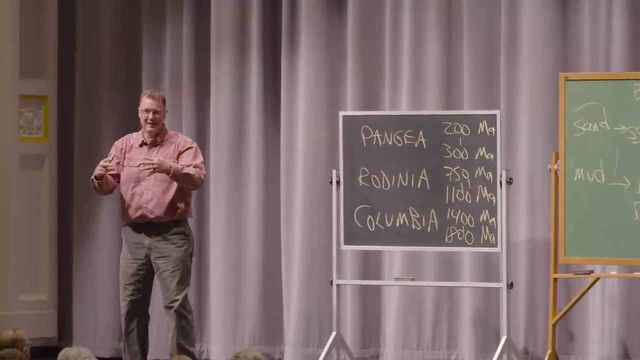 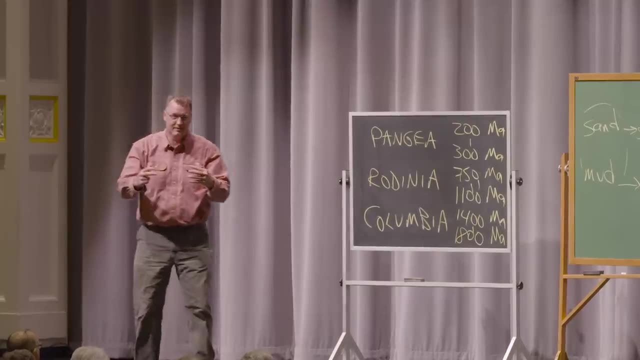 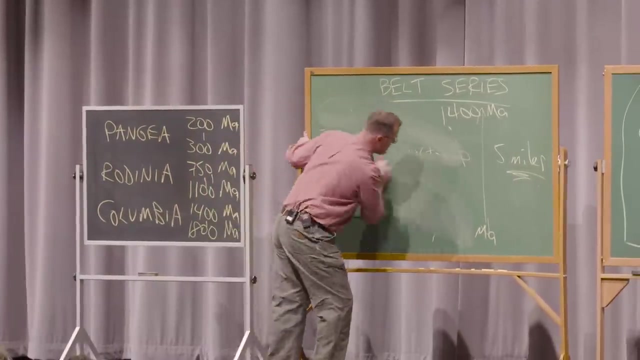 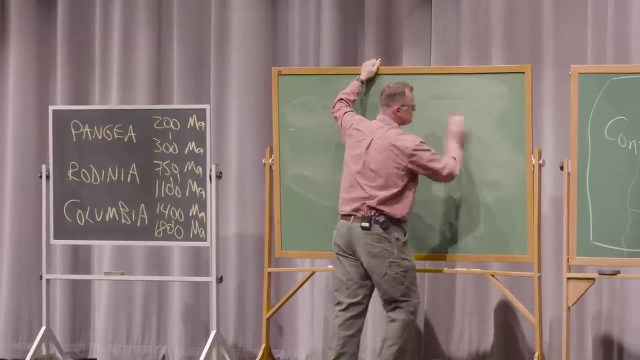 When all the continents of the world were together, When North America was connected to Australia, Continent X was Australia. Now, let's draw that and possibly turn your telephones off at the same time. Can we multiply, Can we multitask These new inventions called cell phones with ringers? All right, 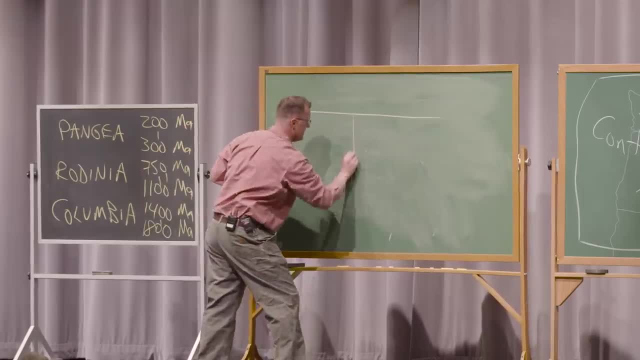 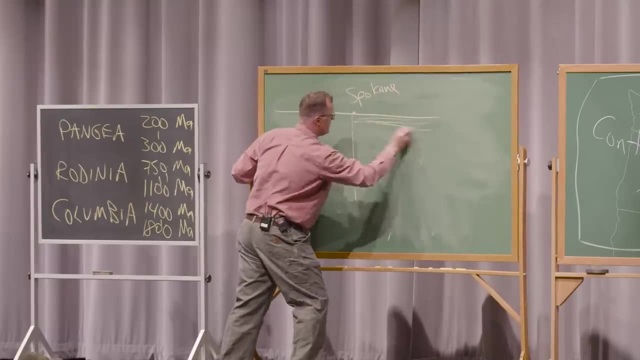 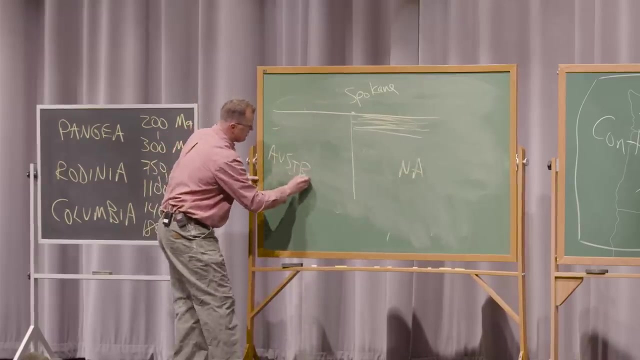 Let's do a cross-section of this same thing. Let's put Spokane here, Let's put the Belt at the coast of North America And yes, I revealed it verbally. Let's do it this way And I have to put an asterisk behind Australia. 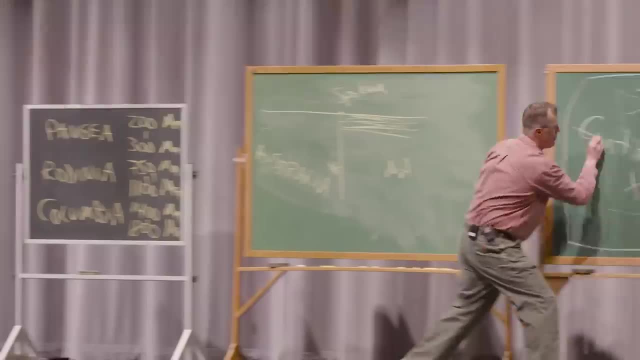 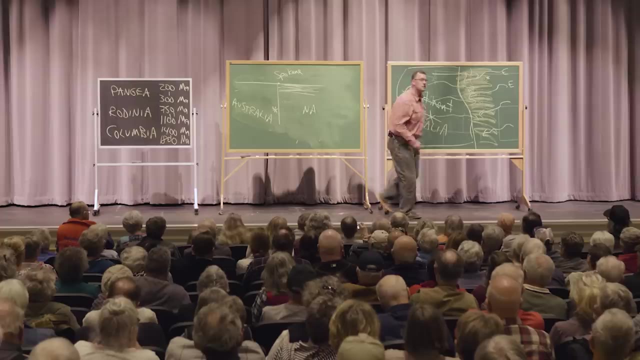 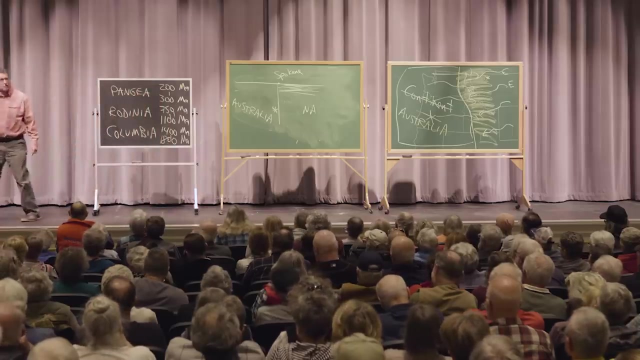 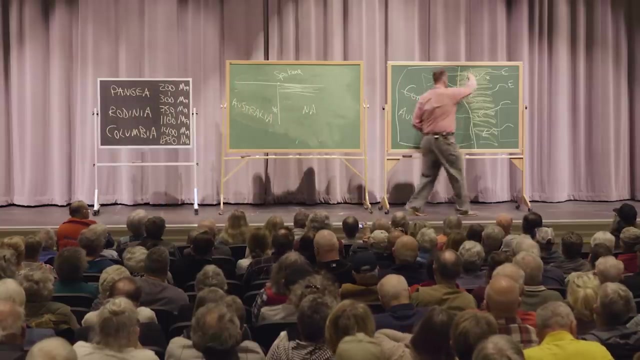 I'll tell you why. in just a second Australia You could have walked. if you have relatives in Australia, you could have walked from Northern Idaho to Australia. There was no Pacific Ocean at this time. Now what's the evidence? The evidence is you can study the zircons in the Belt and you can find pre-Cambrian. 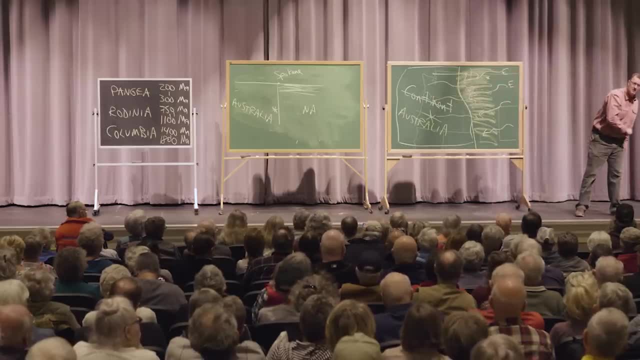 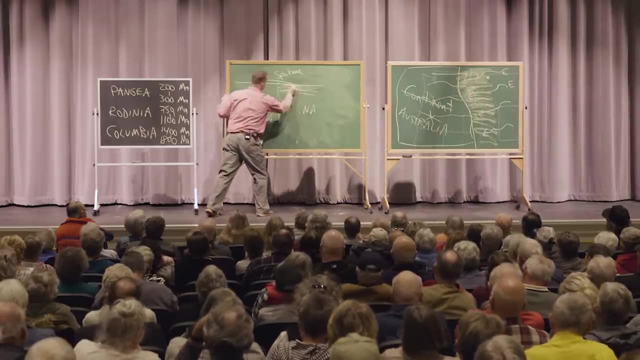 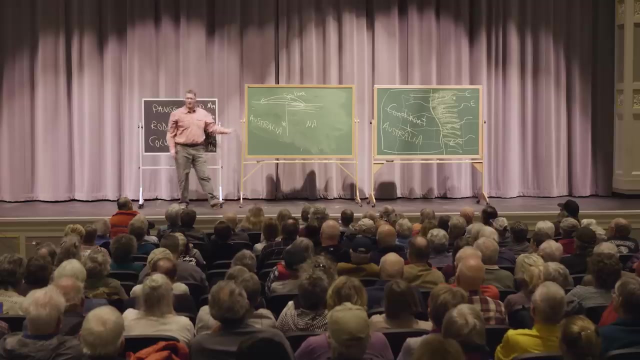 rock in the core of Australia. that's a match. That's a match. age, chemistry, everything else Same thing here. On this sketch, I can do this. It even gets better. There are some grains of ours that went the other way. 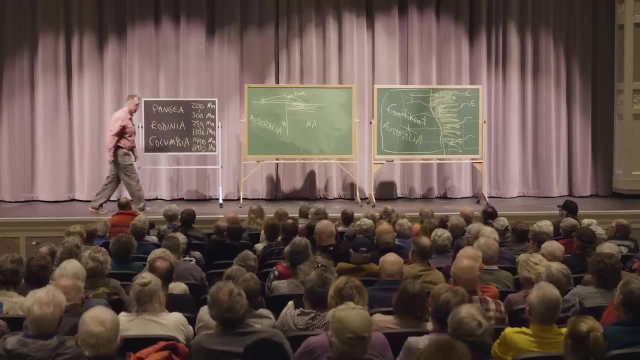 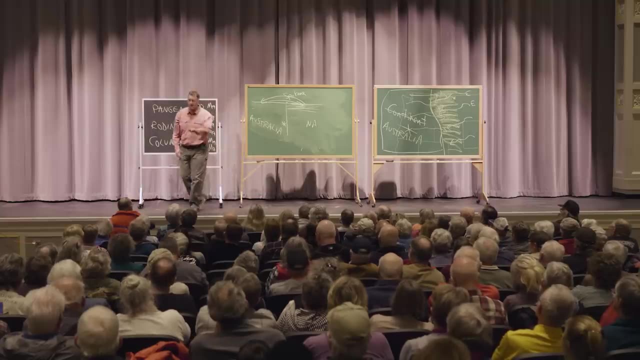 But I have to put an asterisk next to Australia, And here's why A majority. it's 2019, is it not? There's a majority of geologists in 2019 that say it was definitely Australia. I've written my scientific paper and I've got all this evidence to match the Belt and 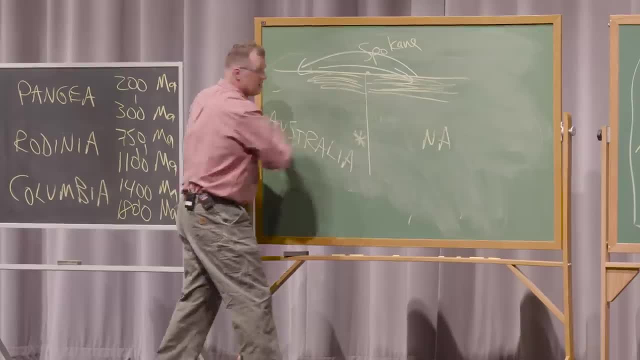 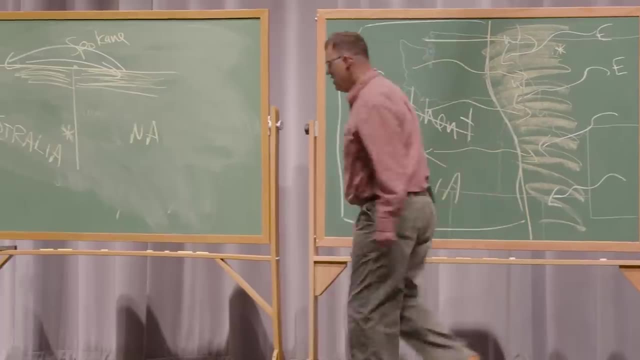 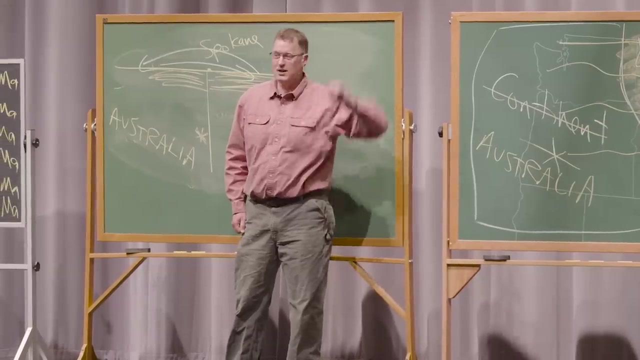 to match the belt of the Pacific Northwest with the belt of Australia and some old craton on North America and Australia as well. But from this point forward in our little lecture I'm going to do this every time I say Australia. okay, This means asterisk, because there are still some holdouts. 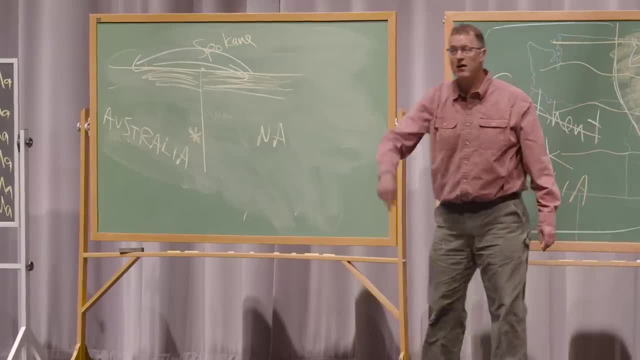 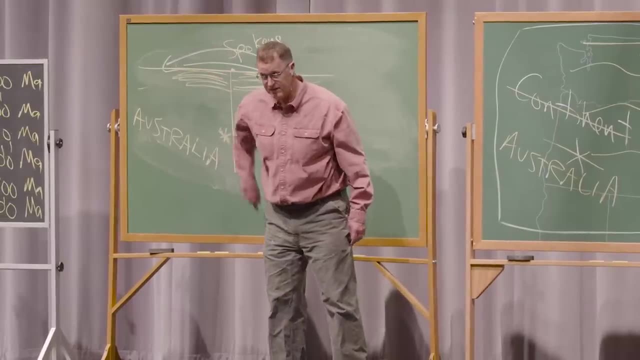 There are still some geologists who say it was not Australia, it was Siberia. Another group says it was not Australia, It was Antarctica- next door parked at John Stockton's house in Spokane. Even another group saying it was not either of those. 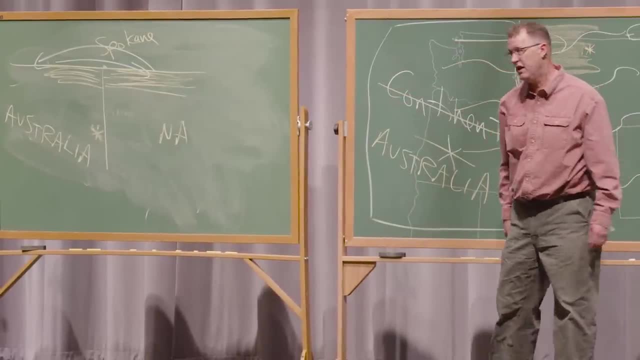 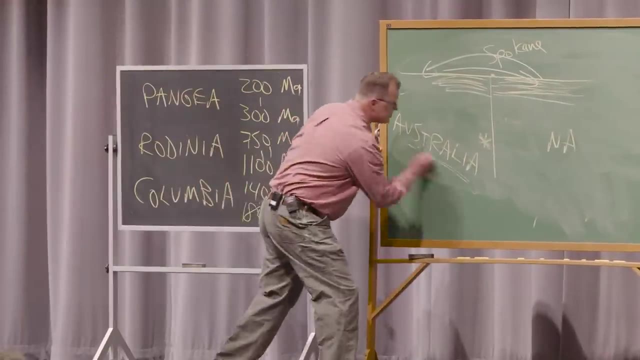 It was a piece of South China pre-Cambrian craton of South China. So there's a chance all four of those are still going to be in the literature for a while, But there's enough people saying Australia and the visuals I'll have showing these world. 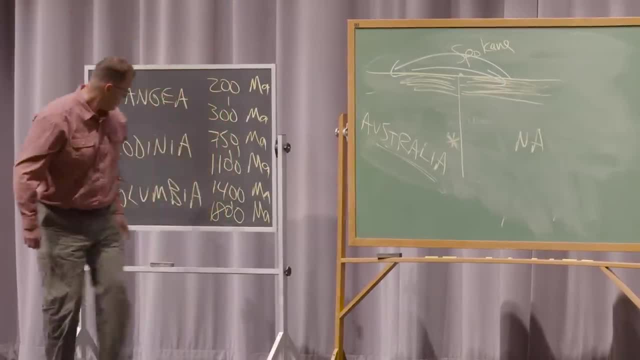 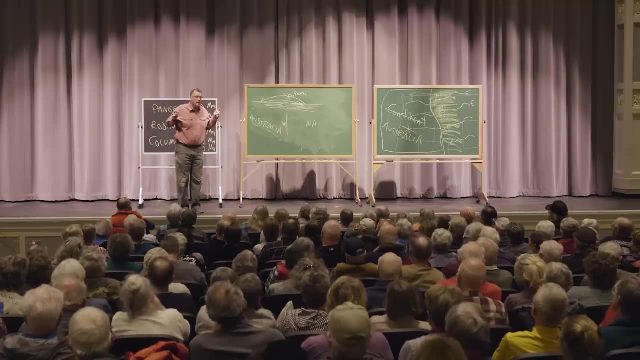 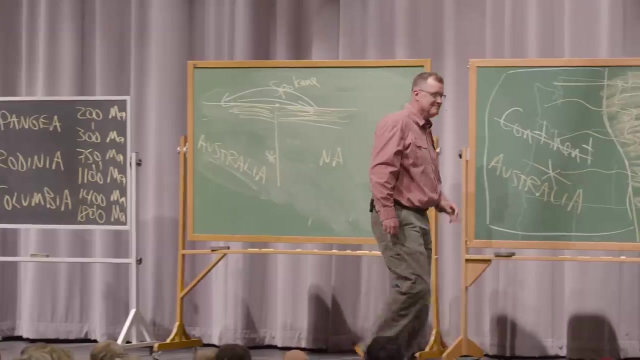 maps. many of them will have Australia next door during supercontinent Colombia. I don't know how you feel, But that was the big moment tonight. Now I'm telling you how to react. That's cheap. So last time I checked, Australia is not here anymore. It took off at some point and we have a date for that For sure. everybody agrees that continent X, most likely Australia, rifted away, began to break away from the Pacific Northwest- Pacific Northwest- 750 million years ago. The evidence for that is something called the Windermere Group. 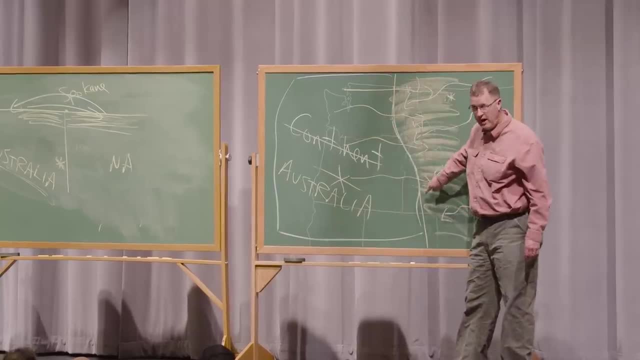 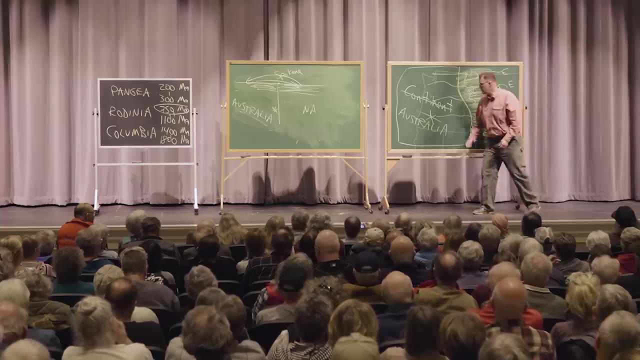 And specifically the evidence for that is there are basalts that start showing up, Basalts that have now been metamorphosed into rocks called green stones, But they were originally basalts. And anytime you have a continent rifting away from another continent like North America, 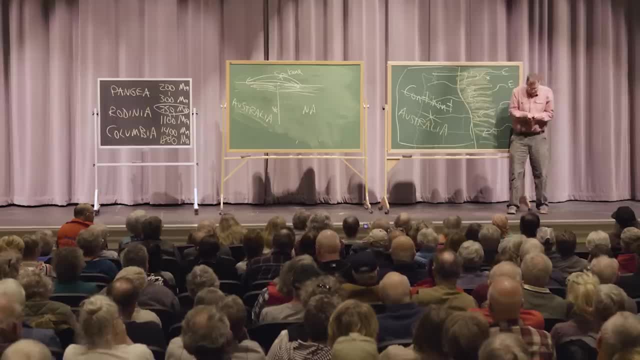 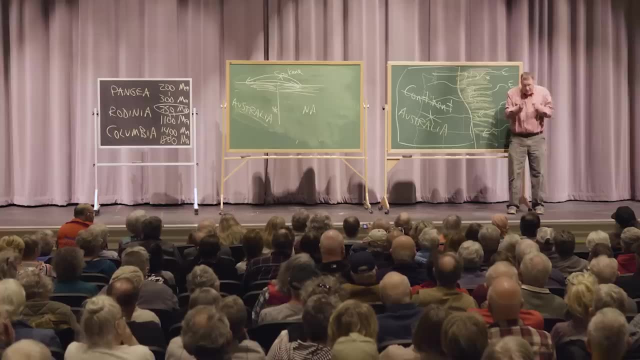 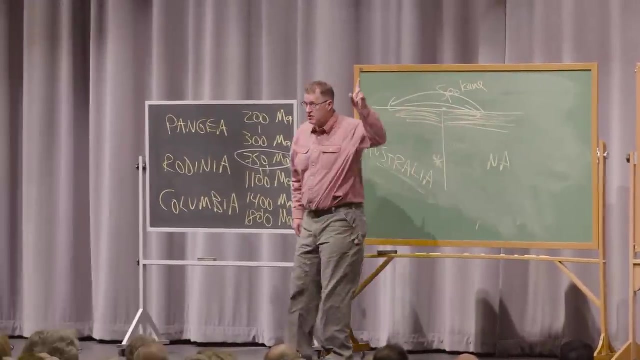 rifting away from Africa during Pangea's breakup. you develop ocean crust in between those rifting continents. You create ocean crust, Ocean crust in between these rifting continents. So the basalts- now green stones- of the Windermere Group is the basalt that formed as Australia. 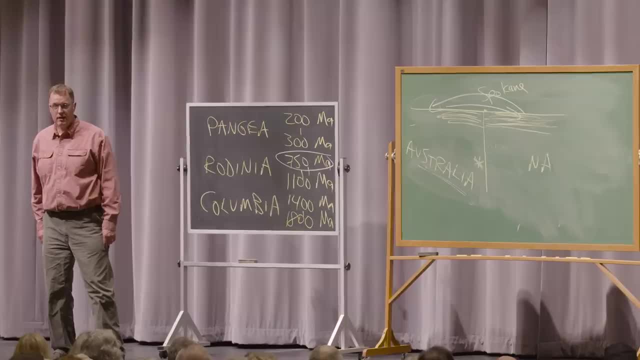 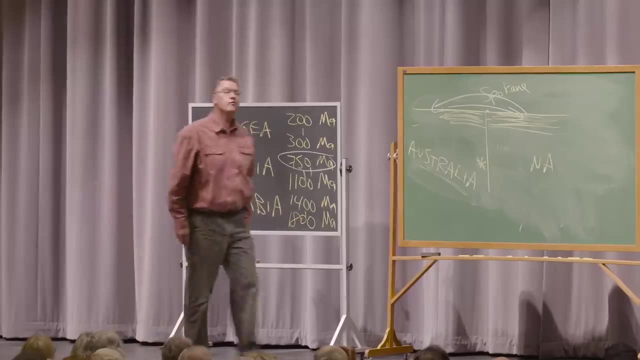 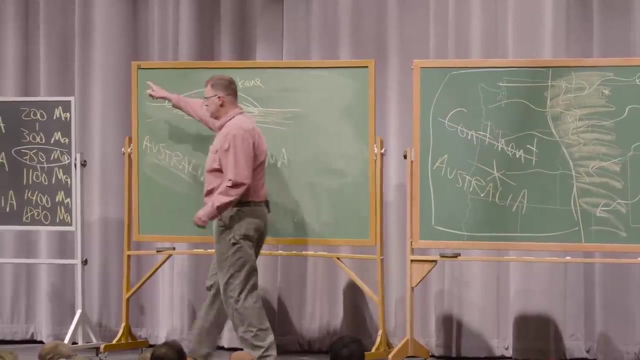 rifted away from old North America, Never to come back, Or will it? Will we reconvene and be reunited with Australia at some point in the future, in the next super continent to come? The last thing I want to do is very quickly on the chalkboard and then we will switch. 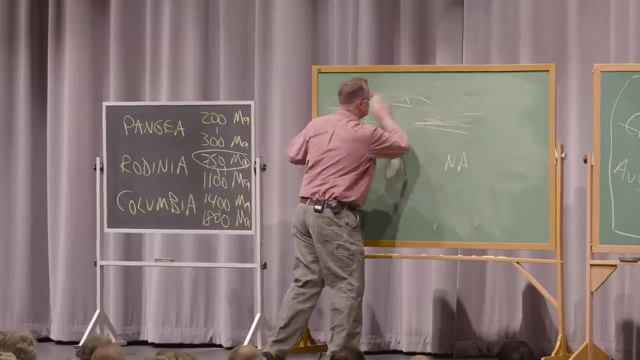 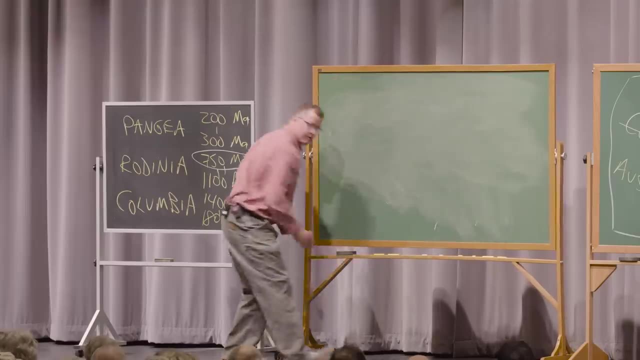 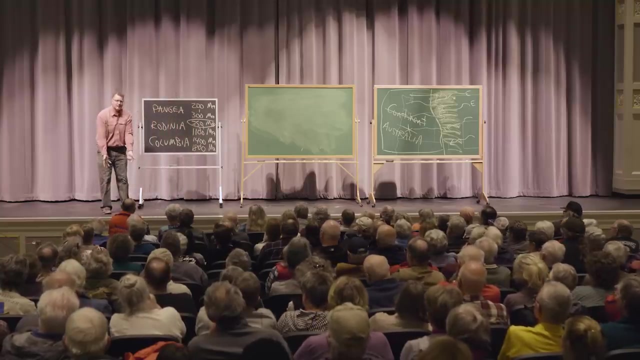 to the visuals, because I've got lots of good stuff for you there. Australia is gone, But I feel we need to make Washington. If this is a lecture in Ellensburg, Washington, in the Morgan Auditorium, we got to make this. 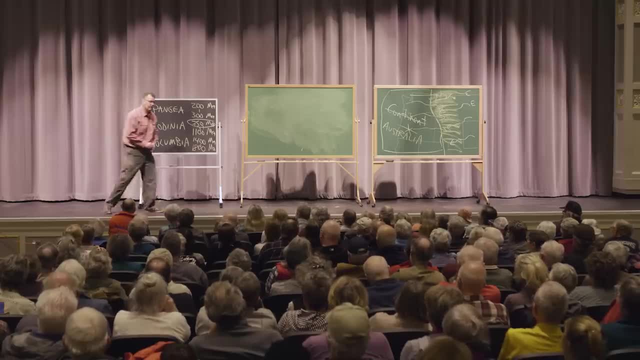 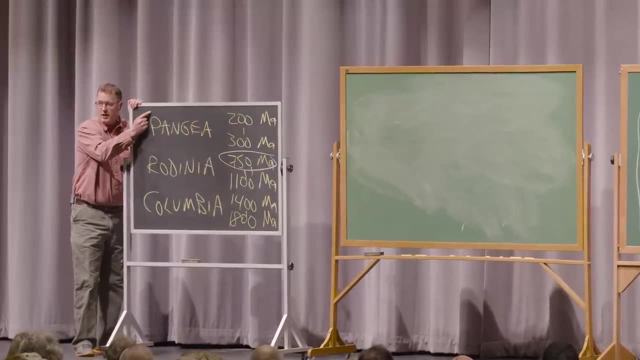 state. somehow, don't we? We can't just leave deep ocean here. At least I don't think we can. And so if we jump way up here To the breakup of Pangea- And North America is starting to move west as Pangea breaks apart- 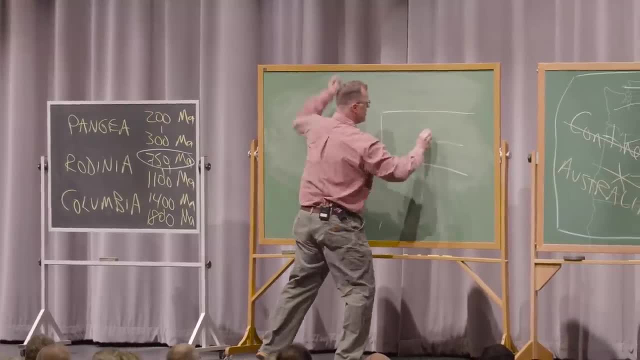 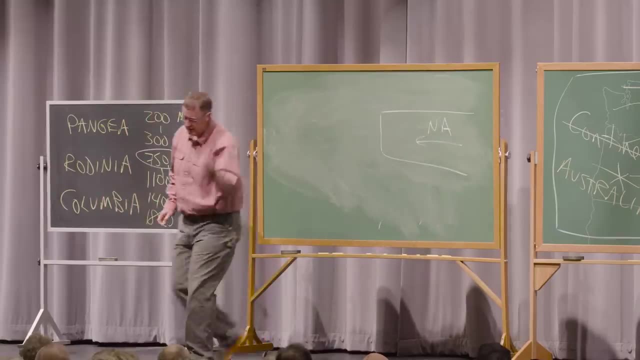 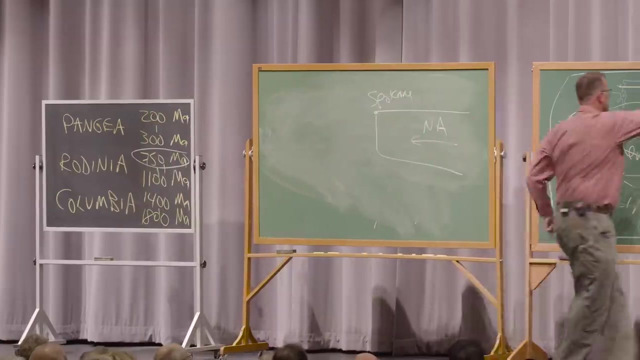 Let's do that. North America is moving west with the breakup of Pangea, So there goes Africa heading out the other way. And if this is new to you, you'll see some maps. What city is here? Spokane? This line is clearly where Australia rifted away. 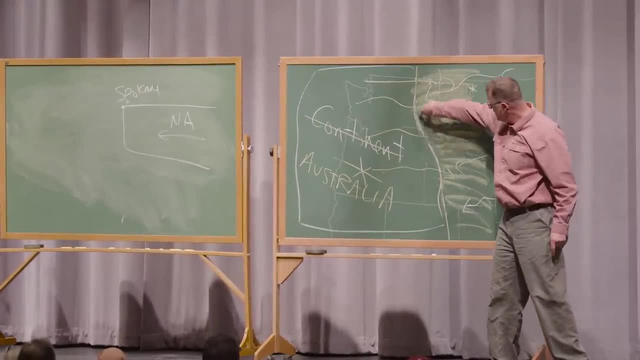 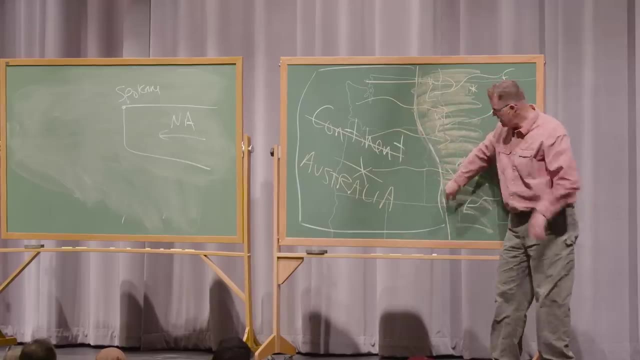 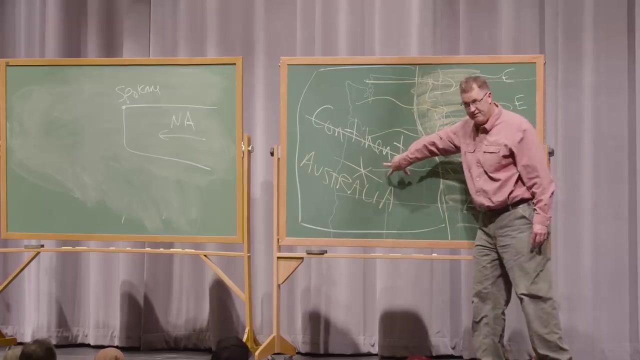 Australia And that old rift has been there for a long time. It's a very sharp boundary. Geologists call it the strontium 706 line, simply meaning that there's certain chemical signatures in the magmas coming up through this craton material and very different chemistries. 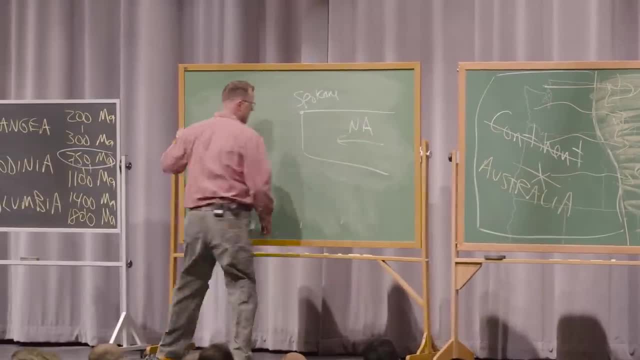 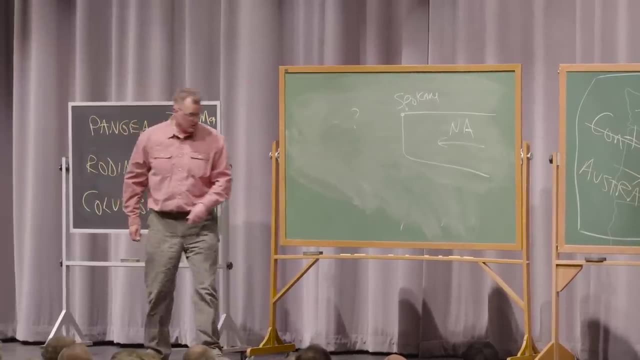 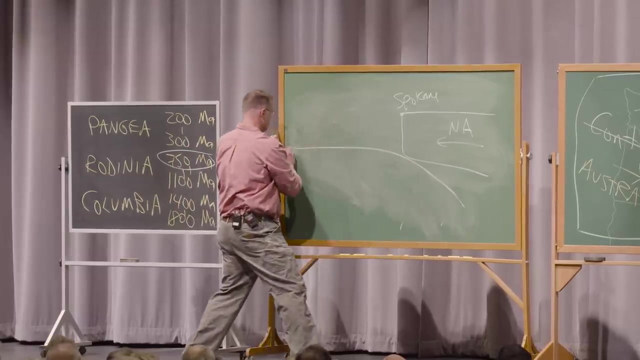 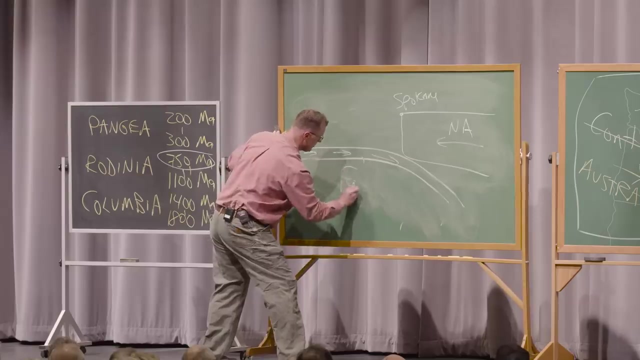 strontium, differences, with the magmas coming up in this other stuff. So how are we going to build Washington in the last 200 million years? Many of you know this. Last year We were on exotic terrains, But I want to revisit the main concept, which is we had a huge ocean plate called the Farallon. 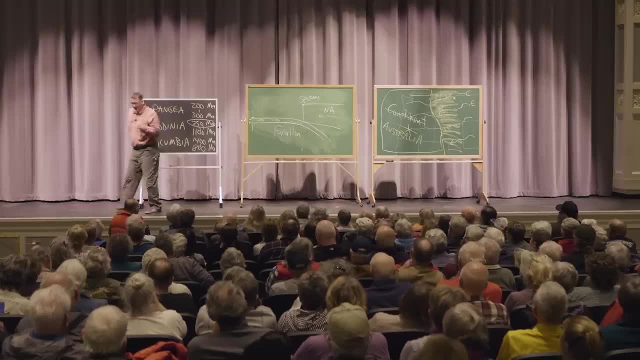 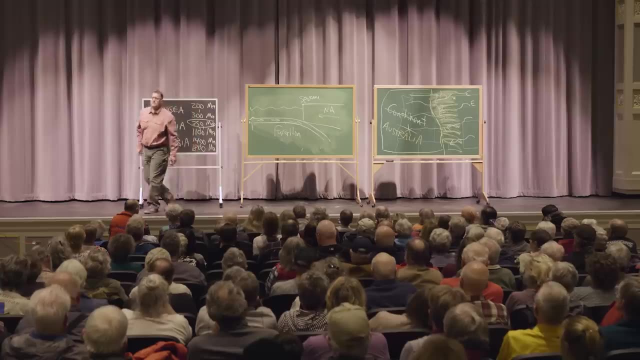 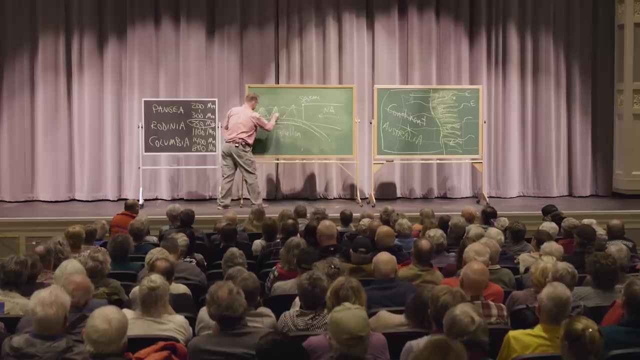 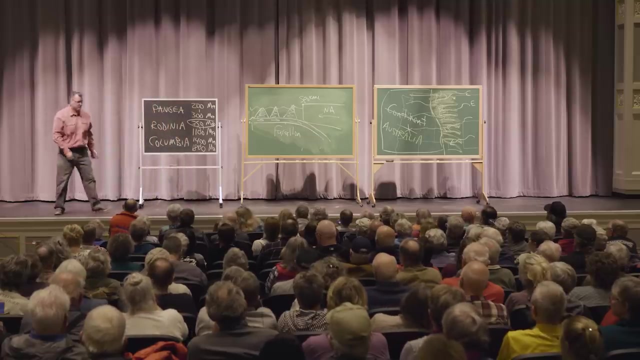 Plate that was coming at us and subducting beneath us. This is ocean now And we make Washington by receiving gifts From the ocean, From the Farallon Plate: Huge gumdrops, Huge exotic terrains of different origins that are riding on this conveyor belt. 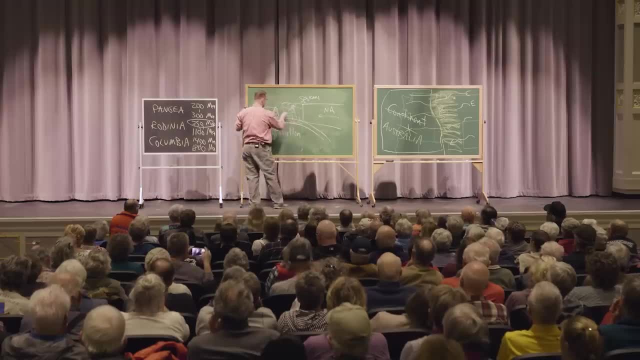 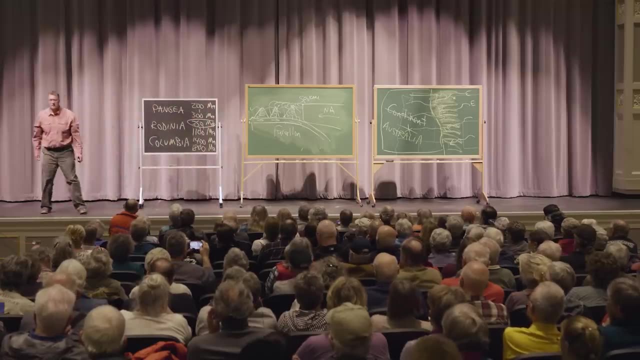 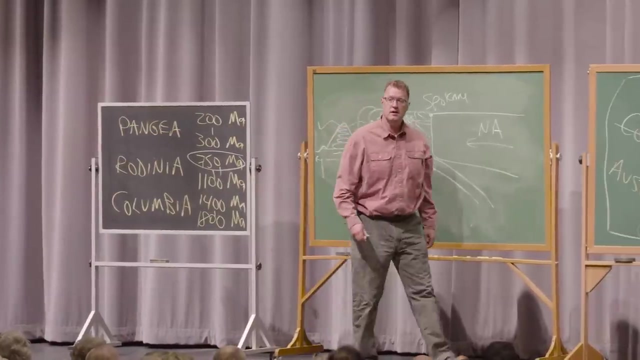 And as the Farallon Plate continues to come at us, we build Washington piece by piece And eventually we build the entire state of Washington. The last terrain to come in made the Olympic Peninsula, And we'll have a couple visions. We will 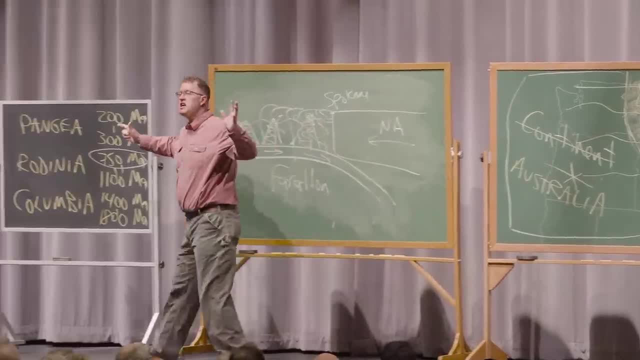 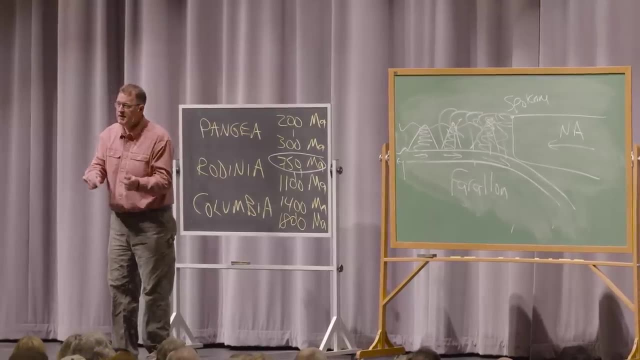 This is a big room. now I can't talk one-on-one with you, Right? So there's a whole scene, There's a whole drama just in the last 200 million years, But this lecture is predating everything we've done in this series. 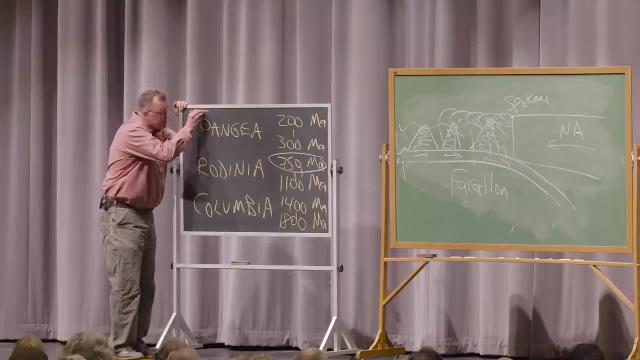 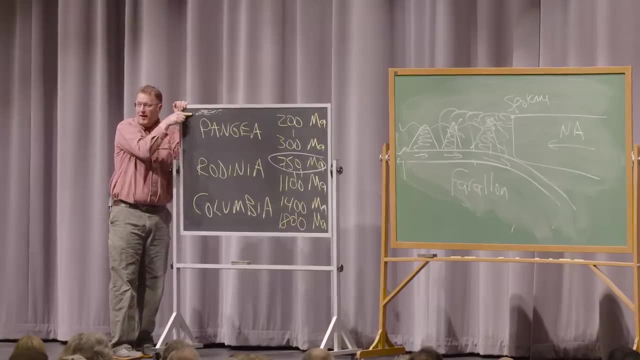 Everything we're talking about here: The Ice Age, floods, The flood, basalts, The Cascades, The Bridge of the Gods, landslide, Everything. It's all right up here. This is the first lecture. We're brave enough to go this far. 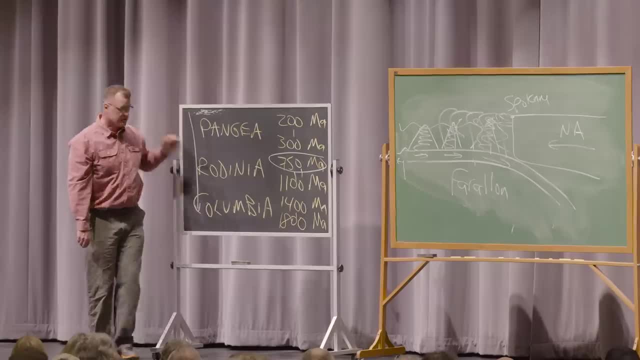 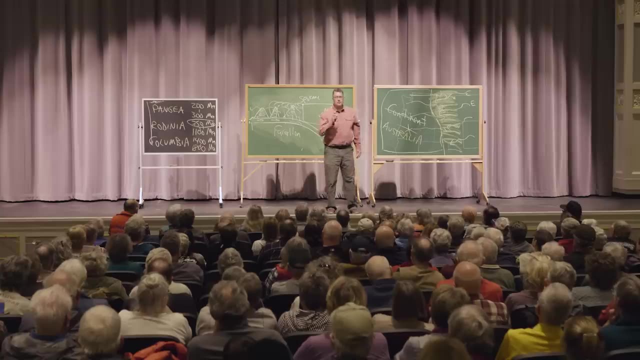 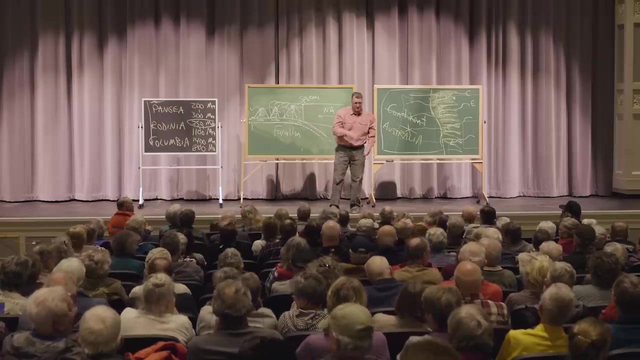 We're brave enough to go this far back in our history And certainly there will be new data coming about, those old supercontinents. This is the moment to say to your neighbor: isn't this interesting? I love this. And while you say that, we're going to get the screen going and the projector 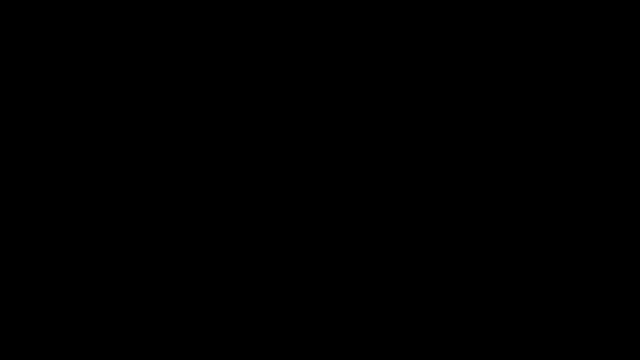 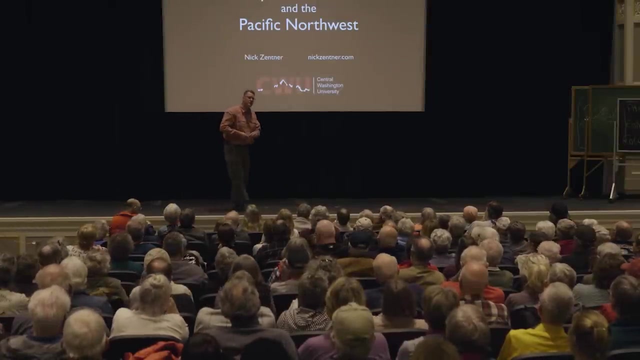 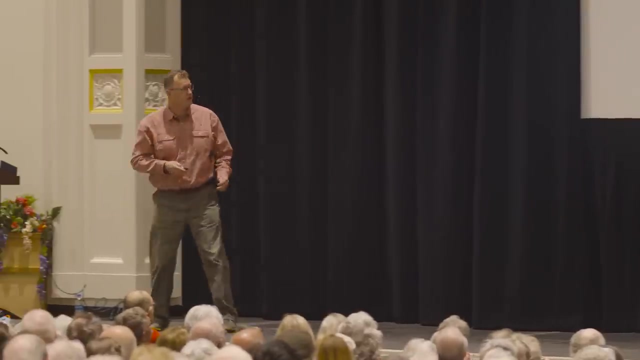 Okay, Give us just a second. Thank you. Okay. The chalkboards do a decent job, but I think we need more. I think we need more professional imagery And some animations and a few other things to make this work. So let's go ahead and take some photos, et cetera. 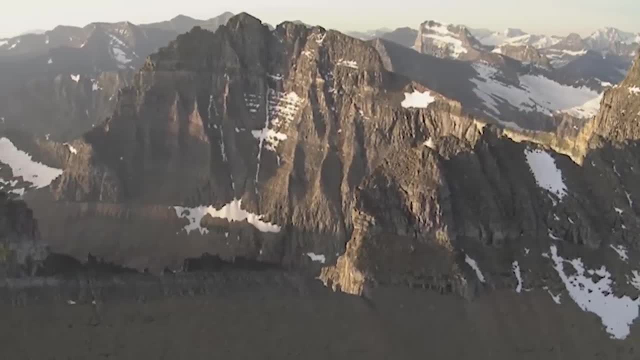 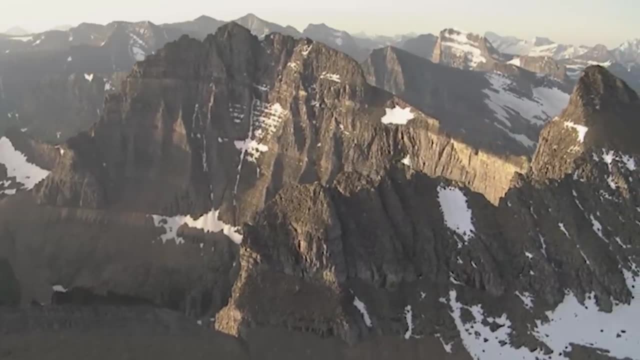 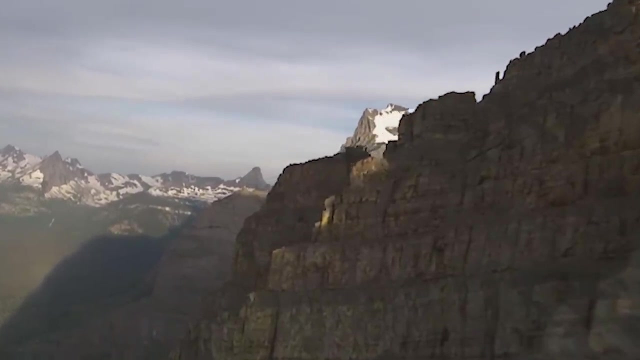 We've got some really wonderful footage of Glacier National Park. You can see the layering of the bedrock here. That's the belt. These are the beach rocks between 1500 and 1400 million years. The glaciers themselves have dug so well recently to reveal all these cliffs, otherwise we wouldn't. 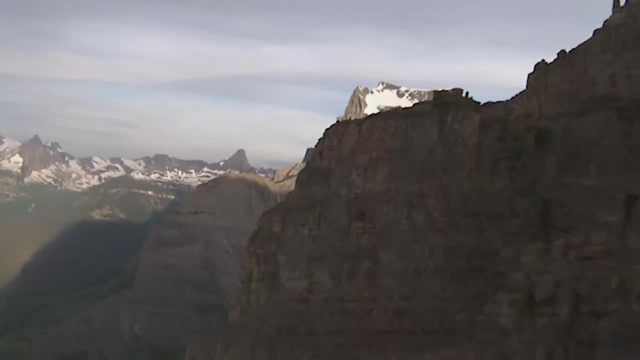 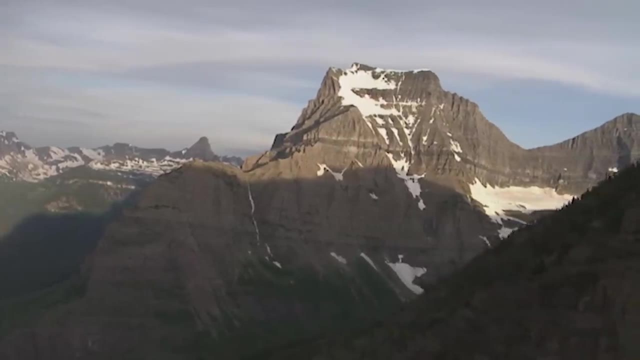 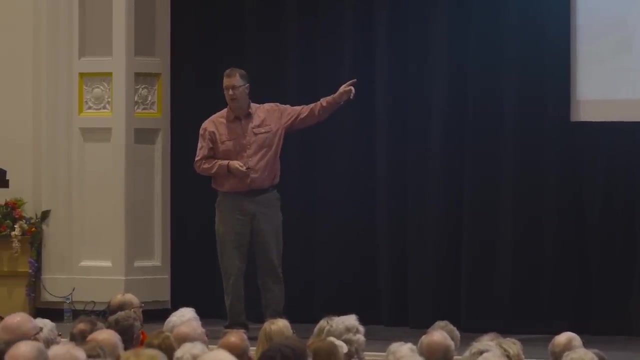 see many of these rock layers, But this is the place that it's quite easy to be introduced to the belt series. They're right there in front of your face. They're on every hike that you do in Glacier National Park- Coastal rocks. and are you looking at this in a different way now? 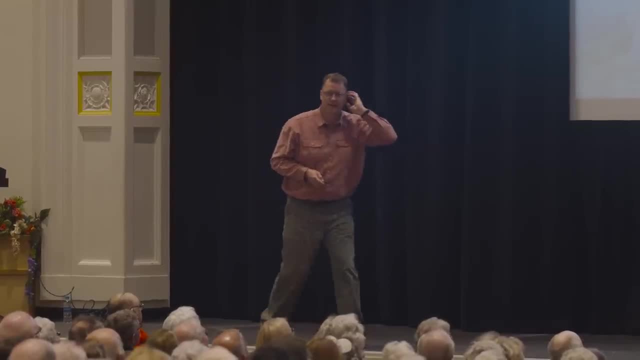 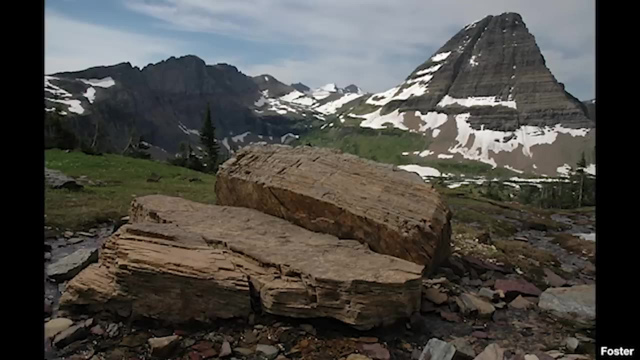 Oh my God, there's grains from Australia in the picture. Now let's zero in on some of the structures that are in the shales and the sands that are now metamorphic rocks. Just think about it: These are the rocks that are in these salt shales. 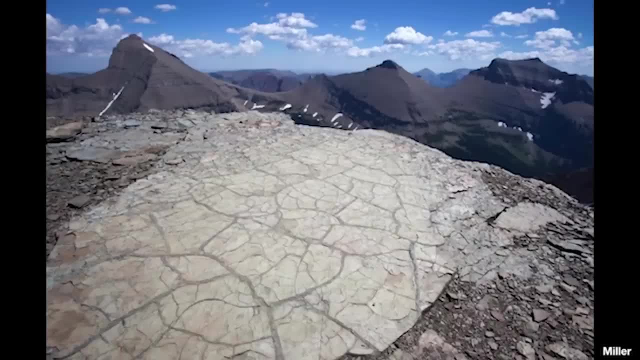 These are the rocks that are in the sand. Now what we're trying to do is we're trying to come up with a way to determine these rocks and to convince ourselves that this beach story really is true. Look at this. These are mud cracks in a tidal mud flat from more than 1400 million years ago. 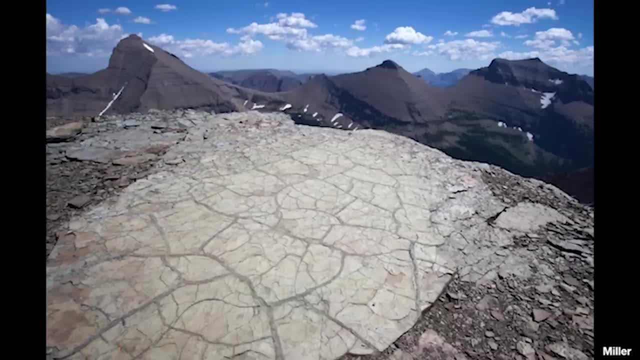 Isn't that unbelievable. This is so far back in time. we have no major fossils to bioturbate to screw up all these very delicate features. So the amount of preservation in these rocks that are more than a billion years old, when these rocks are so high up on the surface of the earth, what's it going to do for us? 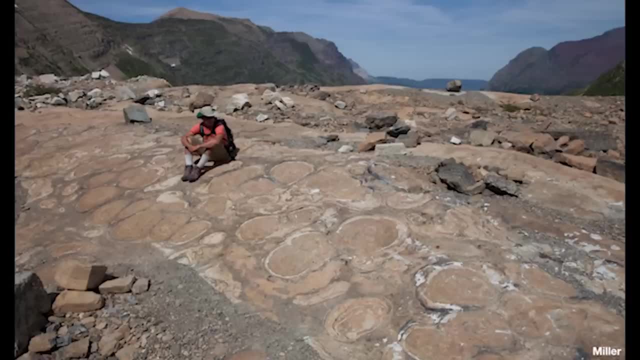 It's going to be very hard to determine them- is absolutely staggering. These are the stromatolites. We're still in Glacier National Park now. These big mounds of blue-green algae- Think the Great Barrier Reef off the coast of Australia, if you like. 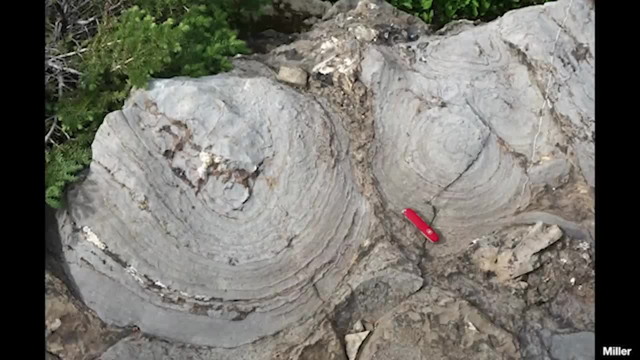 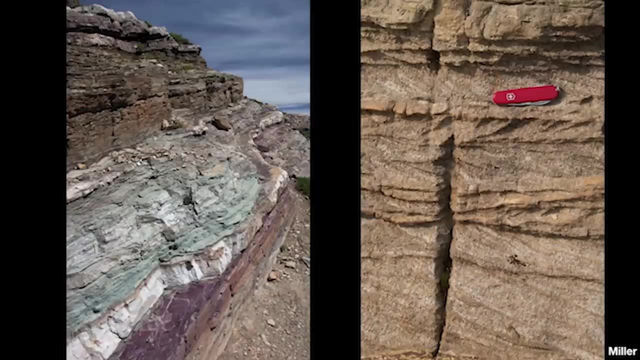 Oh, that's ironic. Off the coast of Australia It's so rare to see fossilized mounds of algae number one, but to find them in this old setting is truly outstanding. Now, the picture on the right is the best I have for you. 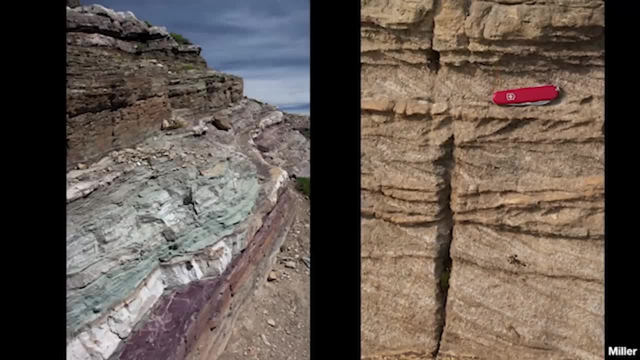 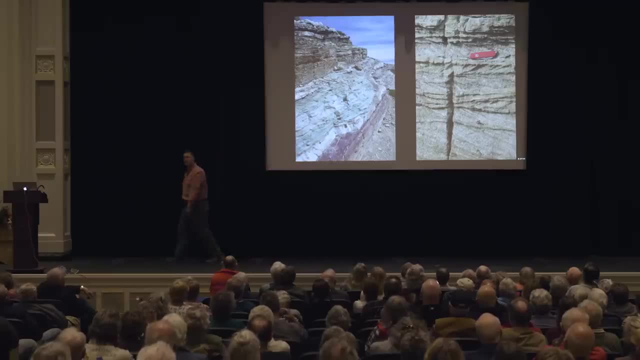 to show some of these current indicators. Can you see? there's kind of some Nike swooshes in some of this stuff. So geologists can study the arrangement of the sand grains and say something about the direction that the river was flowing. And here are the uncomfortable rocks to sit on. 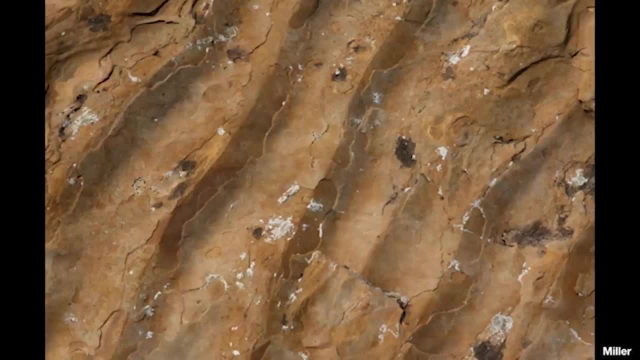 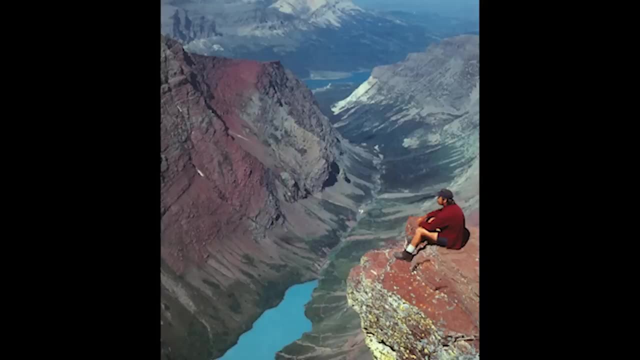 the ones that have these symmetrical ripples in the slate that used to be mud. So these maroons and these greens and these purples- if you've been to Glacier Park, you know exactly what I'm talking about. And those are the rocks. 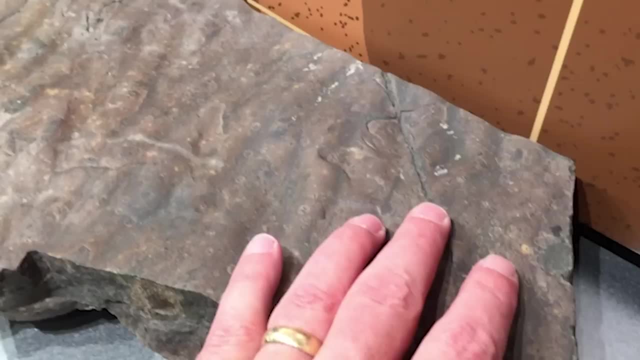 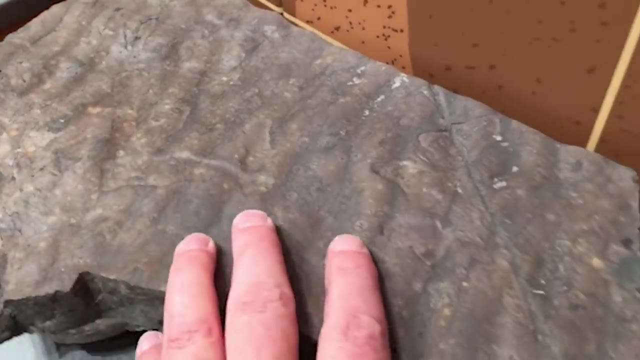 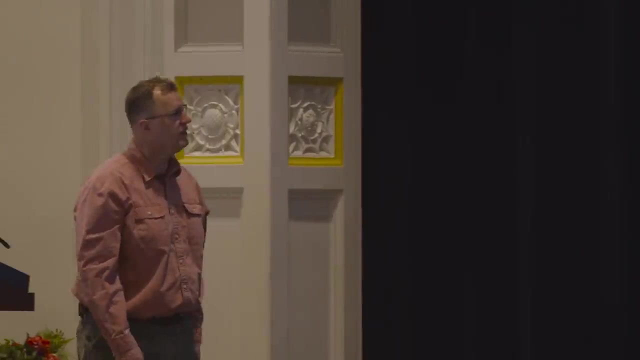 that we're featuring tonight from supercontinent Colombia. This is a slab that's on display in our geology building here in town, And just running your hands over those ripples is like being at the beach 1,500 million years ago. Now let's leave the high country. 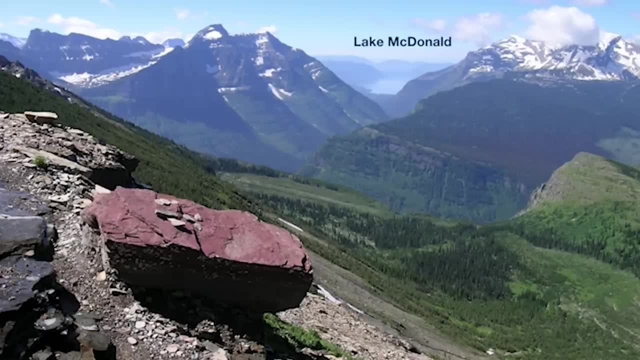 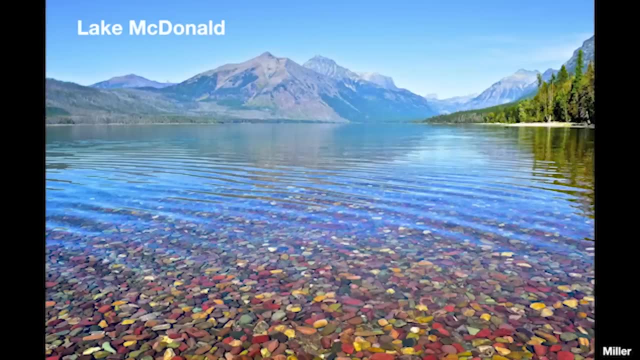 where the belt is best exposed, the belt series. and let's go down to Lake McDonald. Lake McDonald, famous for its beautiful, brightly colored rocks in the bottom of the lake. We know those rocks. now Those are broken off pieces of the beach belt series. 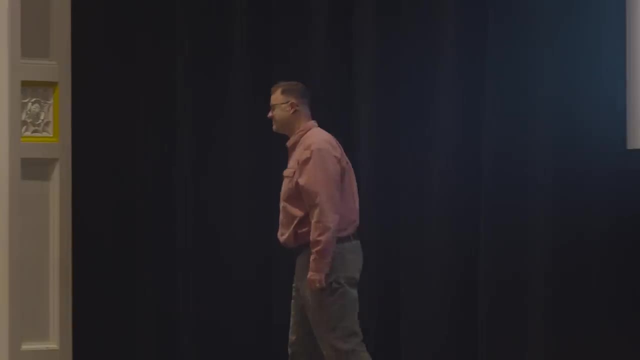 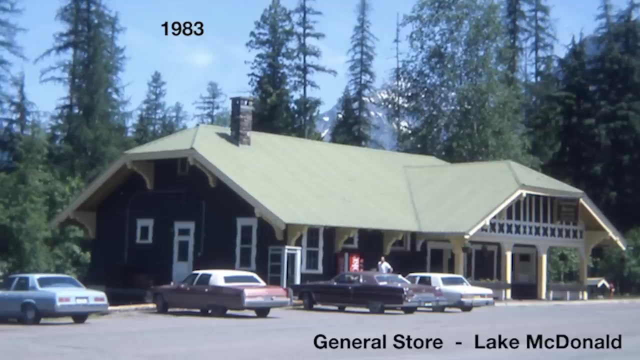 Oh, but we're going into the archives And there's the general store. It still pretty much looks like this. Look at the size of these cars, by the way, in 1980. And the huge Coke machine. So I'd be walking back and forth. 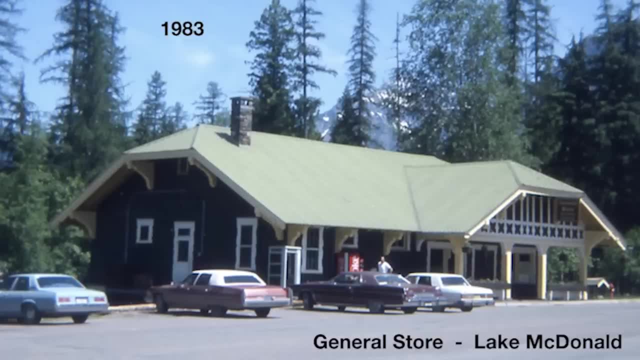 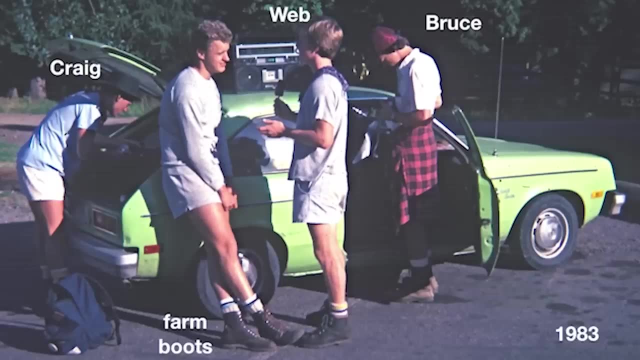 When a car would pull up to the pump, I'd walk out and pump their gas and then go back and sell rubber tomahawks and all sorts of stuff. And this is the morning of that hike that I was telling you about, The very morning of our group of four. 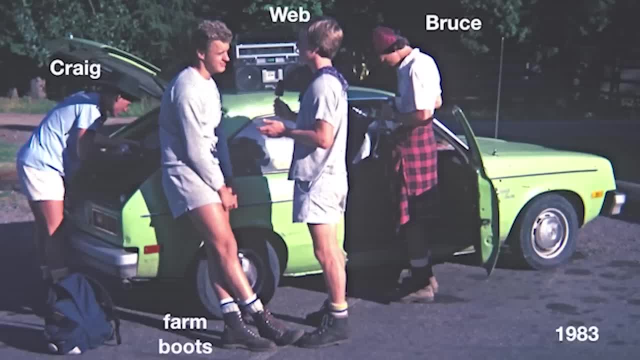 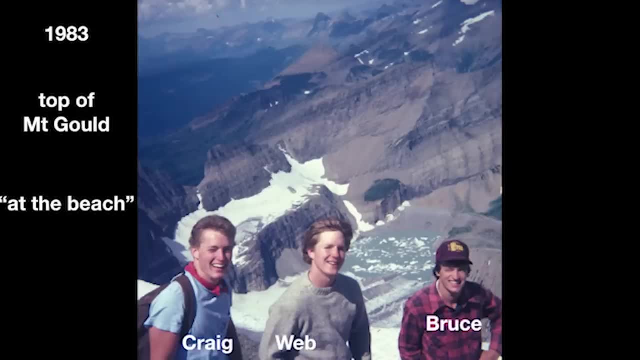 heading up to Mount Gould. Craig was the leader. Craig was the guy telling me about the beach up on top And after our beach conversation I took the photo here because I had a frown on my face. probably I still didn't understand. 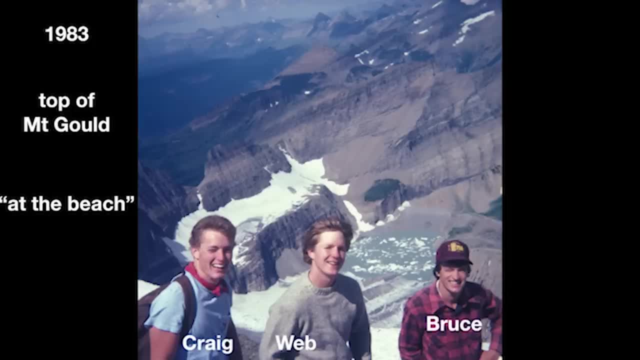 why there was a beach in the mountains. But you can see how high we were And can you imagine the effect of a summer like this from a kid from the farm in Wisconsin Had never experienced anything like it. I still have the book that I read the rest of the summer. 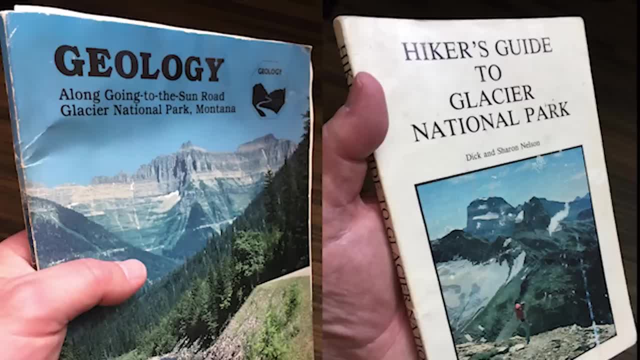 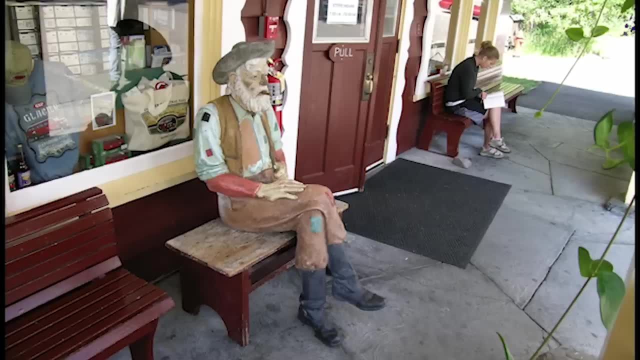 that we sold. I never bought it, I just kind of borrowed it And I would read and reread that geology of the going to the sun highway out in front. So when I took a break from working in the store I'd come out here. 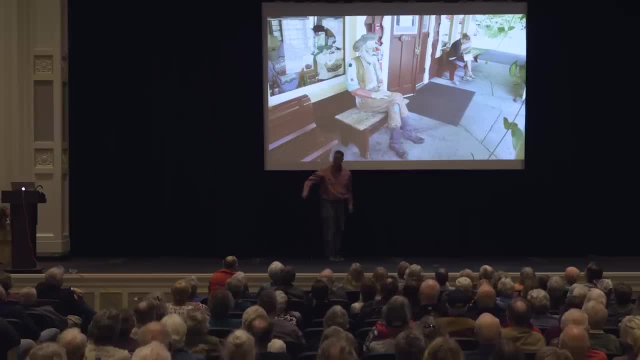 and sit in front and I'd reread that one little geology book. I've got it right up here on the stage And one of my jobs with a co-worker was to bring this statue out every morning and then bring them back in. 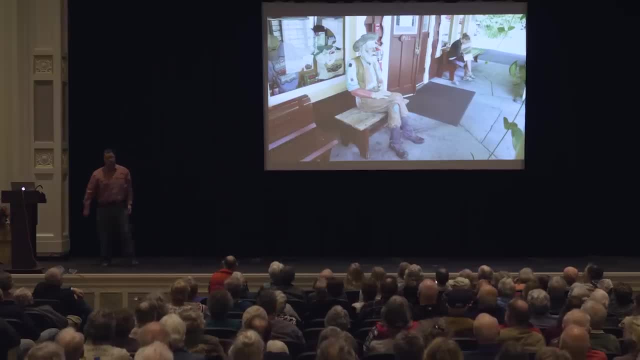 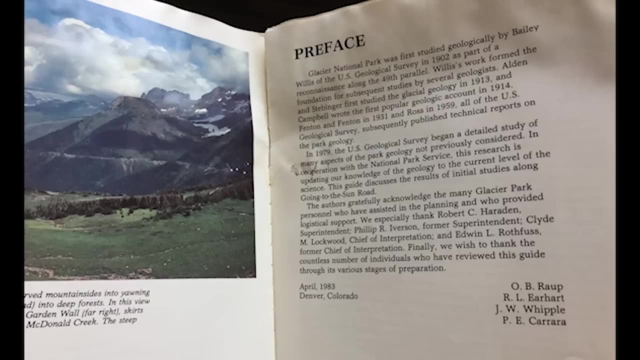 so nobody would rip it off, And I hope that guy's still there with his cigar. He was the last time I visited in 2010.. So this book written in 1983, just a few months before I worked there- was the reason. 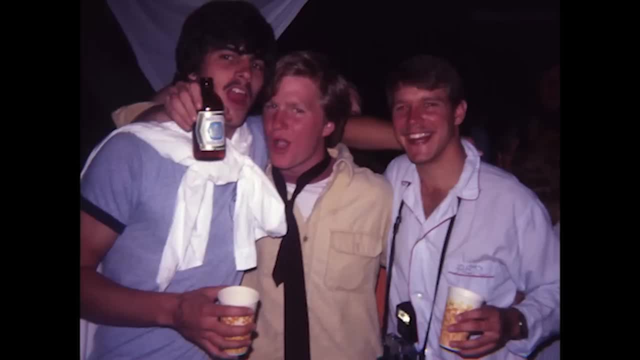 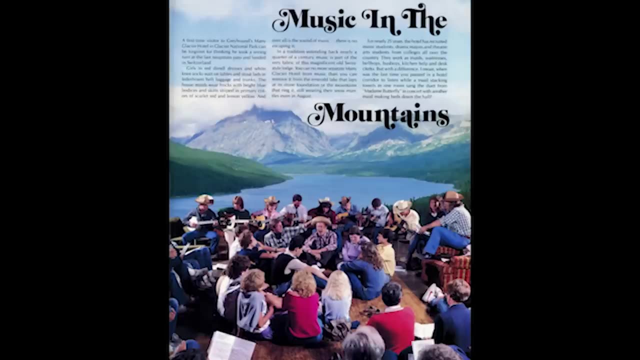 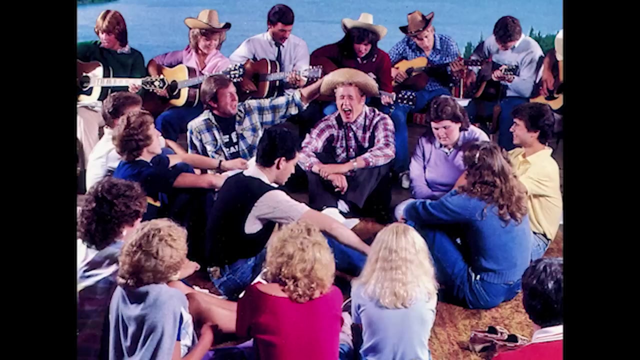 that I got into geology. There were other things to learn that summer- We don't need to go into that. Kids from all over the country And many of us working in Glacier Park had music backgrounds, And so somehow I got to be the little master of ceremonies. 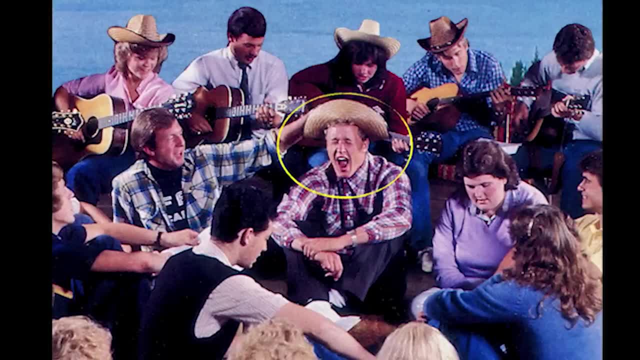 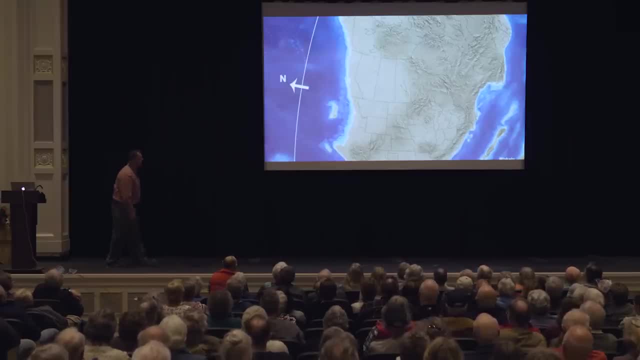 like serenading the lodge people. So every Wednesday night we'd have this little group sing, along with the guitars and everything. Okay, back to the geology. So look carefully at this map. We've got Idaho and Montana, but we've got the old coastline. 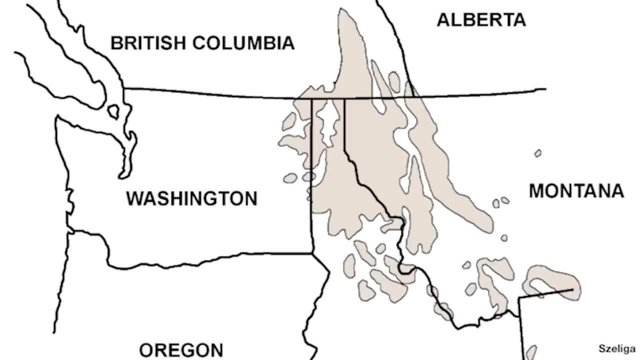 that the belt is telling us about, that the belt rocks are telling us about, And here is a more specific map showing the exact locations of where we can find belt rocks. Notice, we are getting into northeastern Washington. Spokane is about here, right. 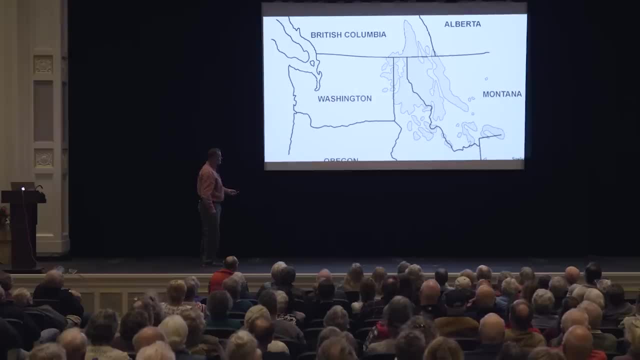 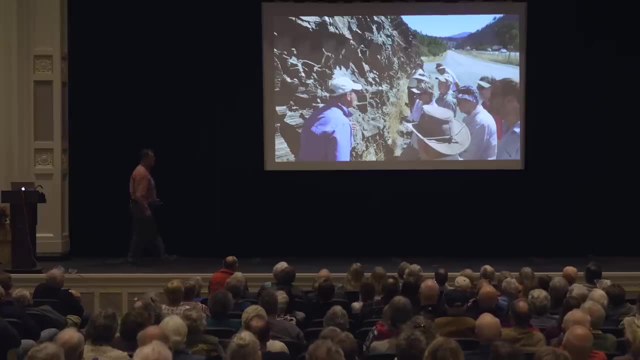 So we've got the corner of our state and all the way down even into the Lemhi Mountains of central Idaho have many of these grains that have been studied very carefully by Paul Link and others. I went on a field trip a couple of summers ago. 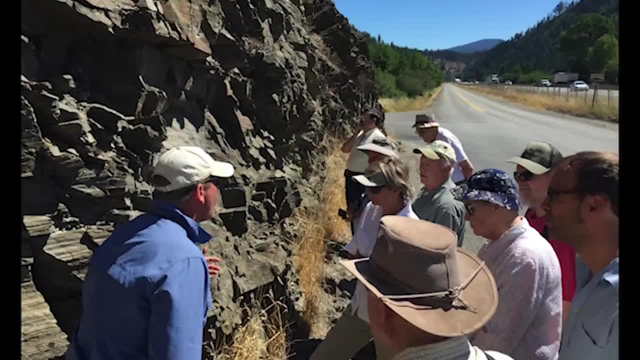 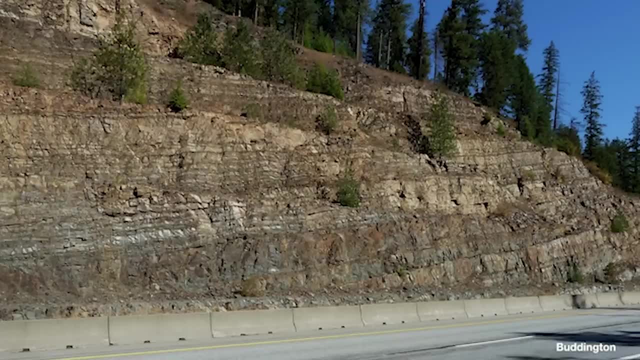 just along Interstate 90 near Coeur d'Alene, and Andy Buddington here is in the blue shirt, And many of these photos are from Andy Buddington, who teaches geology at Spokane Community College. Andy was a great help in putting this lecture together. 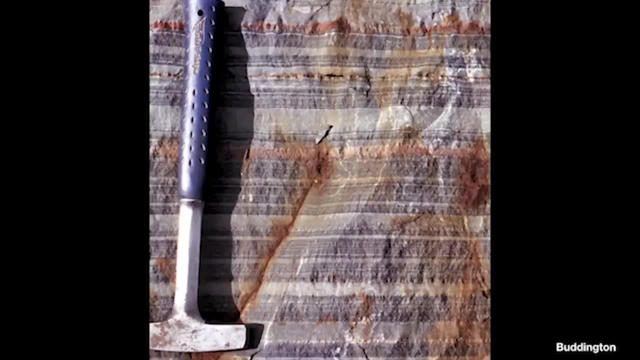 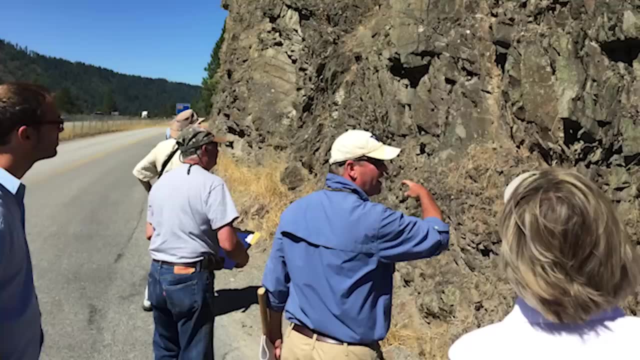 He has studied the belt academically. He worked in the silver mines right out of school as a geologist and so he knows the Wallace area quite well, And so there's a tie with ore as well and the belt. But anyway, this is just the frontage road. 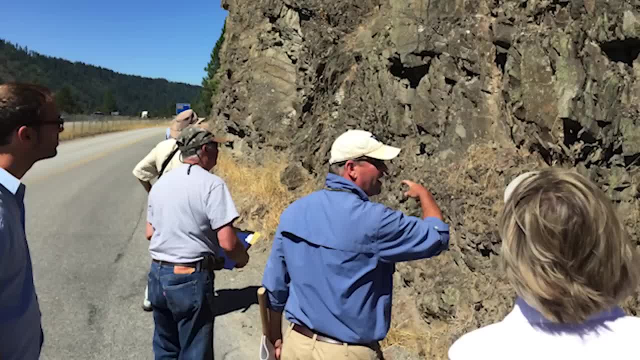 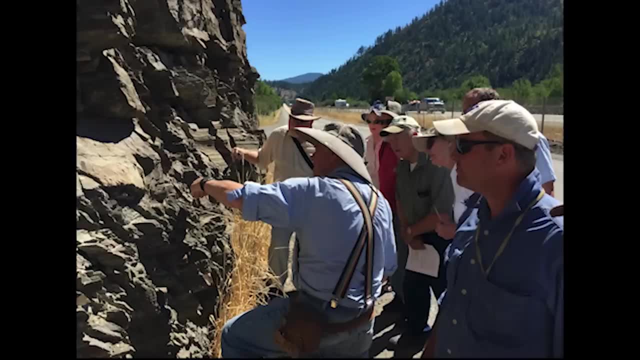 This is the old road right next to I-90, basically by the best stakes in the world at Wolf. what is that? Wolf Creek Inn or something like that? Amazing, amazing place. Here's Eric Cheney from the University of Washington leading us on a small geology group. 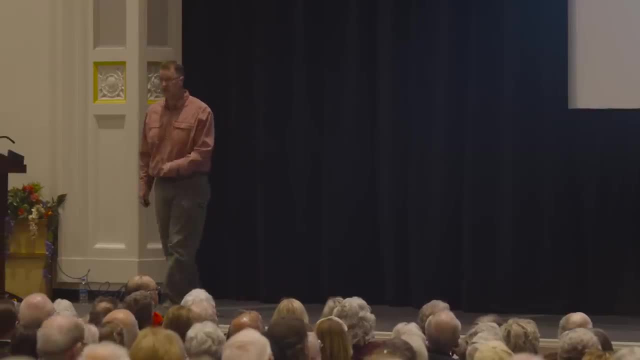 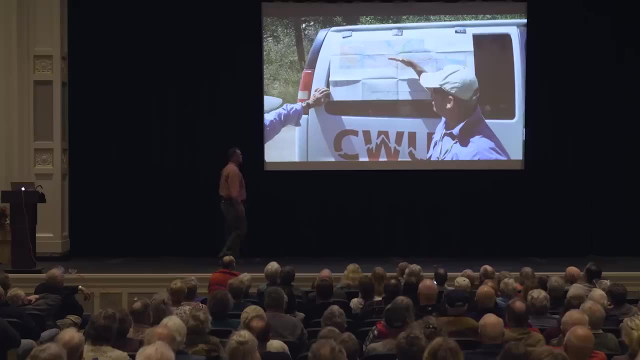 And they kept talking about Rodinia and I didn't know what they were talking about two years ago and the breakup of Rodinia. Now we know how Rodinia and supercontinent Columbia fit into this story. So these, if you're a geologist in the room. 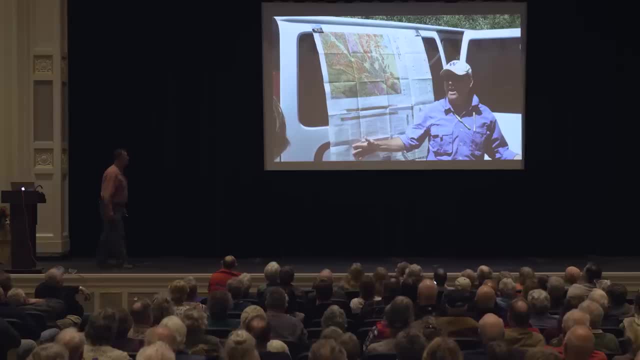 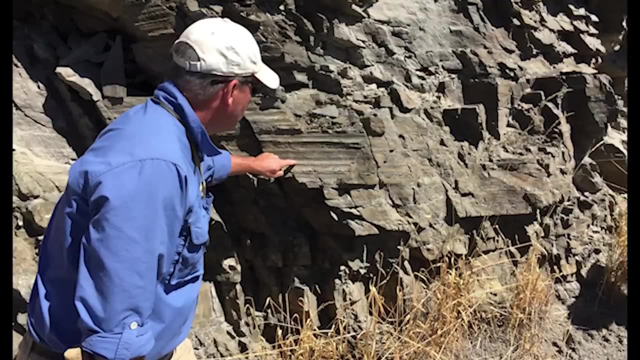 these are all familiar looking photos. You go out, you stop, you put up a map on the side of the van and you talk, and you talk, and then you go point at some more rocks. These are all the belt rocks that we were featuring tonight. 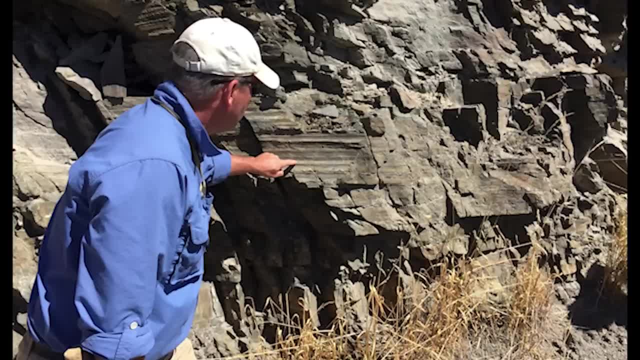 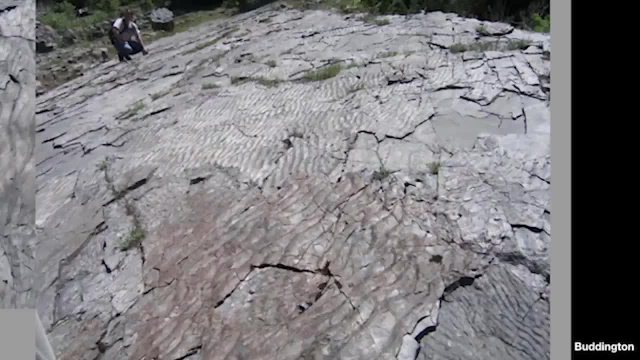 So it's the same rocks that we saw in Glacier Park, but right along the freeway Right there available, Easy to stop and look at if you're very interested. More photos from Andy. Now we're into northeast Washington and northern Idaho. We see more of the ripples. 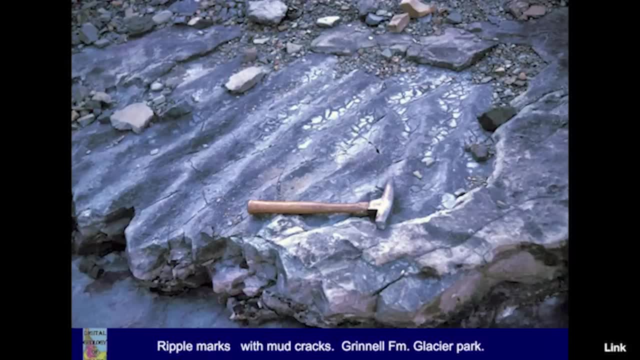 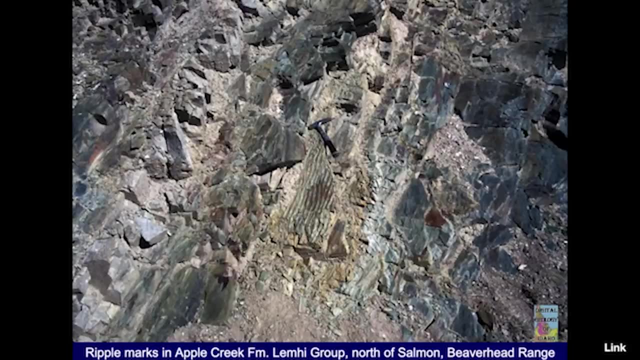 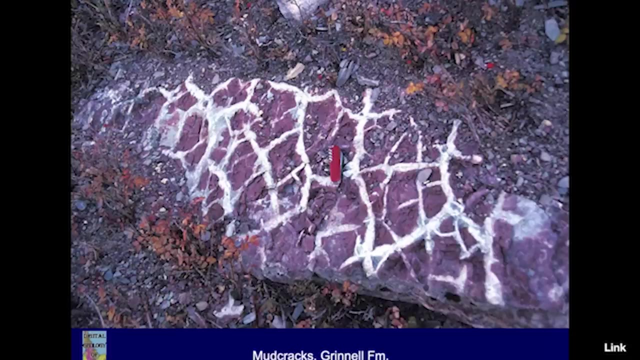 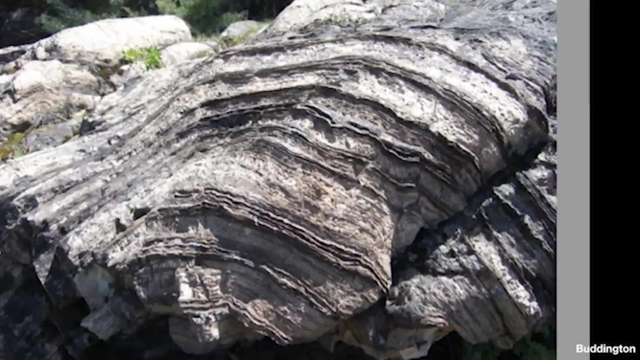 We see more of the petrified ripples. Look, Look at how fresh they look even though they're so old. Mud cracks have different looks. Some of them are truly cracks. Some of the cracks have been filled with replacement minerals and the stromatolites are found in other places. 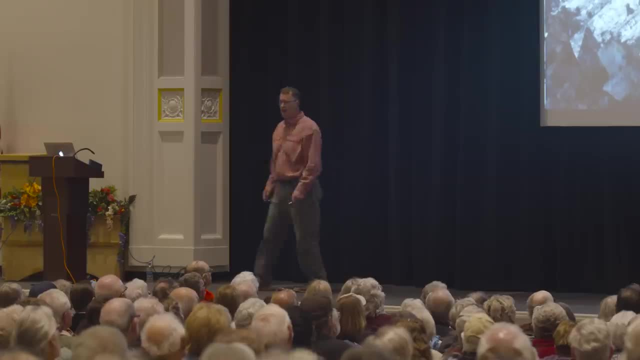 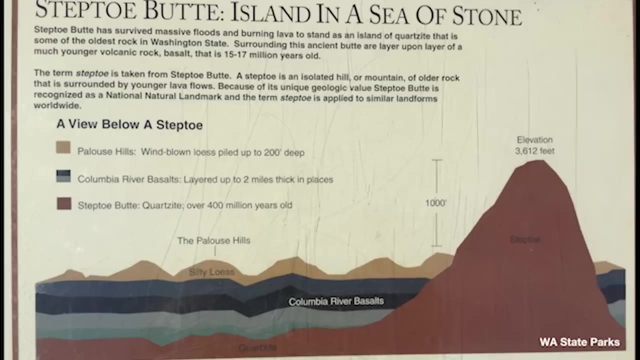 in the belt besides Glacier Park. You've got the point now. We're finding these features, We're finding this consistency. It's a consistent beach story for a long time, Even Steptoe Butte, which many of us know as a landmark. 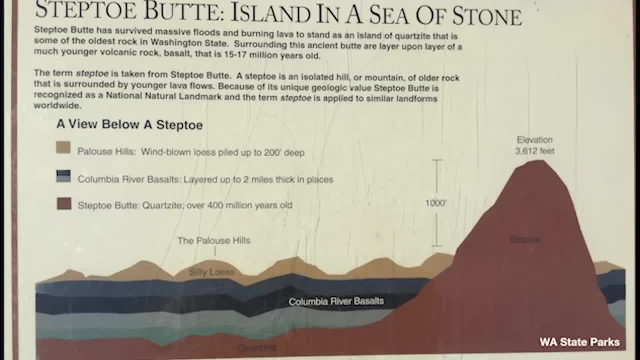 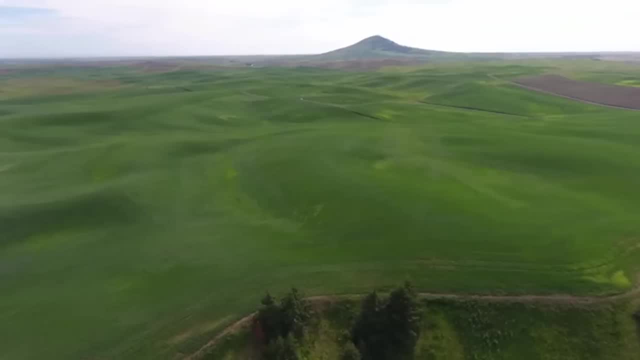 south of Spokane and north of Pullman is made out of quartzite. It's part of the belt. It's an island of belts surrounding by the more famous geology of the Palouse. So our eyes are drawn to the Ice Age Palouse. 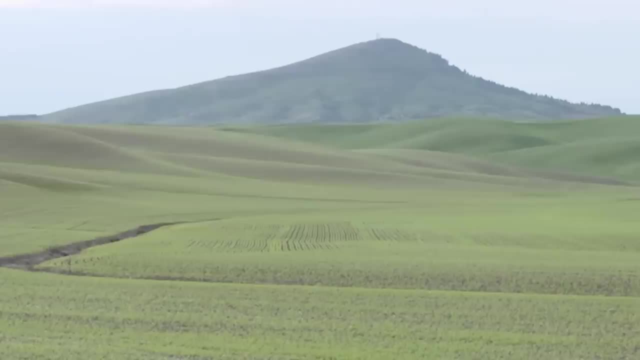 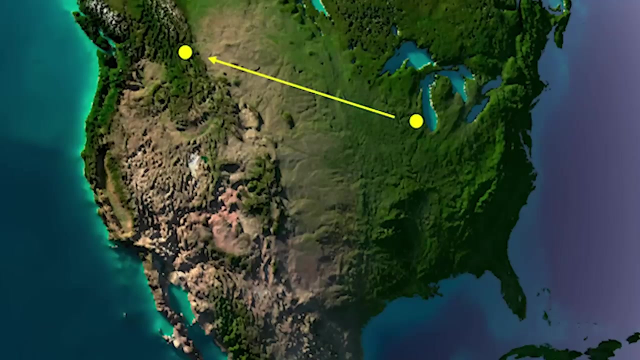 and the flood basalts that are beneath the rolling hills, But the island itself, the mountain itself is from the beach time, From pre-Cambrian days. So not to talk too much about myself tonight, but when I finally went back to Wisconsin, 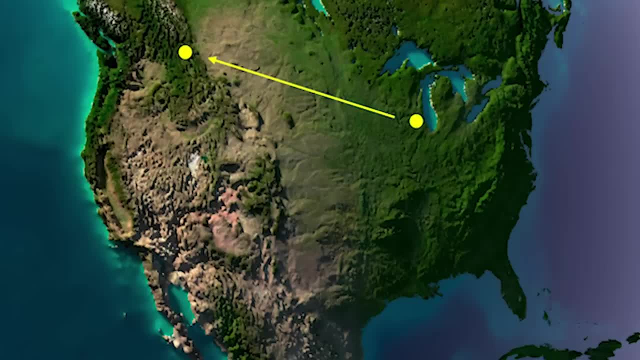 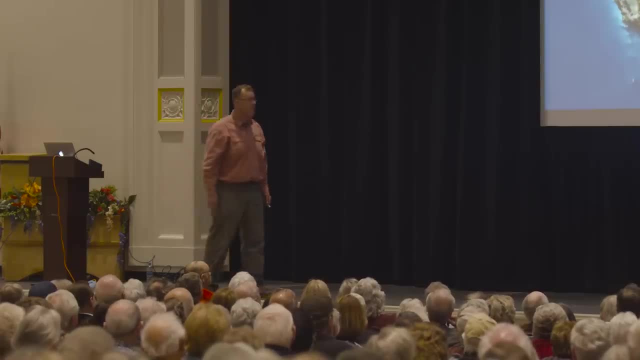 and took geology 101 after that summer in Glacier. I then got a geology degree And it was time to go to grad school And I said, well, I'm gonna go back out there, I'm gonna go study. And I haven't really left the Northwest since then. 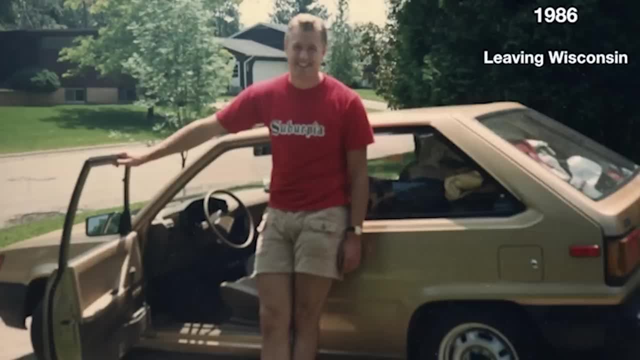 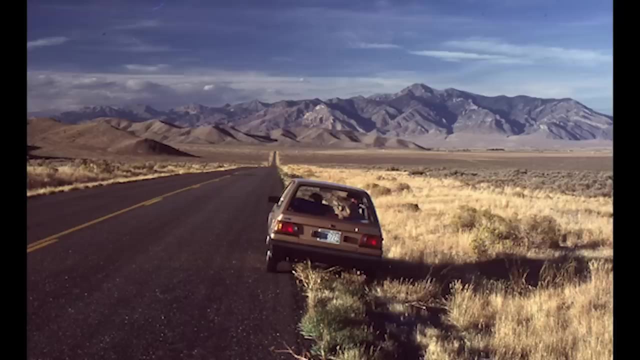 A photo from leaving the tearful goodbye with mom and dad and my brand new car for the first time, A Toyota Tercel with no air and no radio And no floor mats And all of my belongings hitting the road And getting out to Teton Park. 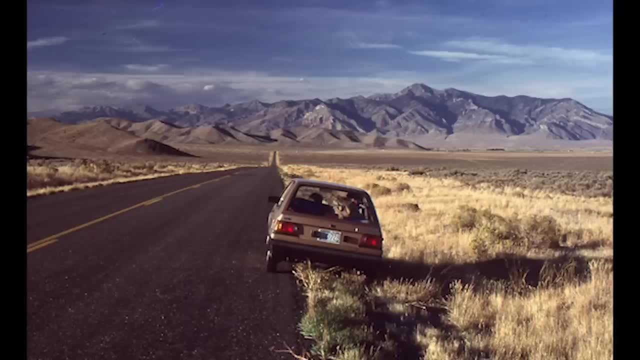 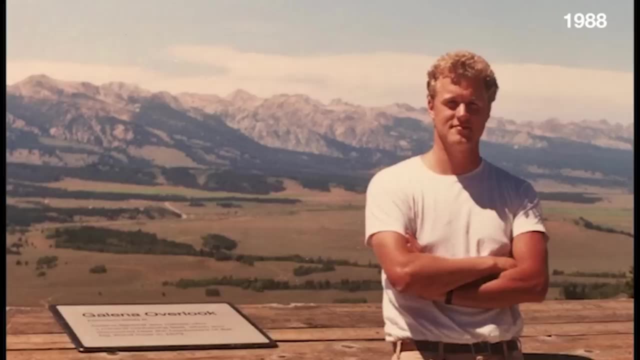 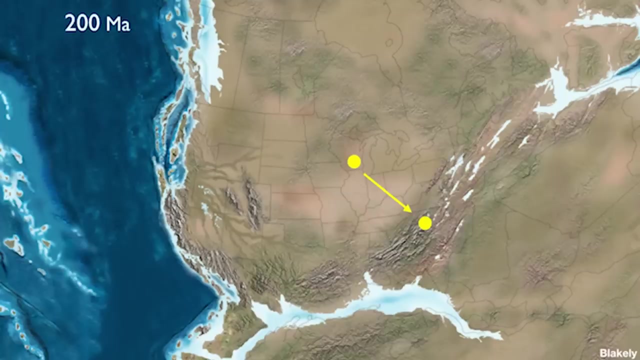 And eventually into the Snake River Plain of Idaho. I went to Idaho State University in Pocatello. It was a great place for me, Learned an amazing amount and started teaching there as well. Great If I had gone to graduate school 200 million years ago. however, there was no reason for me to leave Wisconsin and go to Idaho. There were no mountains at that time. The mountains were in South Carolina because there was no Atlantic Ocean and Pangea was in place. That was the dominant Himalayan like mountain range. 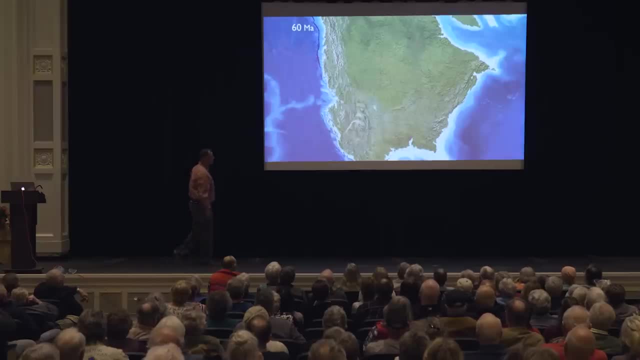 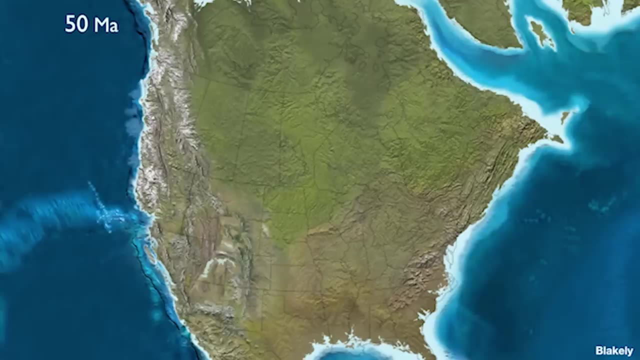 at the time And when we break up Pangea, we take that mountain range, which used to be connected to Africa and Northern Europe, and we split it in half And the Appalachians have been slowly withering away in the last 200 million years. 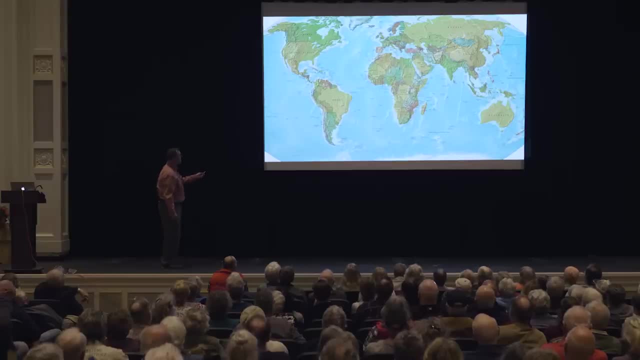 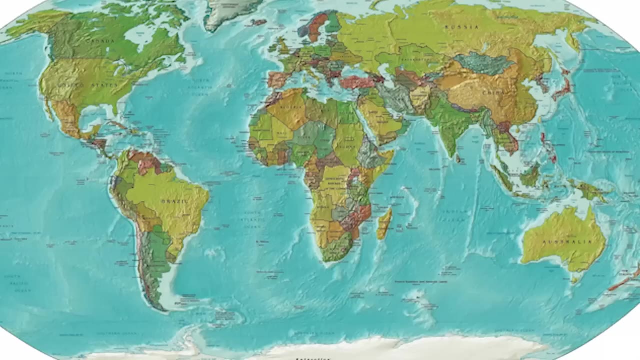 So this familiar world map has half the mountain range from Pangea assembly here and the other half of the mountain range from Pangea assembly there: 300 million year old mountain range, an ocean developing in the last 200 million years. 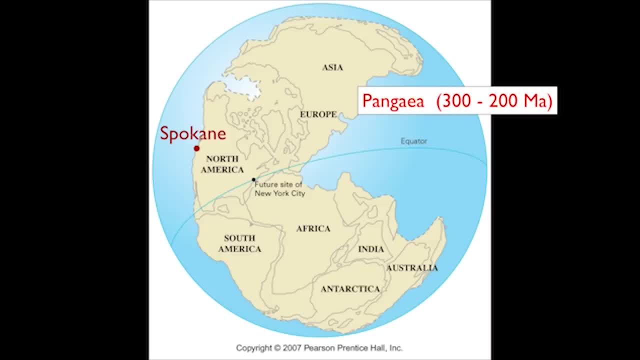 So here's the first of our mind blowing maps, if you haven't seen these before. This is the super continent of Pangea. Notice Spokane on the coast. You're like: where's Australia? I thought that was the big mention tonight. 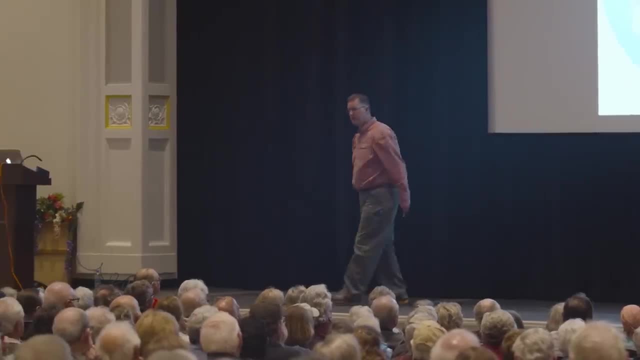 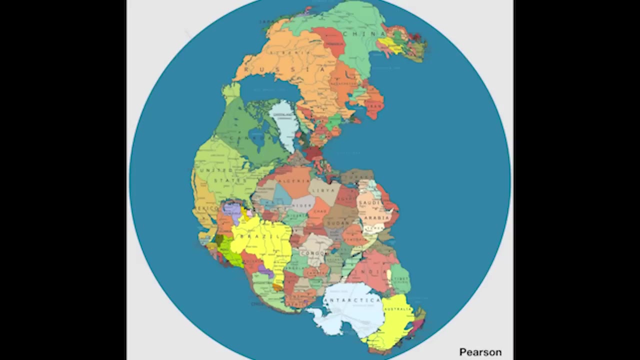 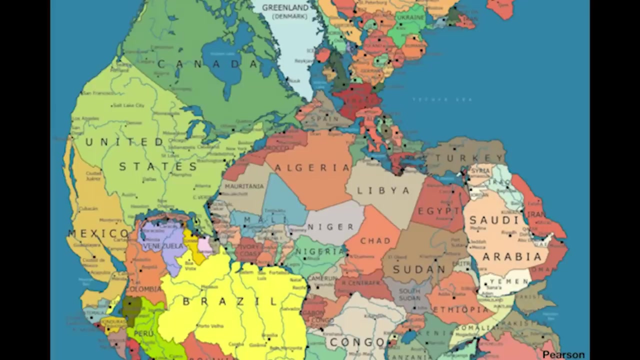 Not gonna be on this one is it? We need a much older super continent to talk about the Australia story. I love this. taking today's countries and placing them on Pangea. Let's zoom in on that So you could go from New York to Morocco. 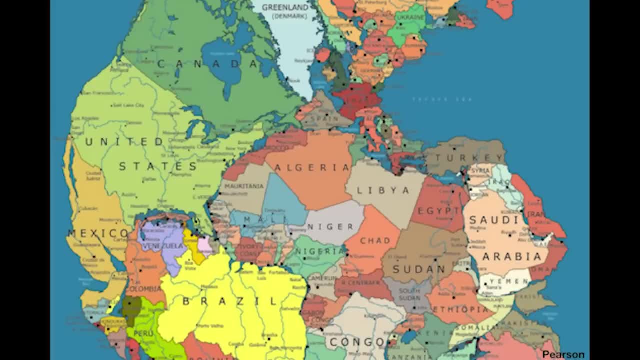 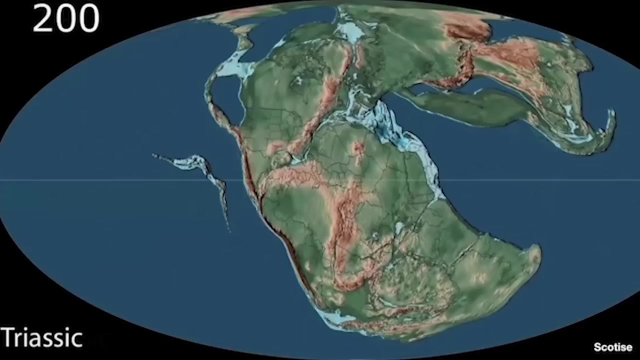 You could go from Charleston, South Carolina, to Mauritania. You could go from the coast of Florida to Senegal. Amazing Pangea, our most recent super continent. Now I'm gonna drive here. Here's North America 200 million years ago. 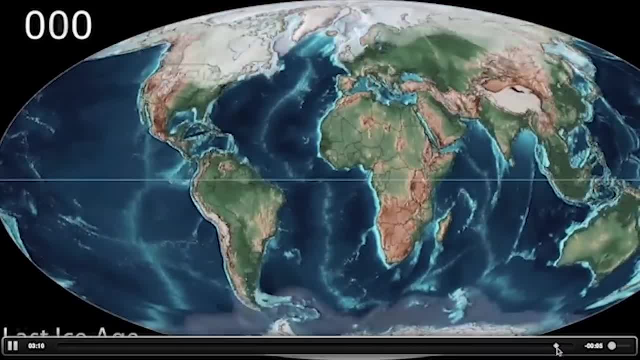 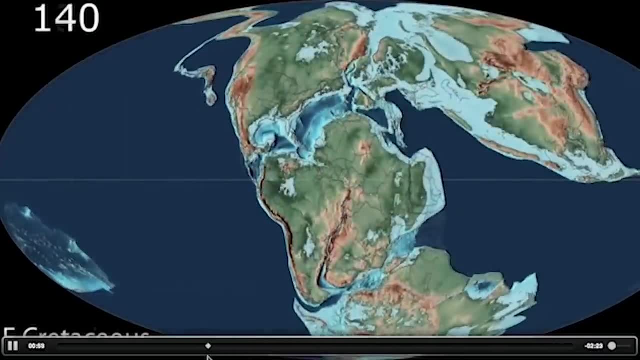 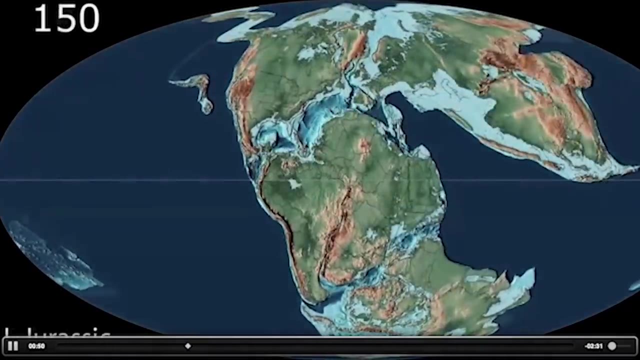 I'm getting us to. that's what's familiar. Now let's go back. Let's close the Atlantic ocean. Oh, you like this? there's murmuring. Okay, this is from Christopher Scotese. There's many of these on YouTube. 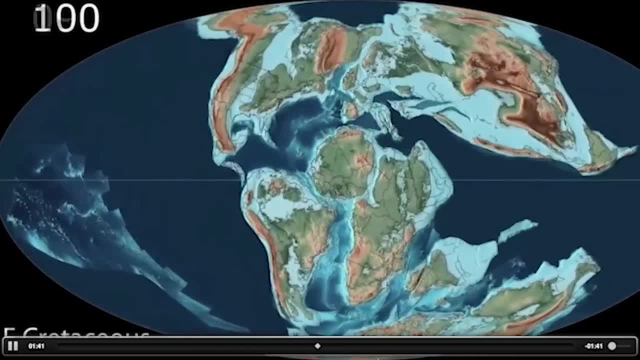 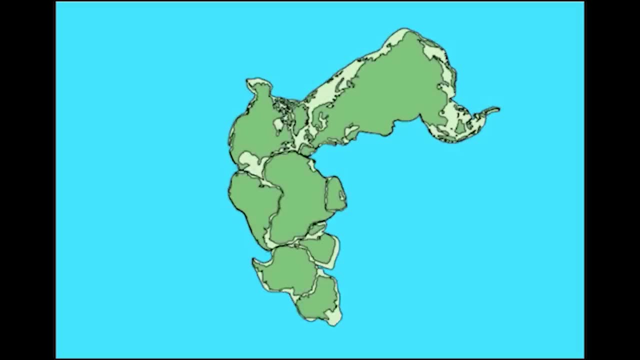 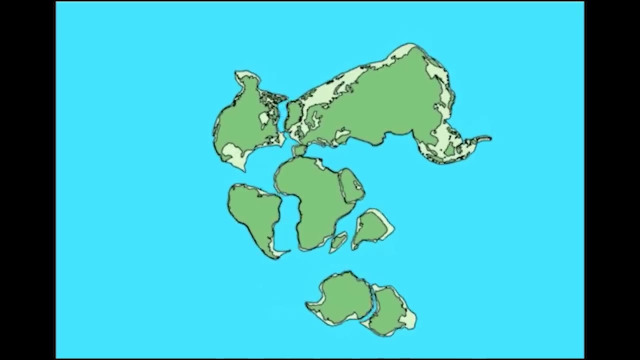 If you look up Christopher Scotese YouTube channel. We're gonna do more of that in a bit. Now this is a more cartoonish version of the same thing I just showed you, And I don't have to control this when it goes pretty quickly. 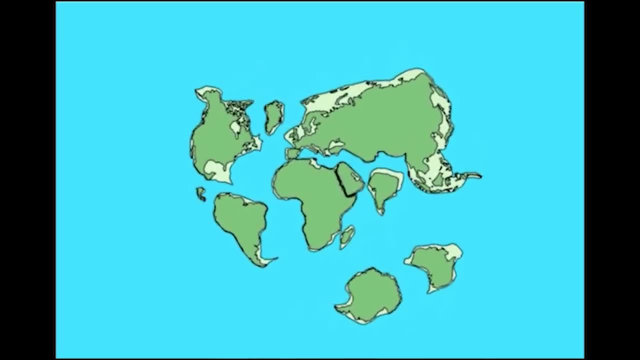 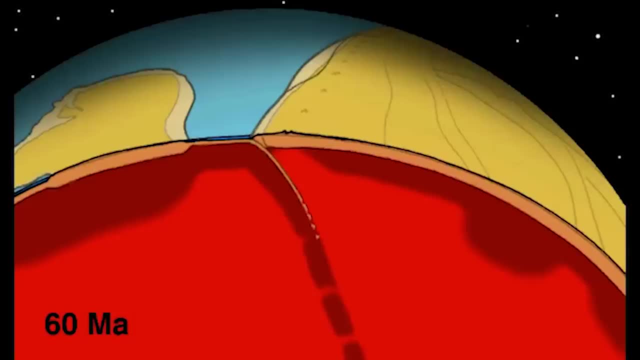 It's the same idea. We're breaking up our most recent super continent, and there's all sorts of things we could talk about, but we don't have time Now. it's important to notice that when we take two continents, we're breaking up our most recent super continent. 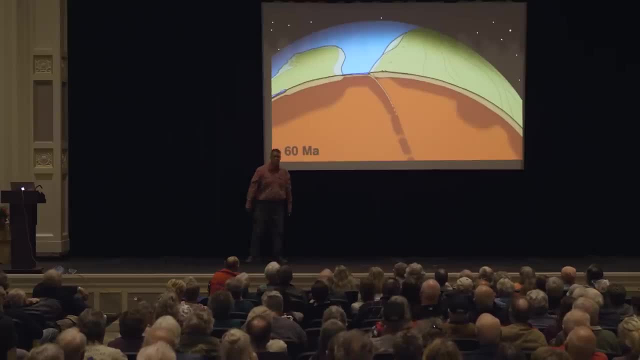 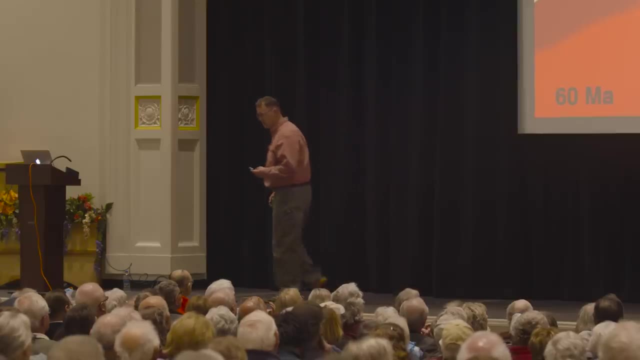 So when we take two continents and start inching them closer and closer together, we've got to get rid of the ocean crust that's between them. We need to subduct or destroy the ocean crust. So when people talk about- quote unquote- continental drift, 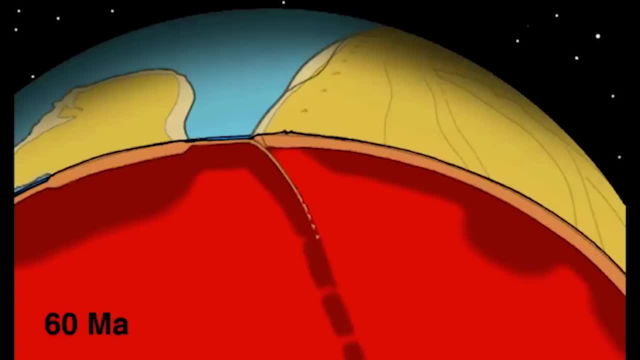 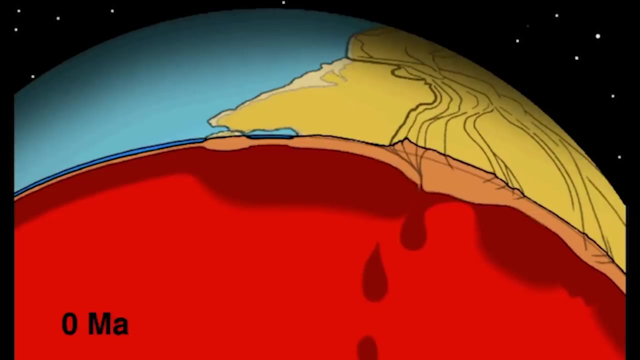 they fail to factor in the fact that the ocean crust is moving along with the continents. It's something we call tectonic plates. So here's India approaching Asia and not stopping once it kisses Asia and eventually forms Asia. So we need to realize that ocean basins need to be destroyed. 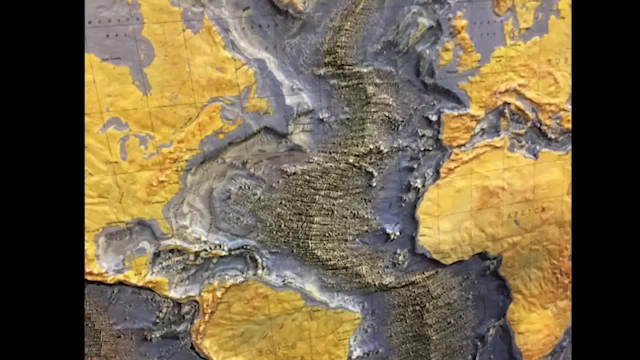 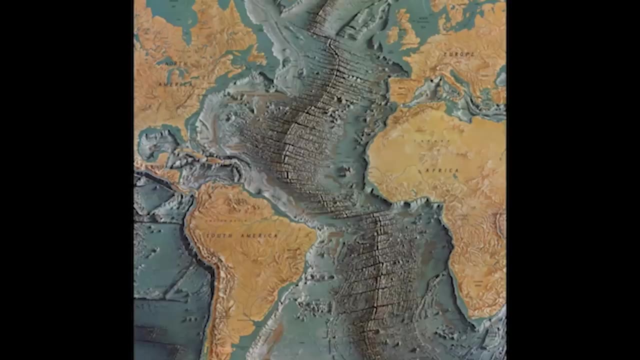 as we do that. So here between US and Africa, is this wonderful mountain range, the biggest mountain range on the planet, called the Mid-Atlantic Ridge. made out of basalt that has formed somehow in the last 200 million years, Mid-Atlantic Ridge. it has a beautiful pattern. 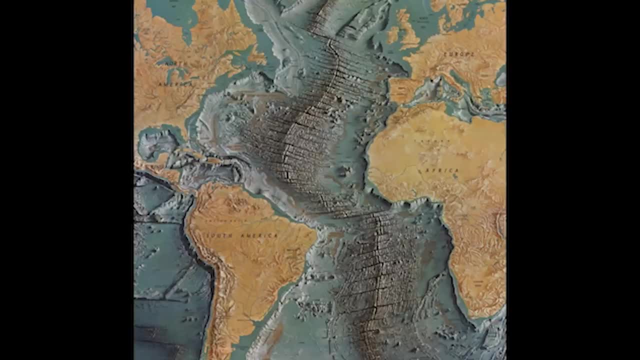 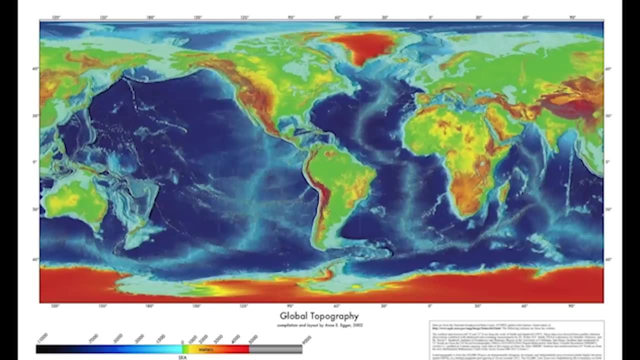 just like the coastlines of the Americas and Europe and Africa. We didn't know about the Mid-Atlantic Ridge until after World War II, But we now know that. that is the reason that we- let me say it differently- we now have good evidence on the ocean floor. 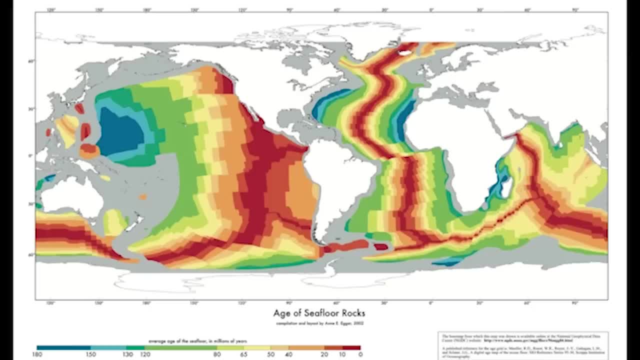 that this sea floor spreading and sea floor creation is a real thing. Have you seen this map before? These colors are the ages of the ocean floor. Red is really young and as we get to oranges and greens and blues, we go back 200 million years. So this was a huge surprise. Why do you have these age? 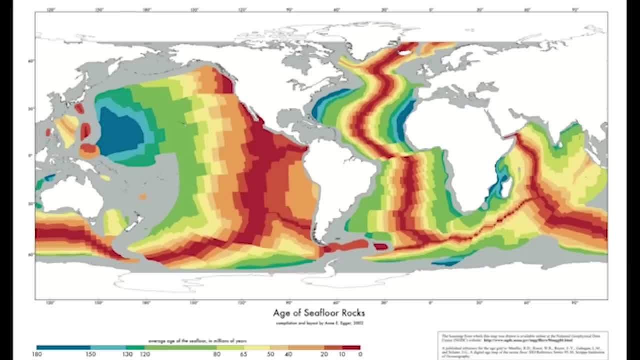 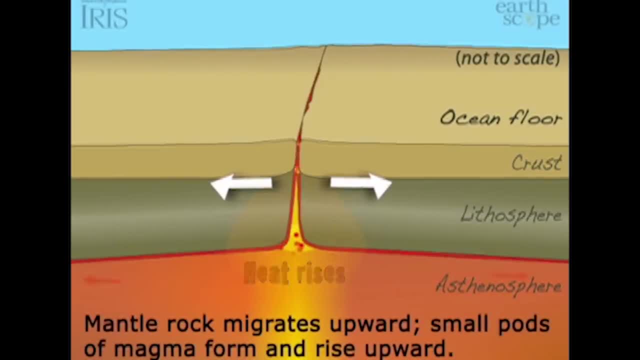 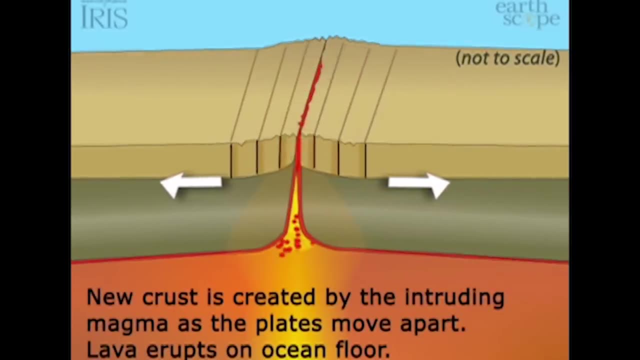 patterns that are perfect mirror images of each other in both the Atlantic and the Pacific. That led to this model, which we now fully accept. today, In the middle of the oceans, we create crust and we make a new batch of crust, crack it in half, send half with North America and half 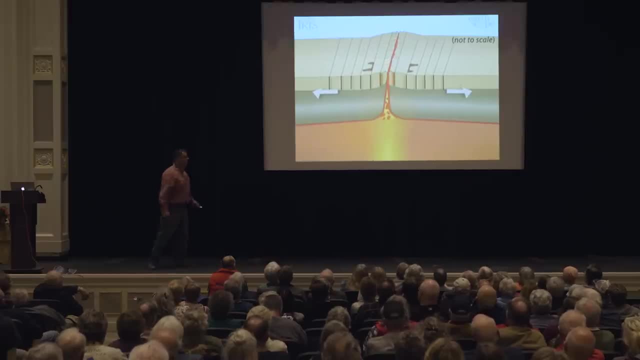 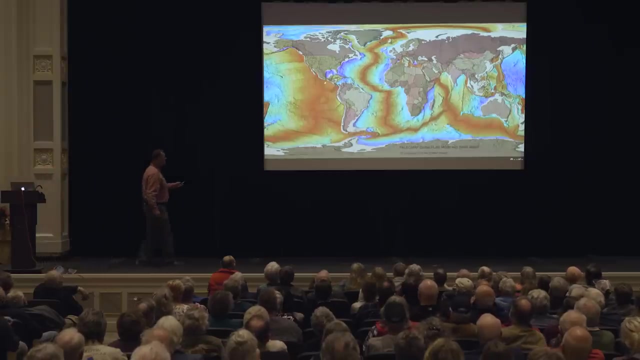 with the African plate and continue, And the continents are drifting away from each other as we create all this crust in between. It's an amazing collection of data from the oceans that tie with the continents. So the East Pacific rise- a seafloor spreading in the Pacific, is actually 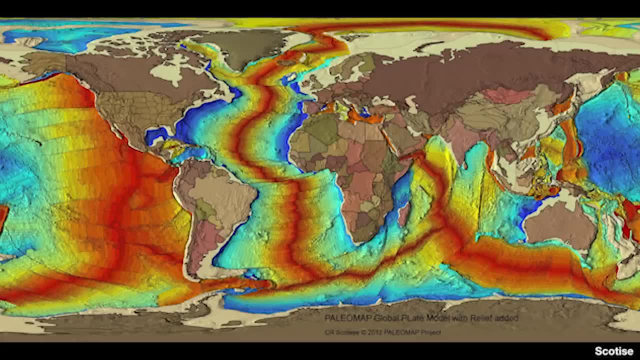 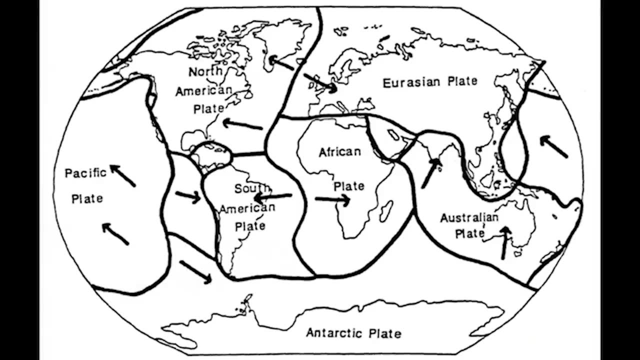 spreading faster than the Mid-Atlantic Ridge, But both are active and both are part of the drifting continent story. Plate tectonics, fully embraced by science. Continental drift, partially embraced because during Alfred Wegener's time he was trying to convince people that continents were somehow. 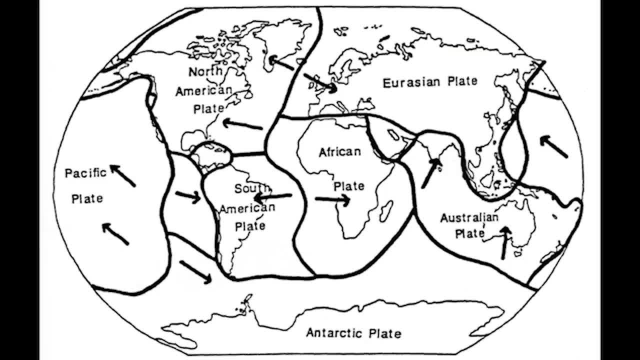 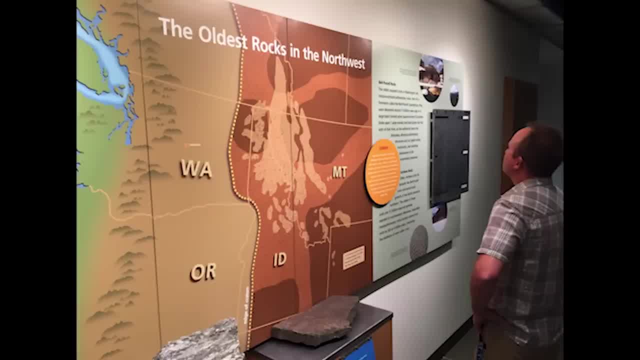 moving through old, dead ocean crust And we now know better The map that we know well. But now let's go to a map we don't know well. This is outside the copy maker in our building. I look at this every day when I come out of the Xerox room and I'm like 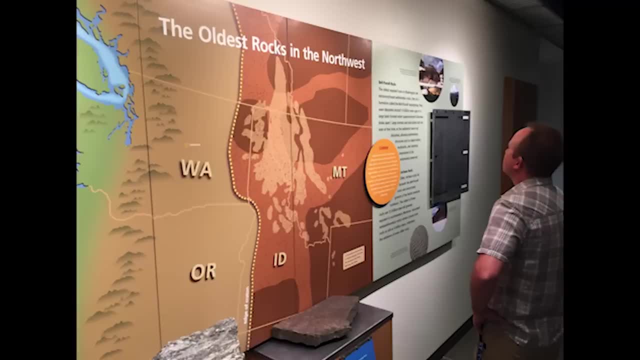 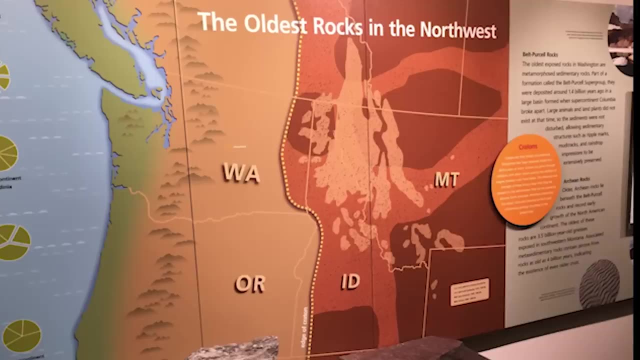 God do a lecture on that. That's such a great display that Walter Zaliga created for us in our new building a couple years ago. What does it show? It shows the old coastline, Do you remember? Here's Montana, Idaho, Washington. There's John Stockton's house in Spokane. 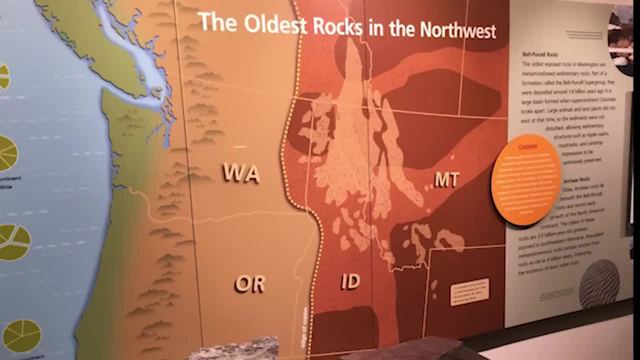 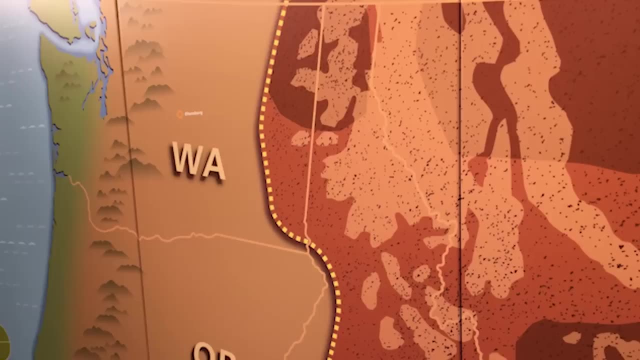 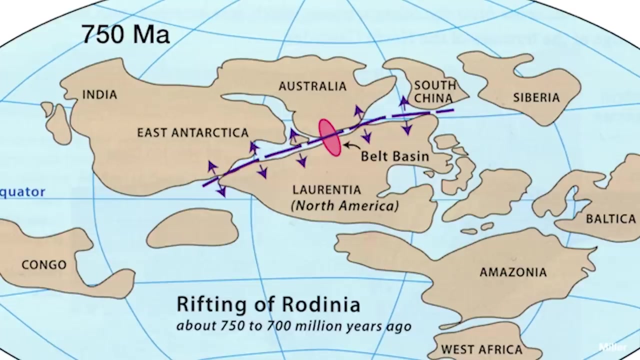 There's the old coastline where Australia broke away at the end of supercontinent Rodinia. There's that coastline Today. Now we're only going to look at a few of these because they're mind blowers, but I'm going to slow down and try to give you a chance to focus on this. 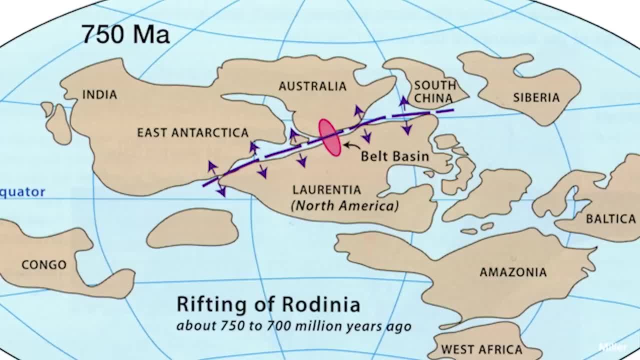 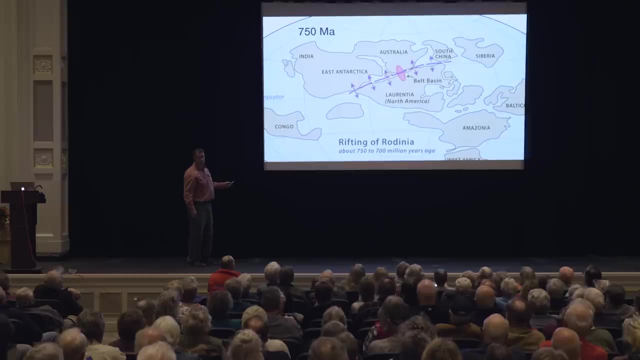 This is the best arrangement that we currently have for the old geography of Roedinia, not Pangea, The Supercontinent Before. Where are we? There's Old North America. There's the Belt of Montanah and North America, Next to the Bazooka Clocking out in view. certainly, But the Okay. 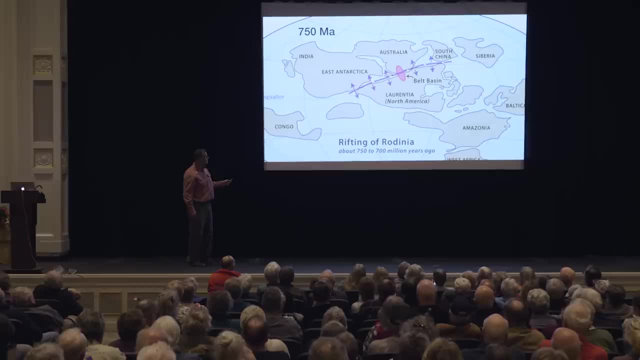 Now, what are you talking about? In fact, there could be some calendars in January. You'll see that, the outside era, we don't have any special â mach RIGHT, We're doing CCG, we bring the A element to the northeastern Washington, and here's the belt, continuing on Africa And remember, 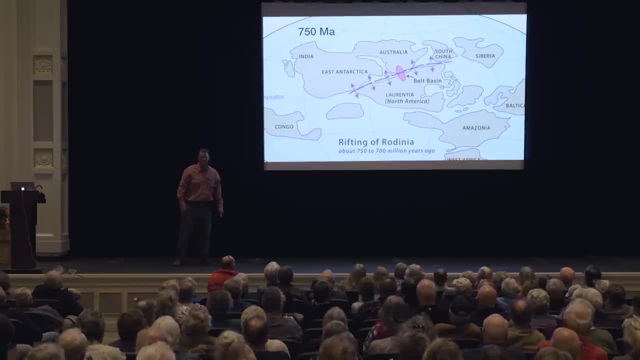 we said 750 million years ago is when we started getting Australia to rift away from us. So I presented it in a nice east-west sense, right, But we've got to throw in some other factors here, So you'll see slightly different versions. 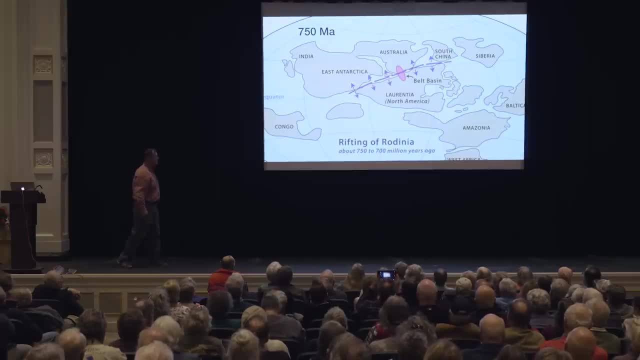 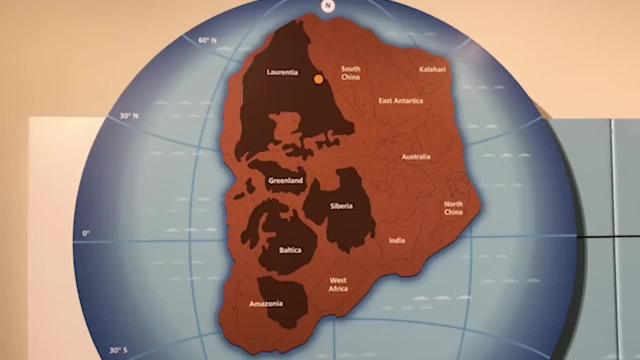 of this map for Rodinia. but this is a fair assessment. This is supercontinent Colombia, the one older, yet the one at the bottom of the chalkboard, And you're like, oh God, what are we looking at? Well, we're looking at a supercontinent, Fine. 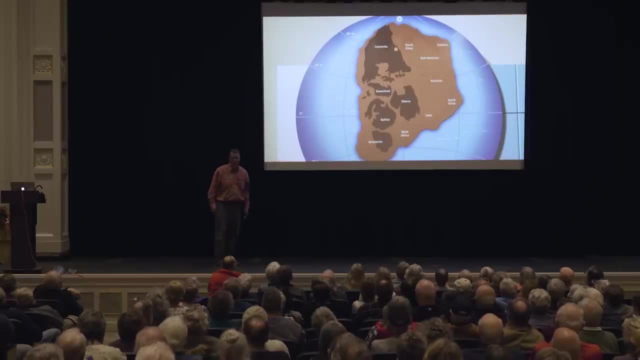 Again. Laurentia is the name we have for old North America. Can I help you? That dot is the belt And you're like wait a minute? that dot's the belt. North America is standing on its head, Mexico is up here, Canada is down here. 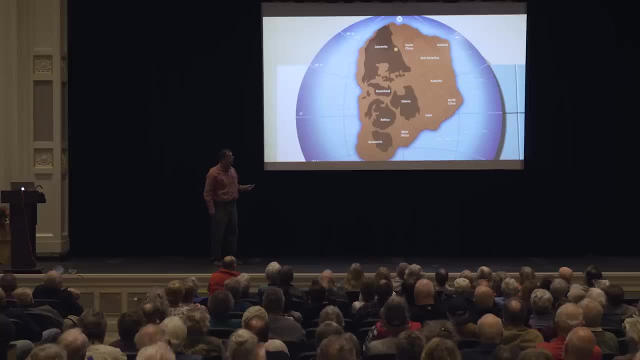 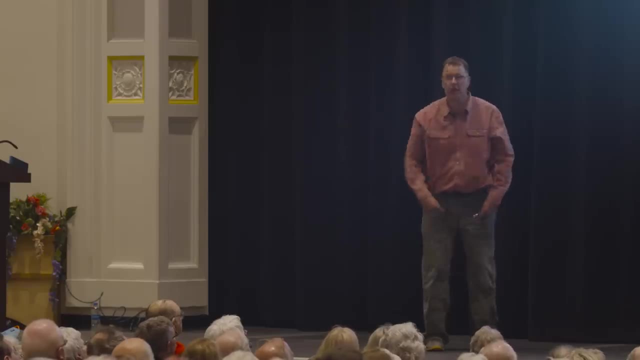 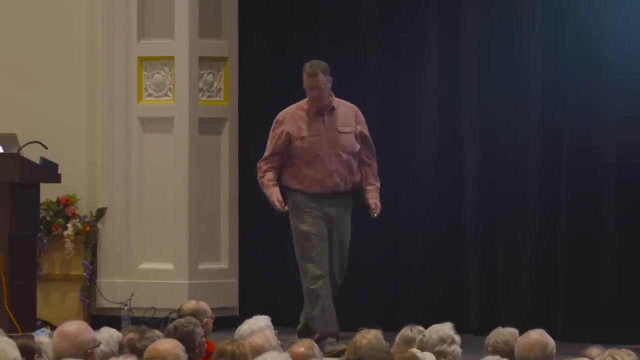 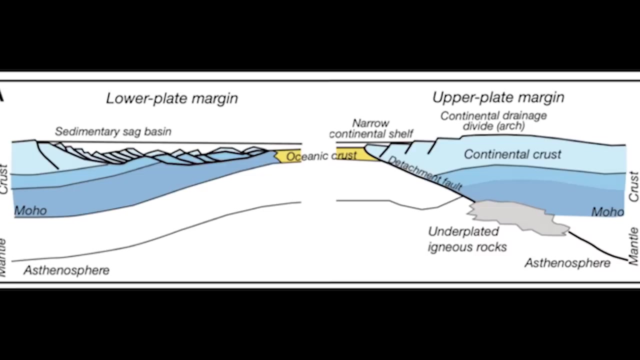 Can I help you all? Yeah, well, see you guys. And this reconstruction of supercontinent Colombia has South China as opposed to Australia. I knew this would happen. The energy has changed. The hands are like: I give up. I get it, I don't know what. I don't, I lost it. I lost it I. 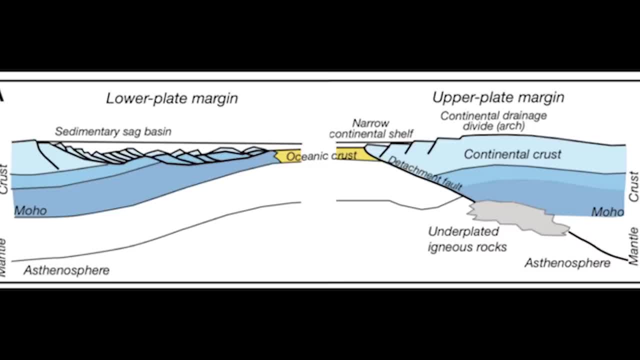 lost it. I knew that was going to happen, so we're not gonna dwell on it. but this is easier to picture. I'm not underselling you now. It's just too much. It's just too much. It's too much too much. But this is this a good. 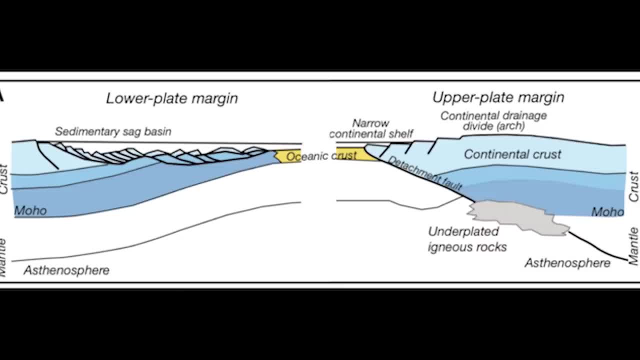 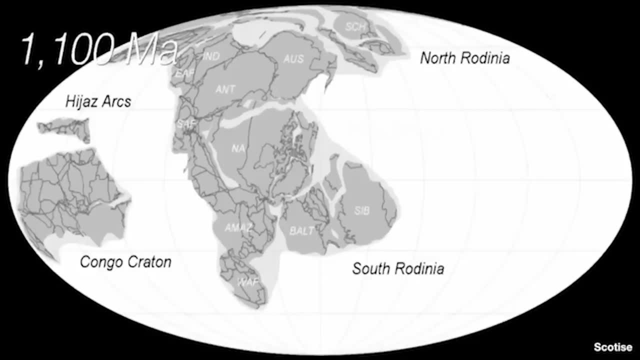 of 750 million years ago, when Australia drifts away from Montana, Idaho, etc. We're going to try this again Now. this guy Scotese, Christopher Scotese, is world famous in geology circles. He's even got an animation going back. Look, we're back to earlier supercontinent days. 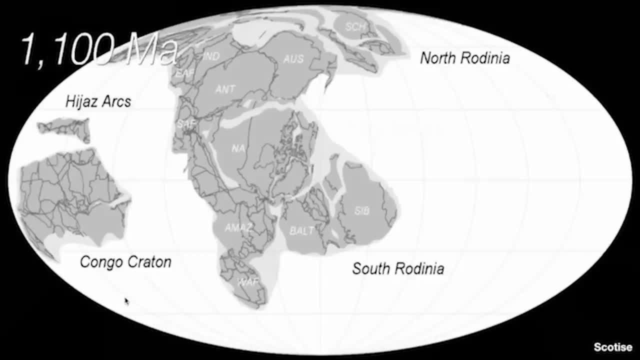 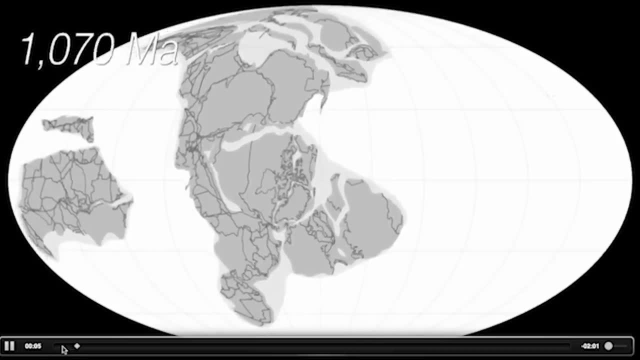 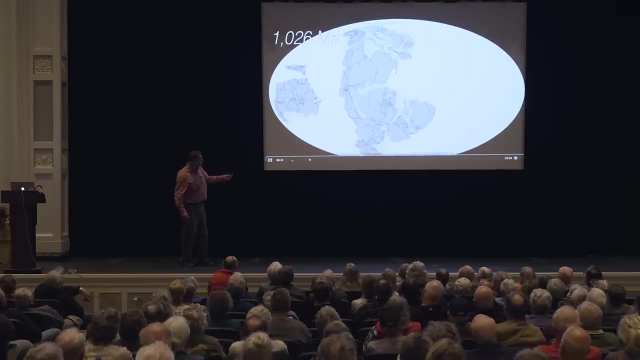 and there's lots of error here, but there's enough to think that we can do something with it. I'm going to try this, I think I only want you to notice one thing: Here is North America, Canada, US, Mexico, and here's our rift. Here's when Australia is going to rift away at 750 million. 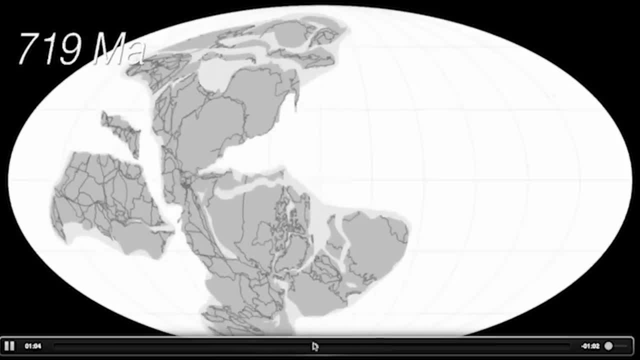 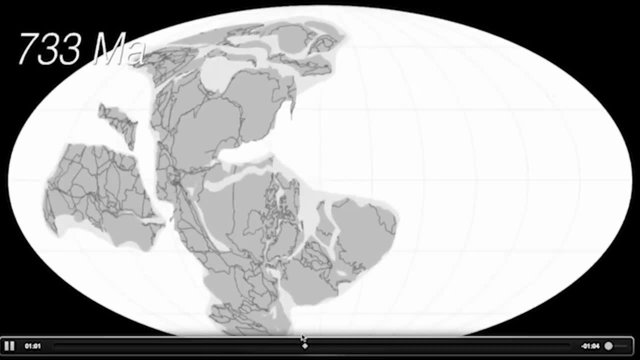 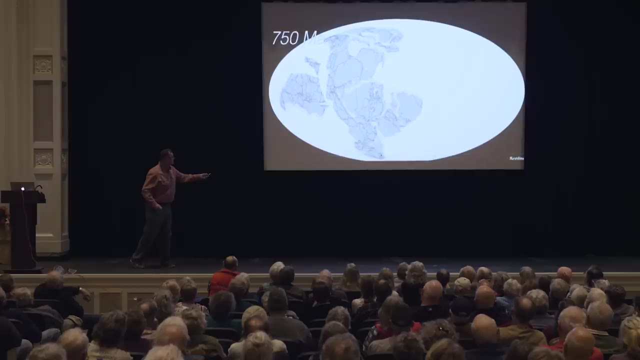 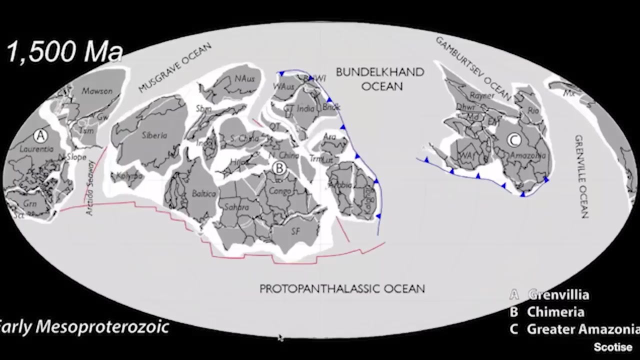 years ago You ready And okay. Now, if you're a great map reader, Scotese has Antarctica instead of Australia next to us. This is Australia, That's Antarctica. This is Montana, That's Canada. So you can see, there's variations just from animation to animation. He's got another one. 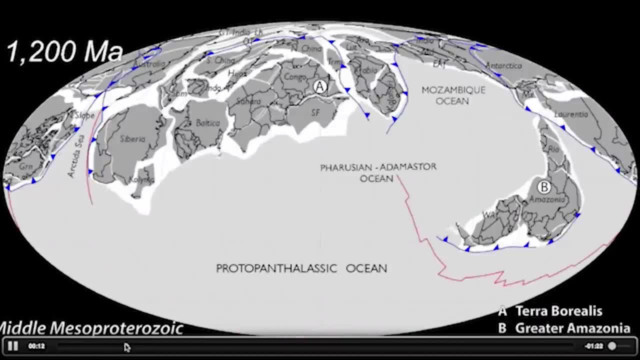 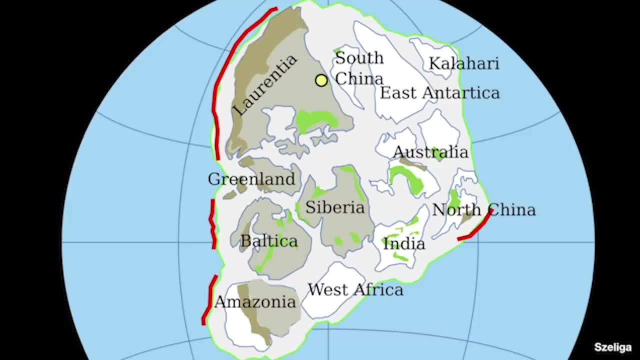 Is it worth it? I don't know Enough to just blow us over. Okay, great, So I don't want to show many more of these. but our assumption that North America always is nice and tidy and Canada's north and Mexico's down, even that is a spinning orb, and the evidence exists for all of that, as 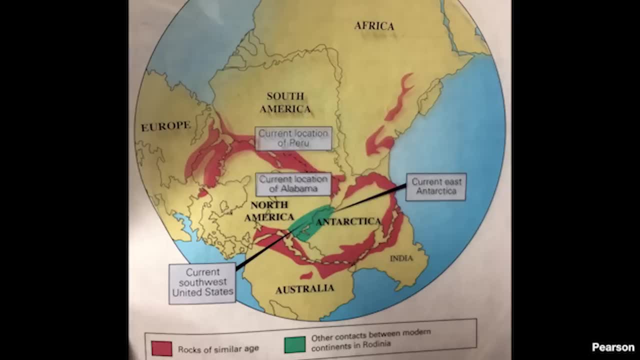 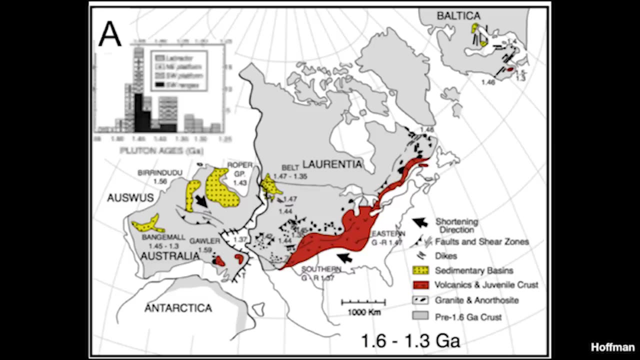 well, which I don't understand very well. That's enough of these. That's enough of these. That's enough of these. Oh, this guy, Hoffman, this gives you an idea of how you can try to make a case for a certain continent. Hoffman's an Australia guy and he says: here's the belt in yellow, There's. 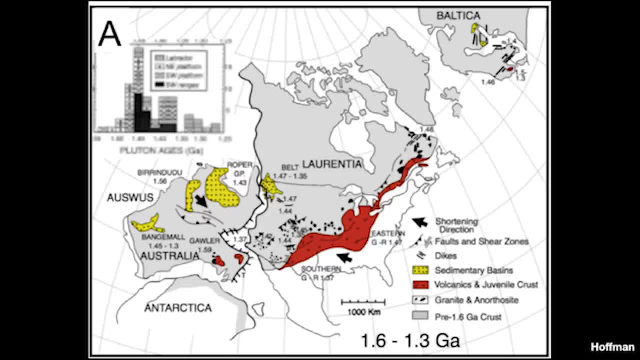 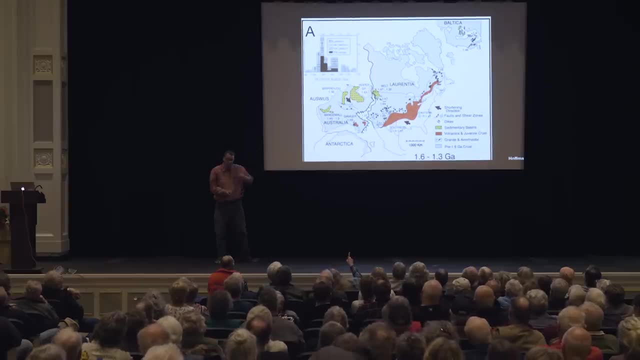 a belt-like basin in central Australia, Another belt In central Australia, Here's Antarctica. down here He's even taking some of the another part of old North America and finding its scraps of Australia. So it's a game of positioning old continents and 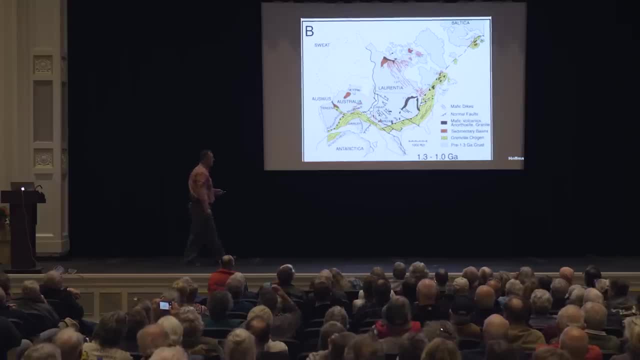 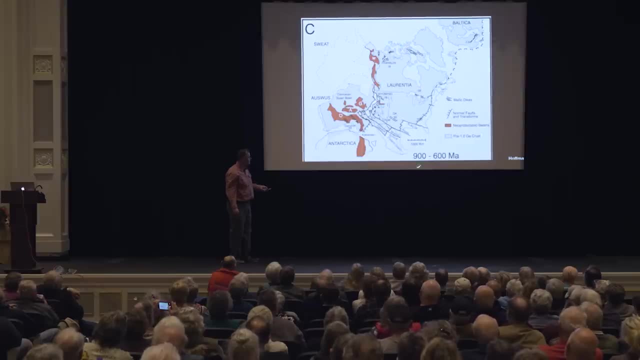 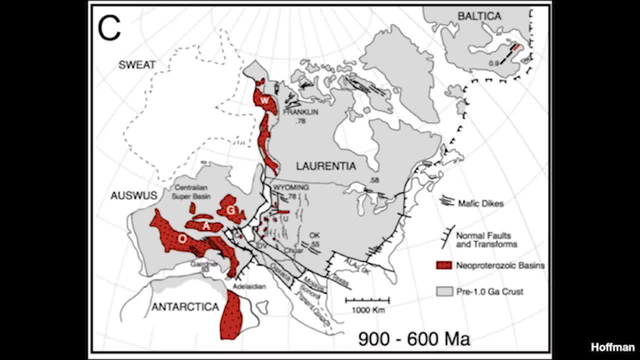 million years ago, and some basalts, Some neoproterozoic basins- I guess they're basins. sorry, But we've got the same idea. So it's not just the shapes of the continents is my point. 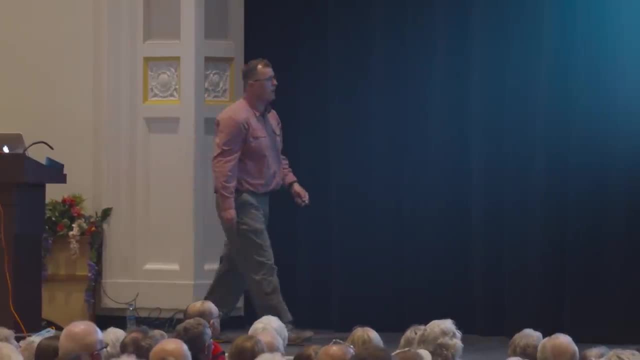 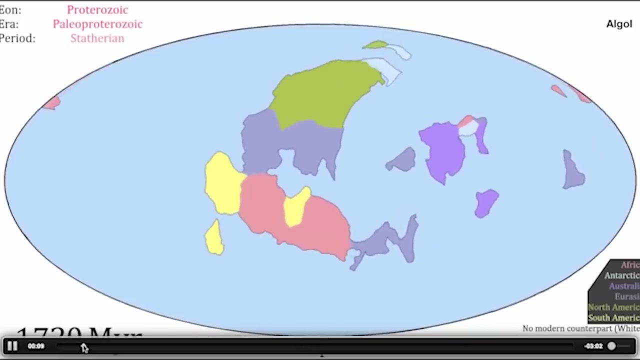 It's using some pre-Cambrian geology in there as well. Oh my God, We've got this one too. You want to really get depressed. This is the last 2 billion years of time, And I'll point out: this is us. 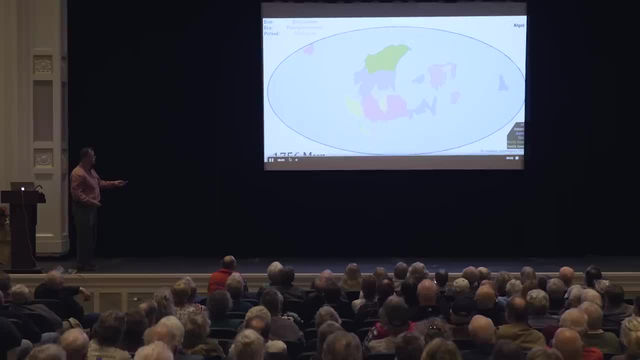 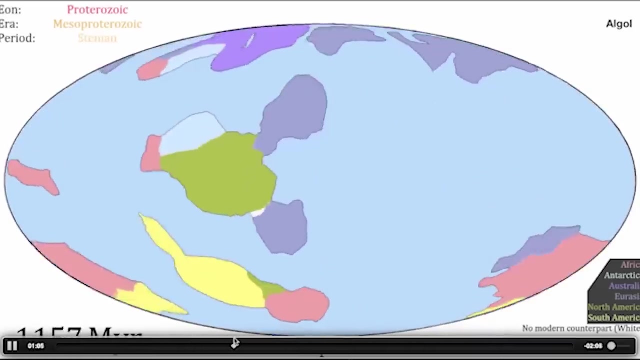 that's North America and presumably that's the Montana coast right there. So I think these will change over the next 20 years as we get more and more data, but I'm gonna stick with this until we get something that looks familiar. We're. 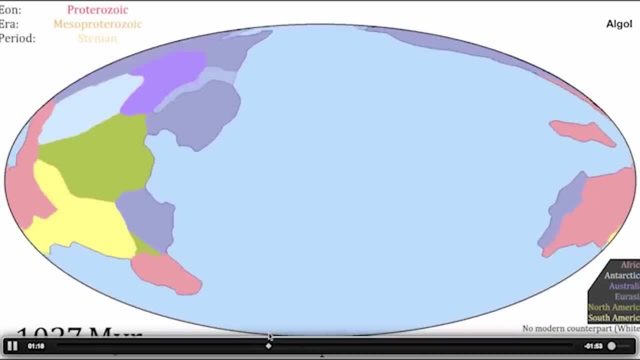 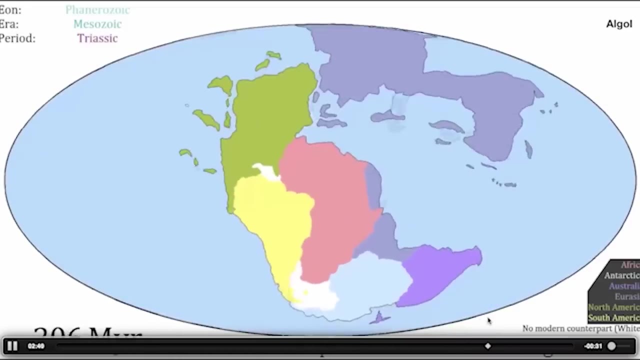 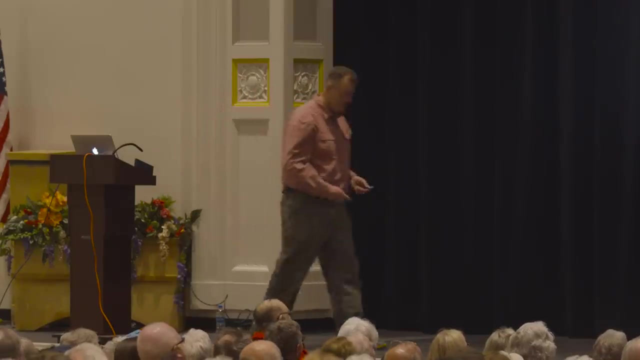 not even to a billion years ago. yet There's a billion and you're like, please, something I can record, please, please, where do I fit in? Oh, oh, oh, oh, oh, oh, oh, hey, all right, oh yeah, okay, great, Yeah, they did a nice job. 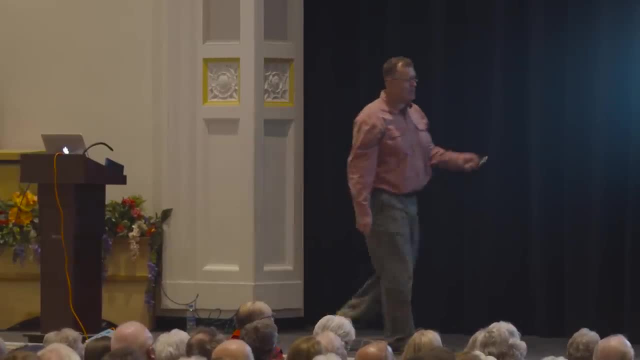 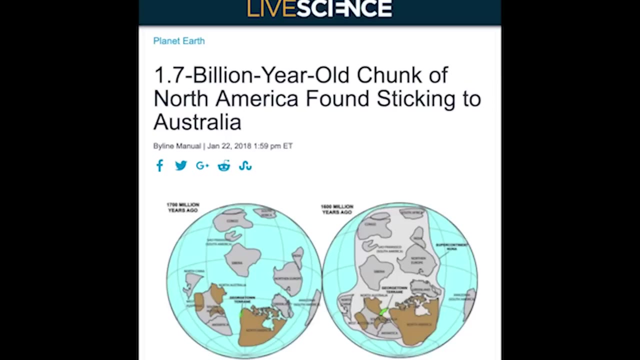 Should have ended the lecture right there. Okay, a couple more. So you've got headlines like these and I never really understood how to make sense of the headlines because I didn't have that timeline that we had on the black chalkboard. I needed that personally to know where to plug some of these. 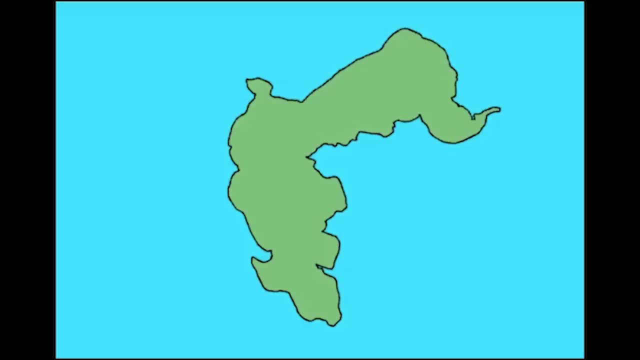 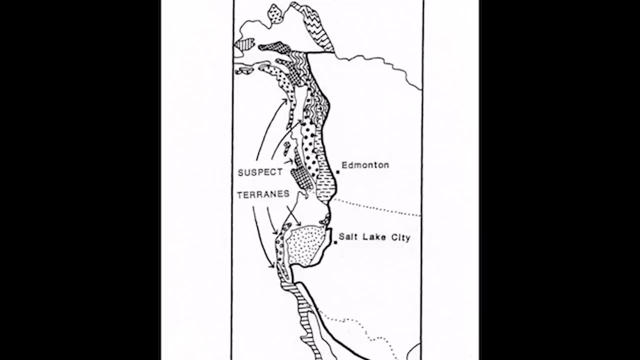 headlines in. I know I'm a little closer to that, and maybe you are too. We've already seen that. So in the last we're gonna finish where we started: talking about Pangea, breaking apart Pangea and making the 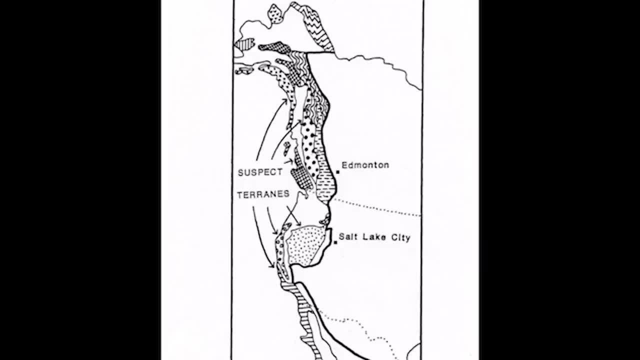 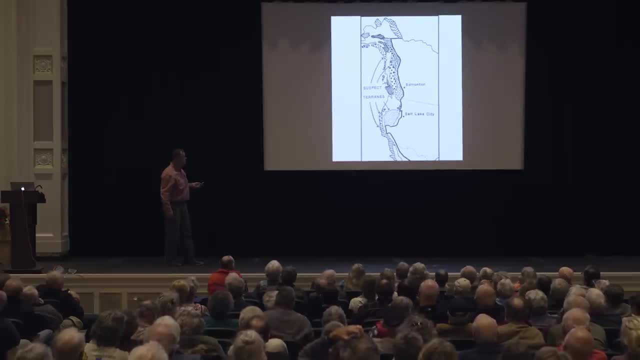 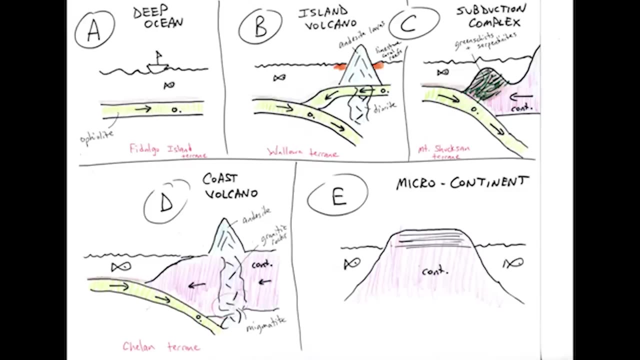 rock of the world. So I'm gonna start with the rock of Washington with a couple new ideas before we quit. Here's Spokane, here's all the crust that has been added to the west coast of Old North America since the breakup of Pangea. Those exotic 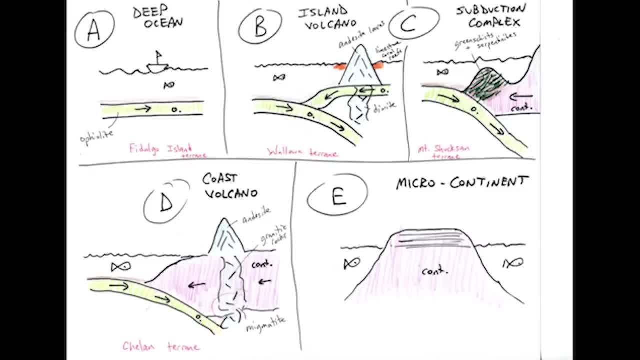 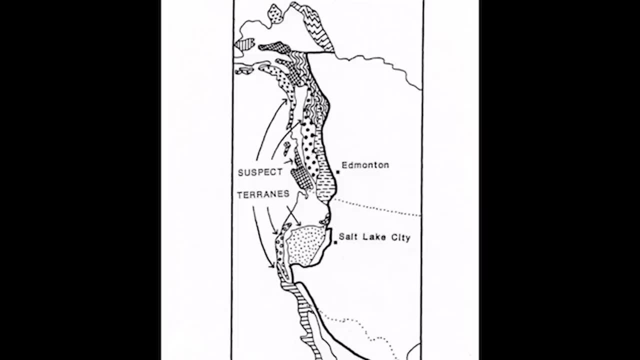 terrains are completely different kinds of rocks with completely different stories of their own. That's a whole other lecture that we tried last winter. That was a tough lecture to put together All these scraps of land, these exotic terrains, have their own story and their own origin. If you remember the lecture, 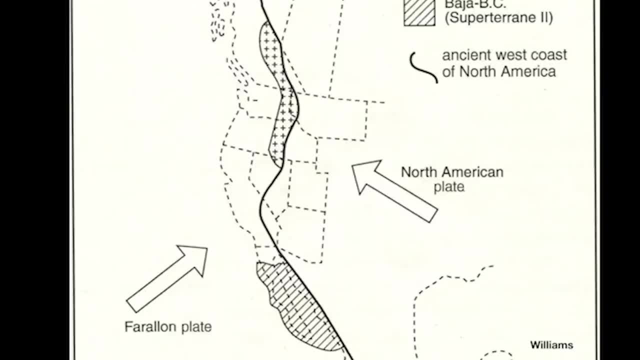 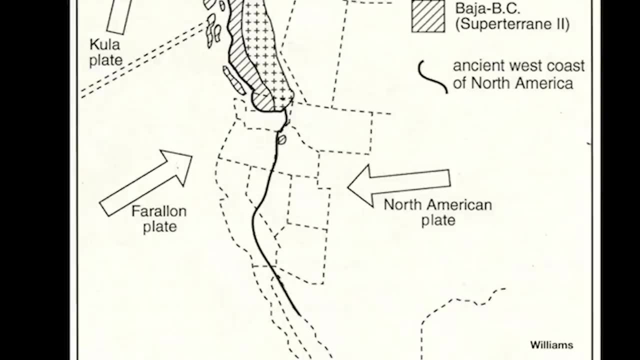 from last year. the main message was: a bunch of those terrains were actually added in Mexico and then got shifted 2,000 miles to the north between 80 and 50 million years ago. Again, this is all crazy stuff happening after Pangea. 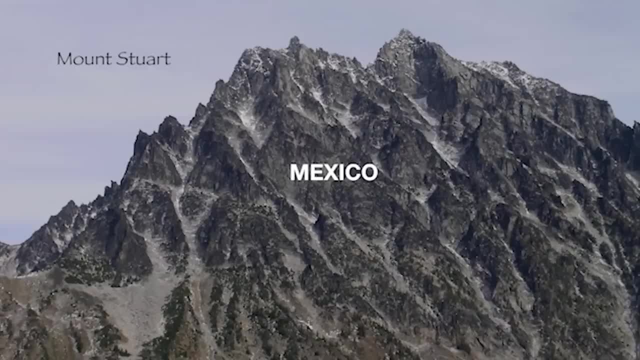 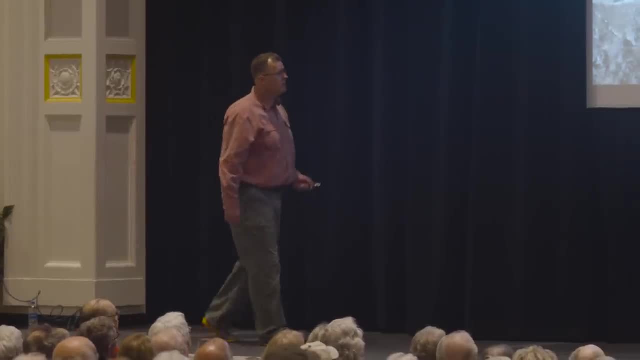 breaks apart. And yes, we made the point that there's growing evidence that our beloved Mount Stewart, north of town, is a rock of the world, And that's what we're going to talk about today. But before we do that, I'd just like to share a couple of evidence points today. 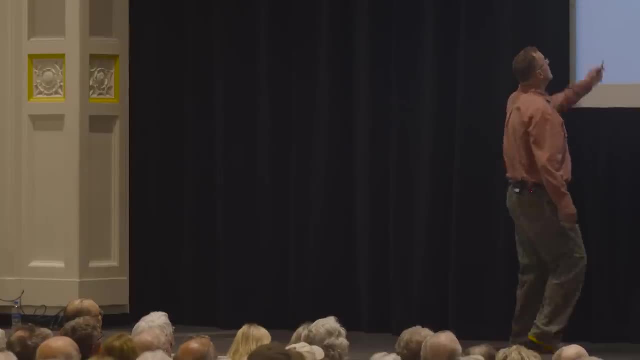 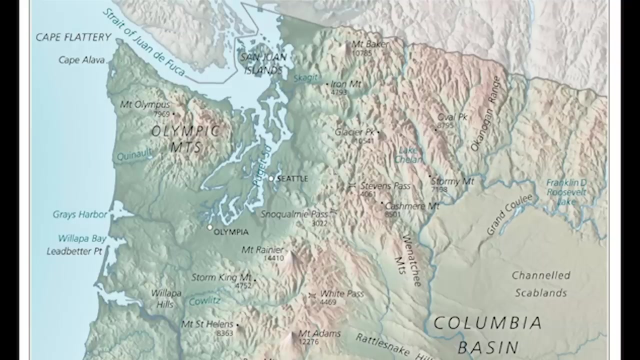 that we've actually found on this map. But first you can see that the July ации town was originally in Mexico. Are you deeply offended by this? So, looking at this map, this is all a very new part of our continent, The youngest and newest. 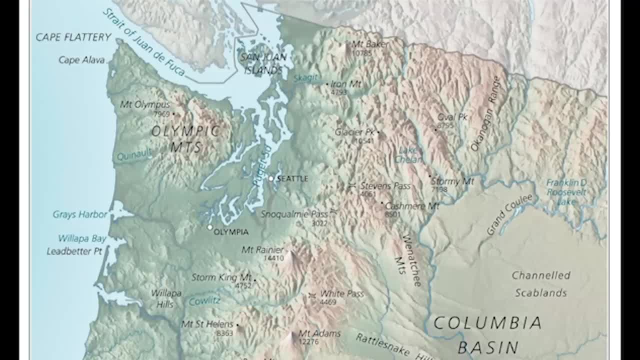 was added, The west coast was at I-5. So that's another way to look at this. We tonight have been looking at all the evidence for the coast of North America over here at Spokane. right, That was most of tonight. But the coast starts jumping west as we keep adding crust to the western edge of North. 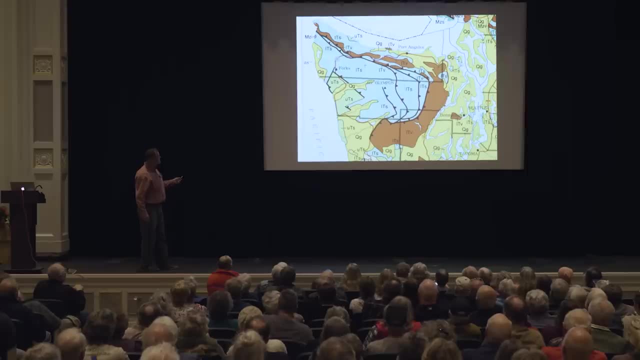 America. All of this basalt that runs from the northern edge of the Olympic Peninsula, makes up the Hurricane Ridge above Port Angeles, swings through here by Hood Canal, the Willapa Hills, down by Olympia. That's all 55 million-year-old basalt that originated offshore A couple years. 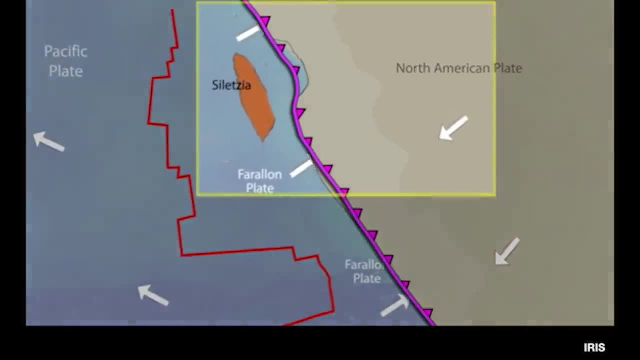 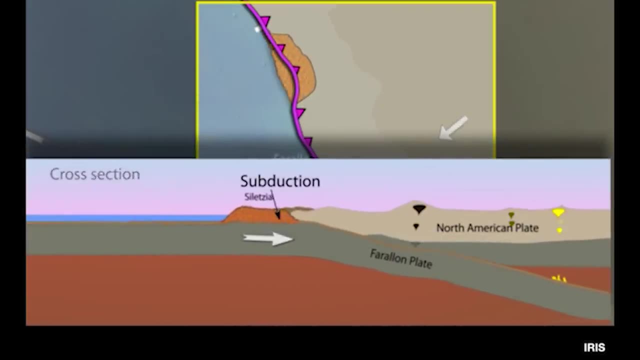 ago we talked about Siletia, a huge chocolate gumdrop out in the ocean, And that's the last of the exotic terrains to add to the west coast here at our latitude. Today we have the last of the exotic terrains to add to the west coast, here at our latitude. 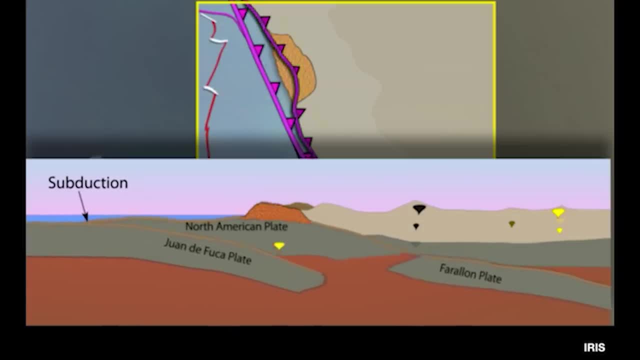 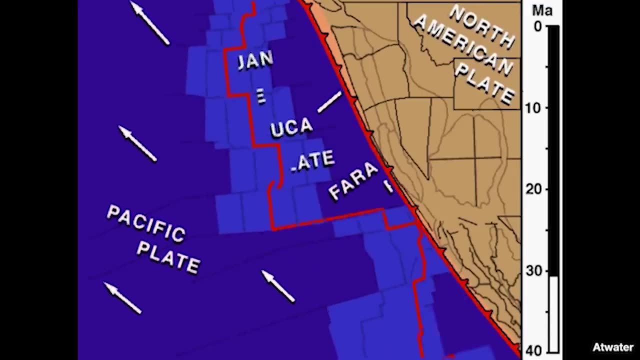 Today we have the last of the exotic terrains to add to the west coast. here at our latitude Today we have the Juan de Fuca plate subducting, which is a remnant of the Farallon. But the point is, the age of a huge ocean plate coming at us is about done And our west coast. 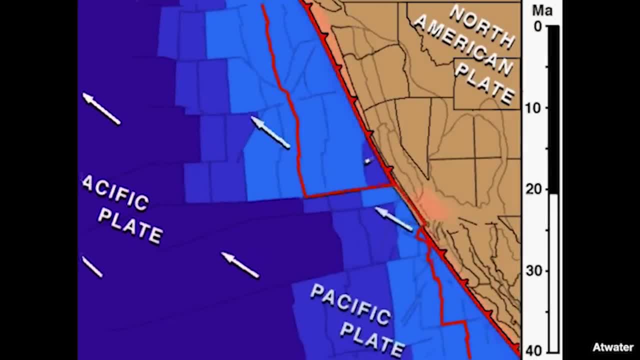 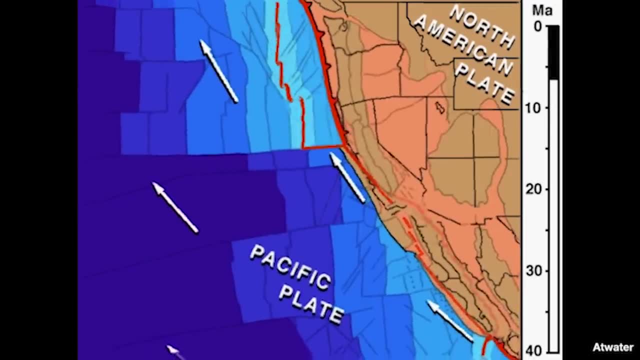 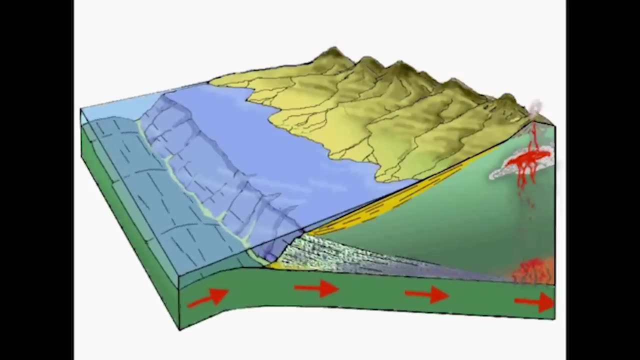 is going through major changes right now, in the last 20 million years. We're realizing it now that much of the geology is changing. I'll give you a couple of examples and then we'll quit. When we did have that big ocean plate coming at us, it subducted and fueled. 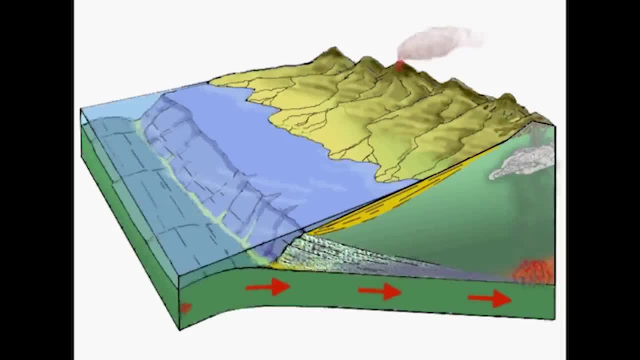 and figured it was about time we left. So we were on the way to the end of our last decade. We still had the Volcanoes, We still had the Cascades. So we still have a little bit of that left. But we better enjoy the Cascades while we've got them, because they're not going to be. 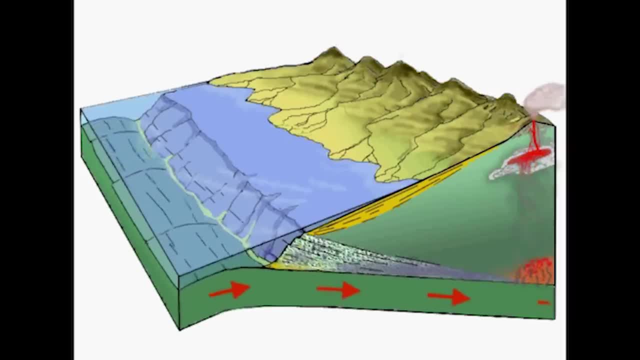 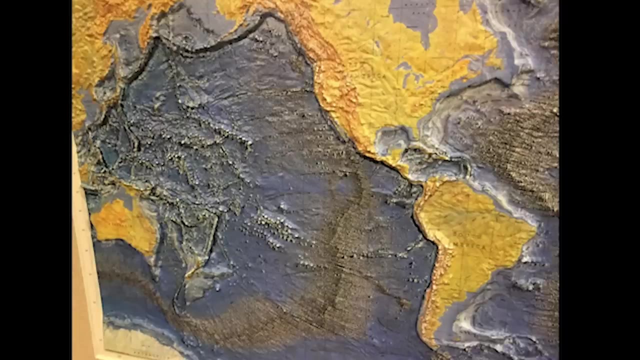 with us for much longer. I'm serious, And that's because this ocean crust coming at us is about to quit. And it's about to quit because we're about to cross, as North Americans, over the East Pacific Rise. You can see the East Pacific Rise today off the coast of South America, But we have come here now. crossed a majority of these Pacific Rise already and only one little piece of these Pacific Rise is still off the coast of the Pacific Northwest. When we finish the job of crossing this little spreading center, like California has crossed the spreading center, our volcanoes will stop. 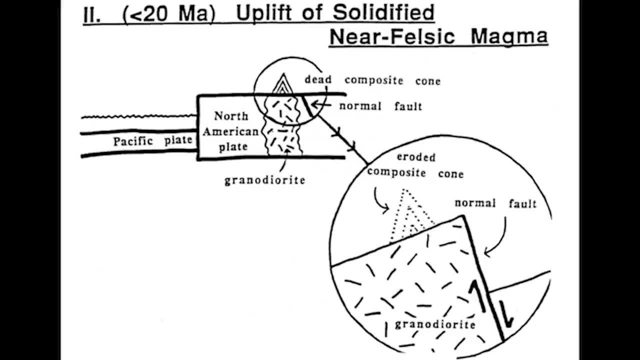 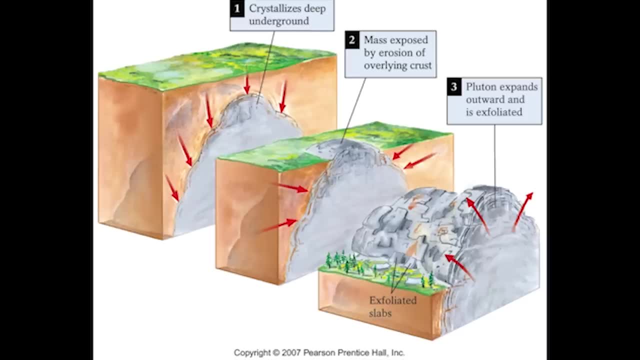 The volcanoes will stop. and the volcanoes will not only stop, like they did in eastern California, they're going to physically go away, and the underground magma chamber rock is now up in the mountains. I'm talking about the Sierra Nevada mountains of California today. There used to be